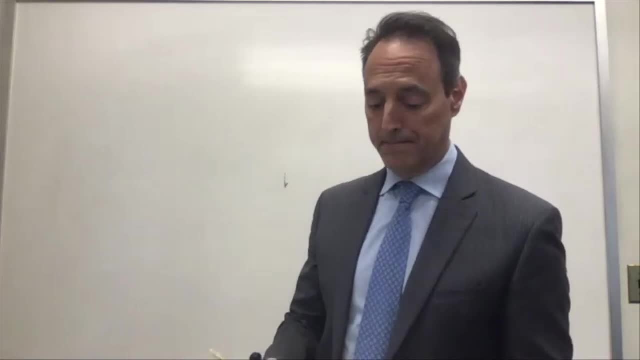 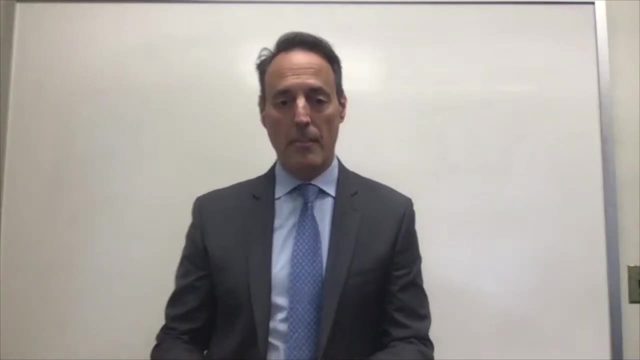 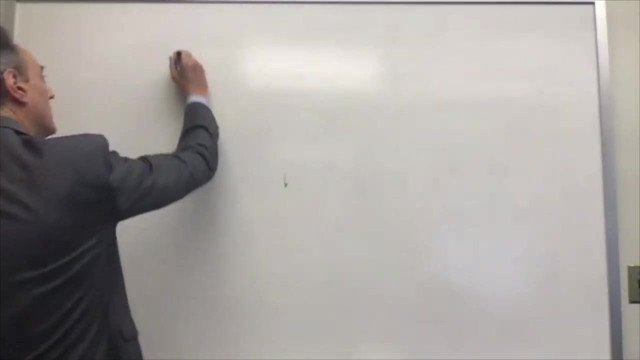 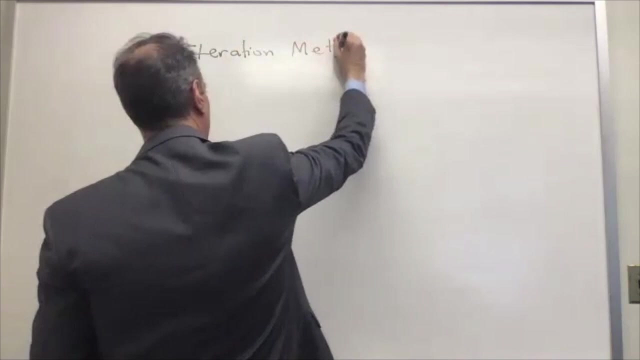 algorithms that allow you a way to solve AX equal to B. Well, Jacobi and Gauss-Seidel are very simple iteration schemes And we're going to talk a little bit more about you know more difficult or more advanced iteration schemes, So this is our topic. 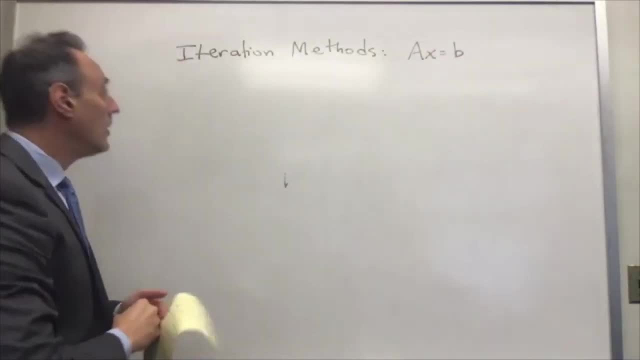 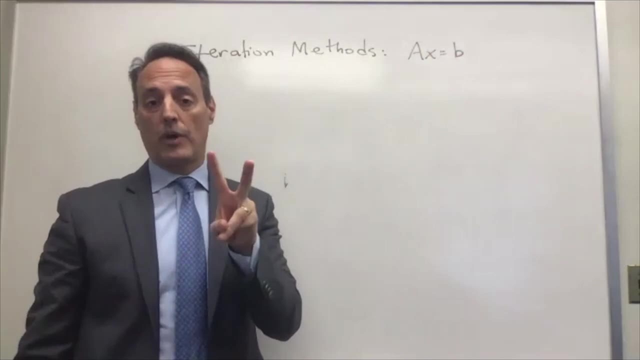 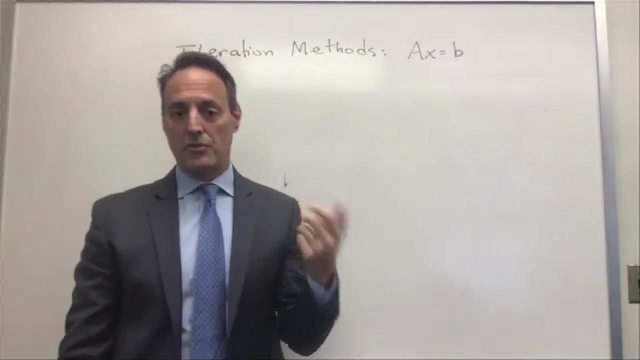 Iteration methods for AX equal to B. Okay, Today, in fact you know I'll get around to- we're going to talk about two methods in particular Today. The first one's going to be called the generalized method of residuals. 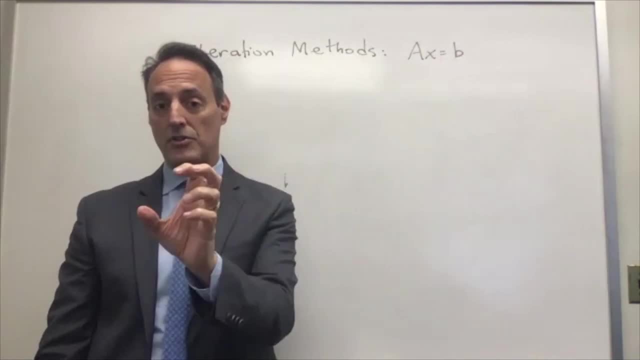 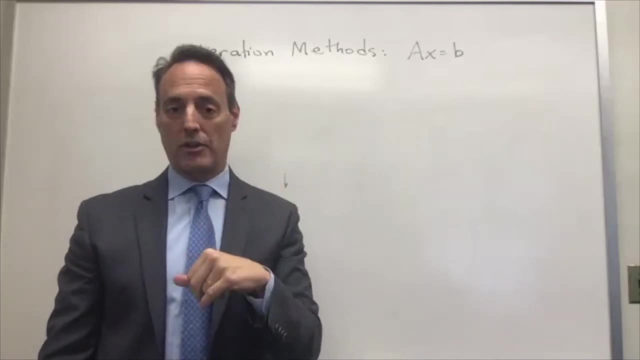 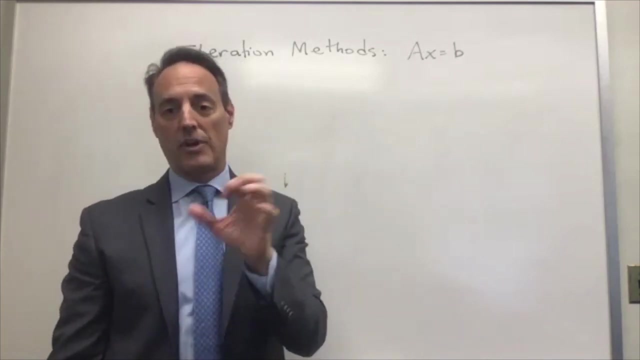 often called GM res, so generalized method of residuals, GM res And the other one's going to be conjugate gradient or bi-conjugate gradient methods, which often is called bcg, stab, or stabilized by conjugate gradient methods. so these are going to. 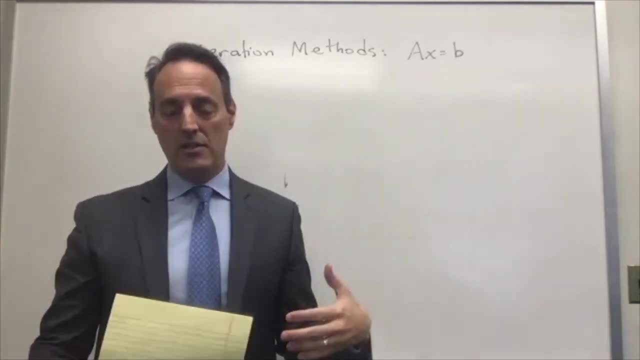 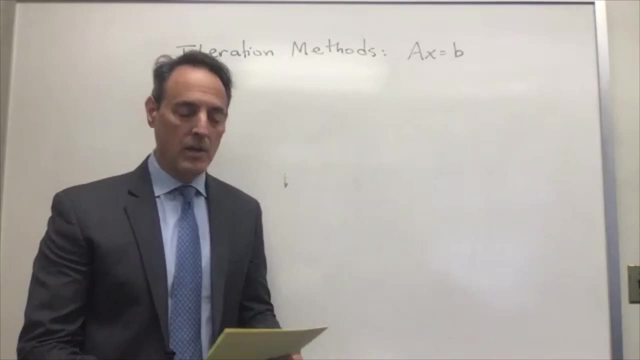 be the two methods we're going to talk a little bit about today- gm, res- and in the next lecture after this one, uh, these conjugate gradient methods by conjugate gradient methods. uh, the first thing i want to do is: why are we going after these iterative techniques? so you could always ask: 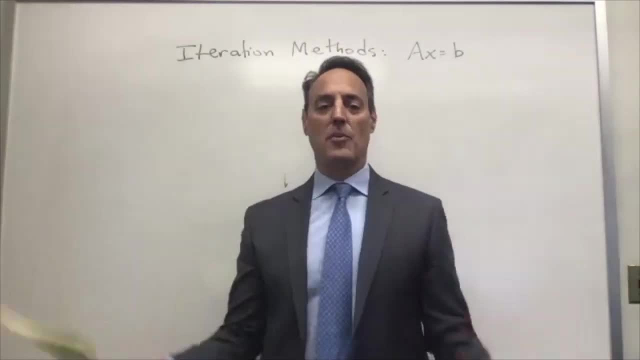 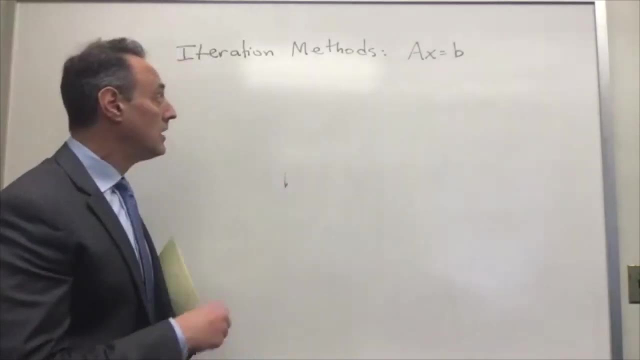 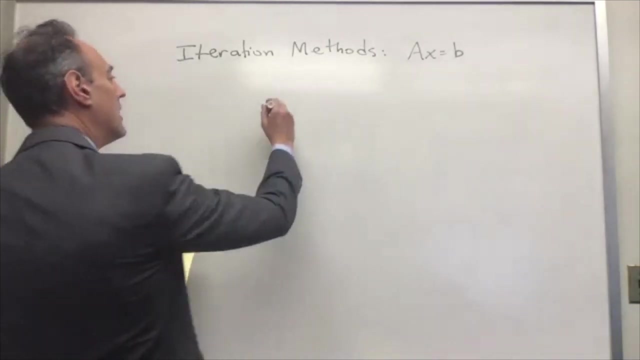 that question right is: why would i do? this is just a, just another way to solve ax equal to b. but why not just use lu or gaussian elimination, because we've learned how to do those. but i want to highlight something, and the thing i want to highlight is this: progress in 1950. 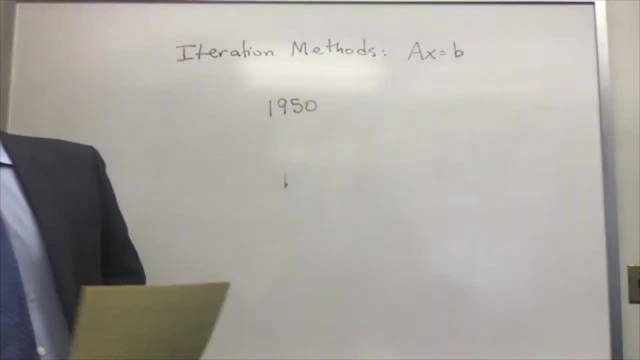 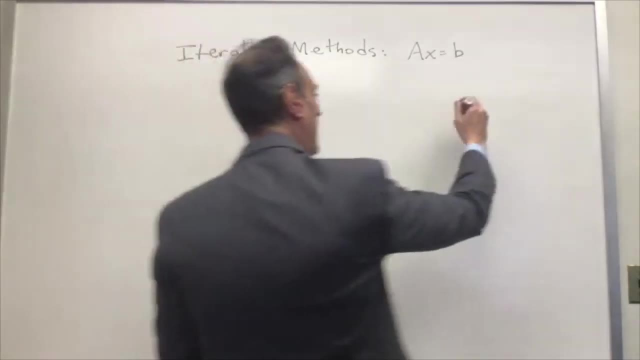 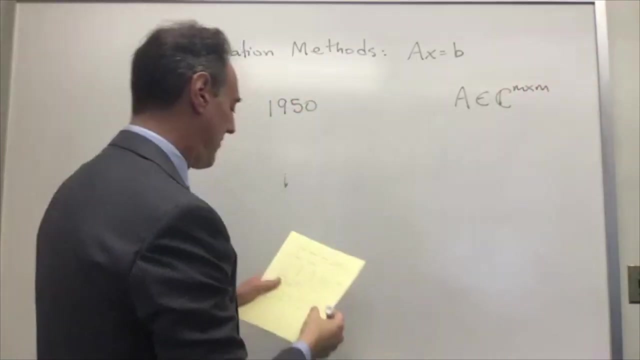 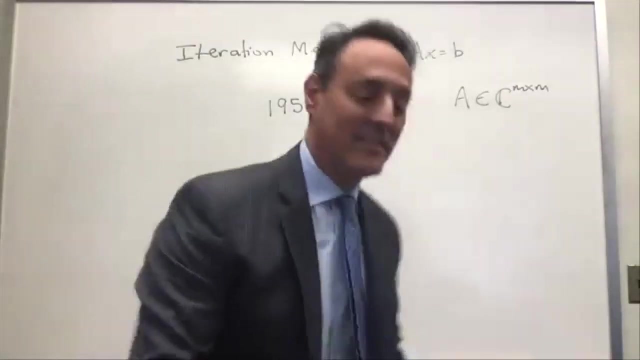 uh, i'm looking for another pen here because this one's not very dark- 1950. what we could do computationally is matrices. if you think about a matrix which is m by m 1950, we could solve these being about n equals 20.. so not very big right. you remember this is the inventions of the computer, so this: 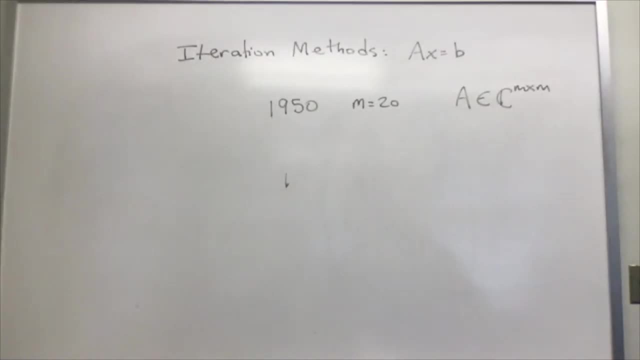 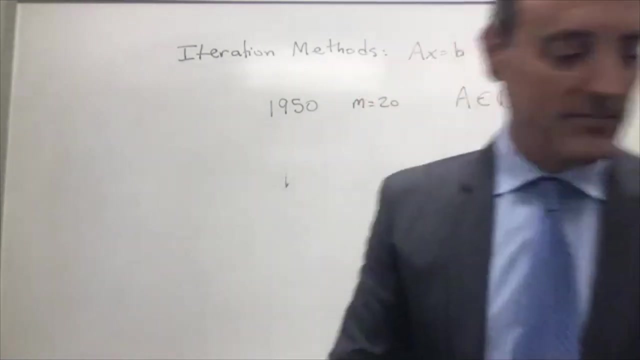 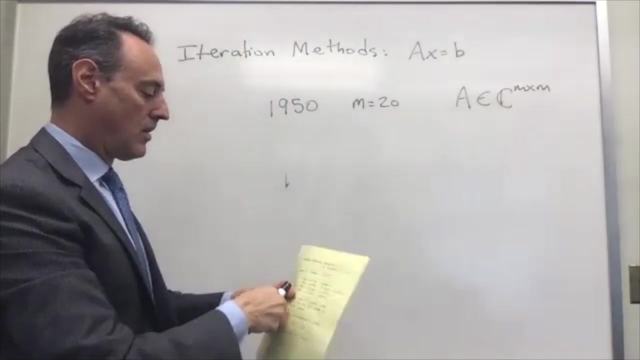 was very slow. all right, i'm gonna get a new pin here because that one is not to my liking. all right, so let's go ahead and do this. let's progress forward in time and let's notice how well things progress. let's jump: fix 15 years. 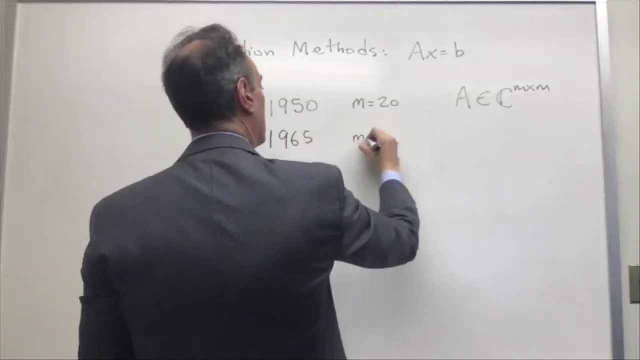 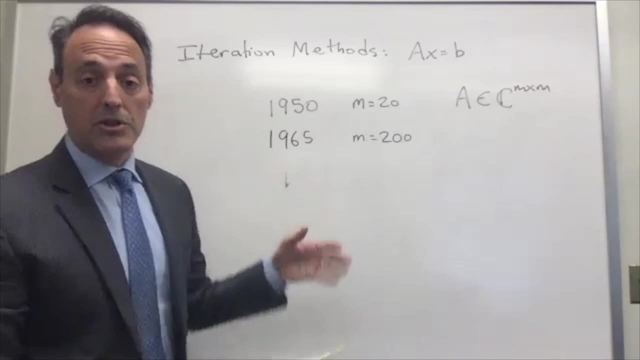 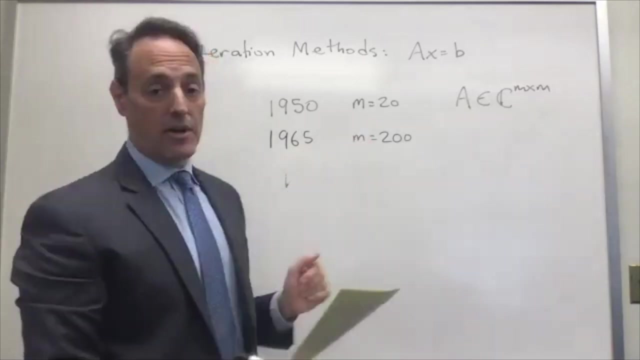 to 65.. uh, you're about an order of magnitude bigger matrices you can solve numerically. remember we still don't have pcs or or computers just available to anybody 1965. it's still pretty hard to get a hold of these and there's people that have them, but it's not widespread. 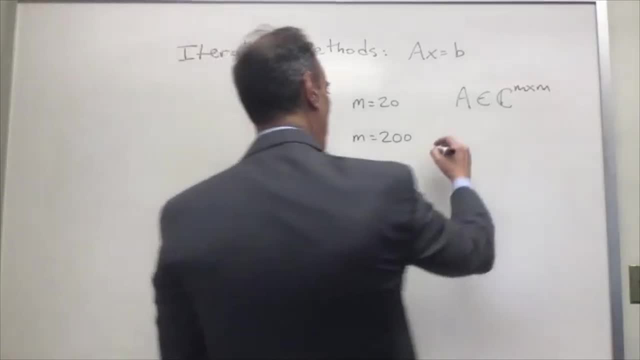 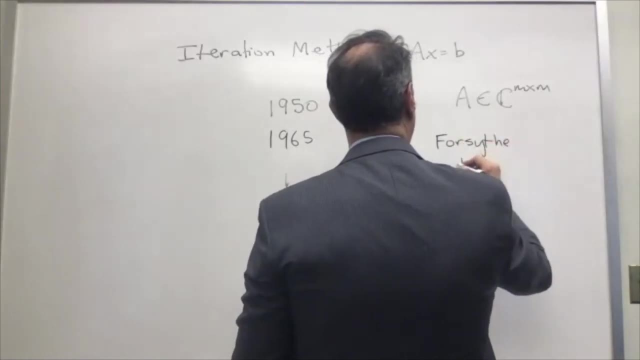 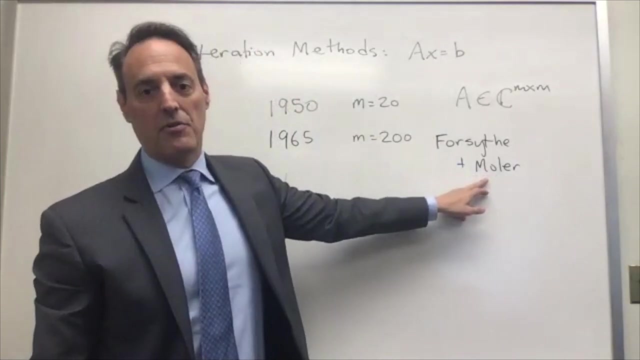 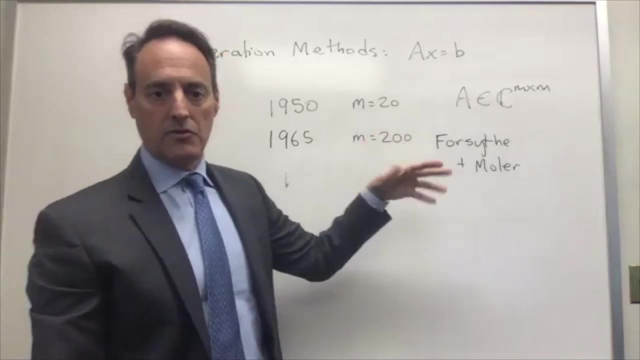 so you can kind of do methods about this big and i want to put some names down here: forsyth and moeller and cleve moeller- he is the founder of matlab. so he was- uh, he actually, i believe, was- working at stanford at the time he started thinking about numerical linear algebra. 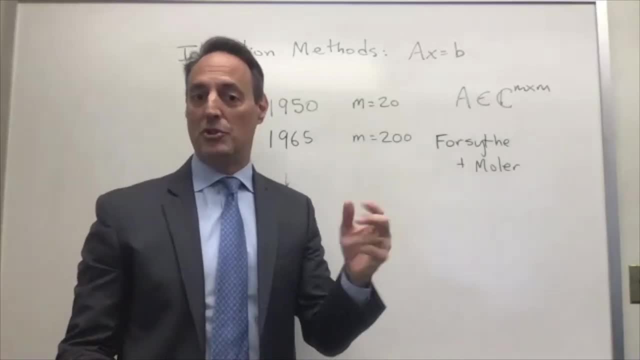 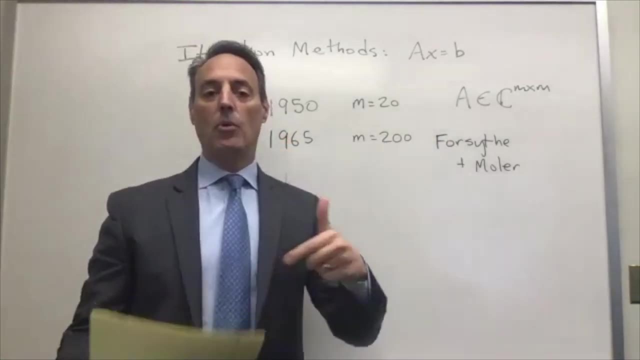 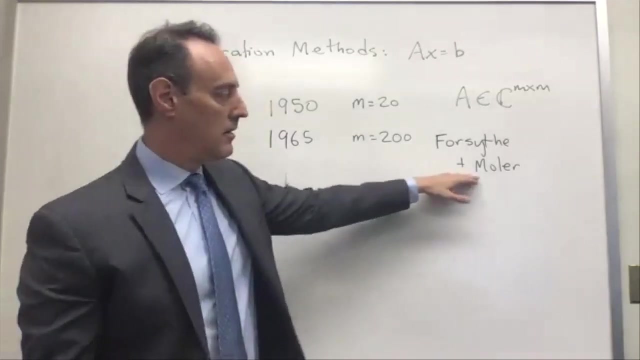 and he came up with matlab, which is a method that we're going to use to solve numerically linear algebra, which is matrix laboratory. so at that point is when you started to see more and more access to computers by everyday researchers, okay, and moeller started developing this software. 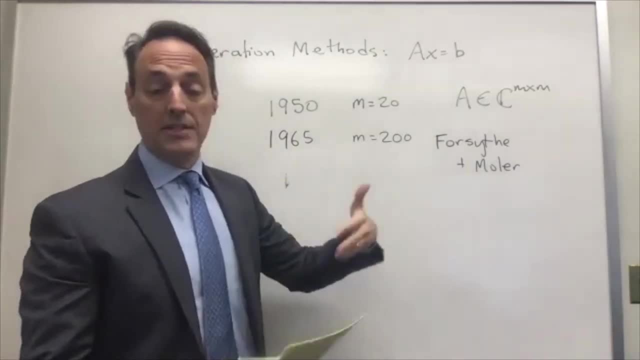 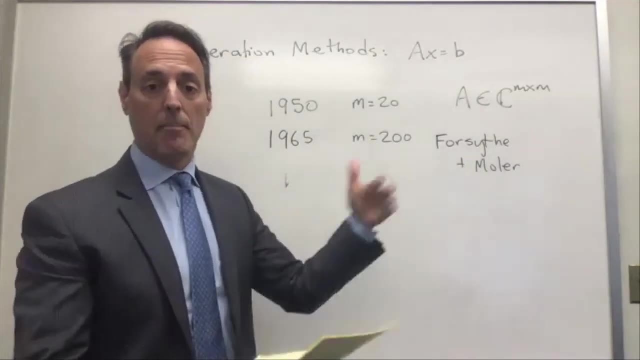 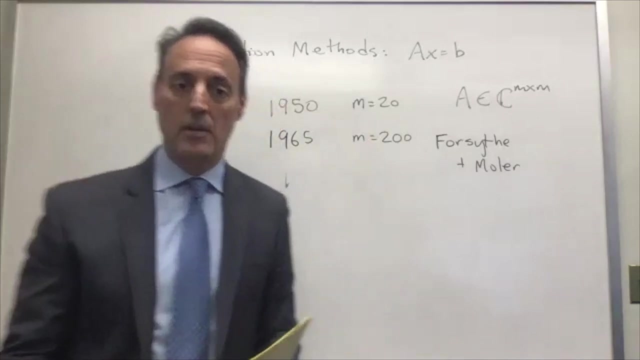 package which would allow people ease of use and the ability to do these computations- uh, you know- in a nice way. so he was really importing, taking modern research and putting it into a computer framework where everybody could just use it. okay, so this is 1965.. 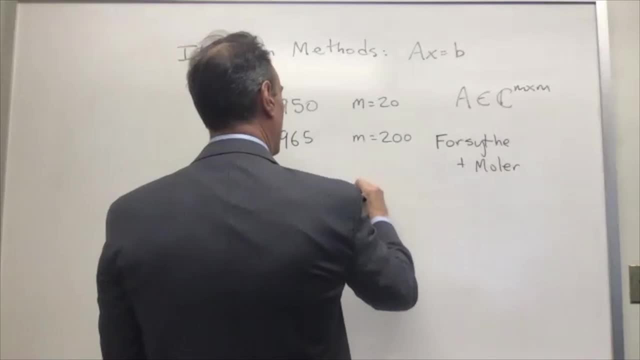 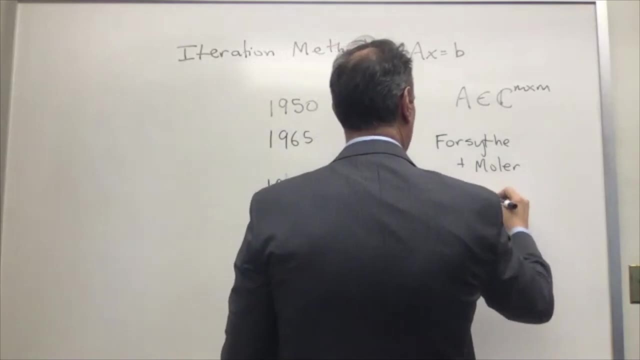 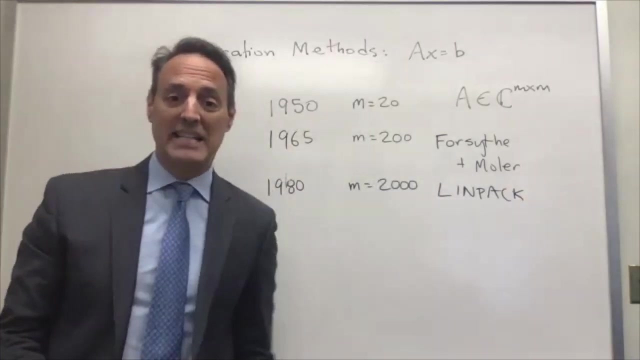 vance another 15 year, then you're around another magnitude up and this is really coming into linpack, which is a linear algebra package, and then you could start handling matrices about size 2000 by 2000, and then you could start handling matrices about size 2000 by 2000. okay, so you're starting to get bigger matrices- 1980. uh. 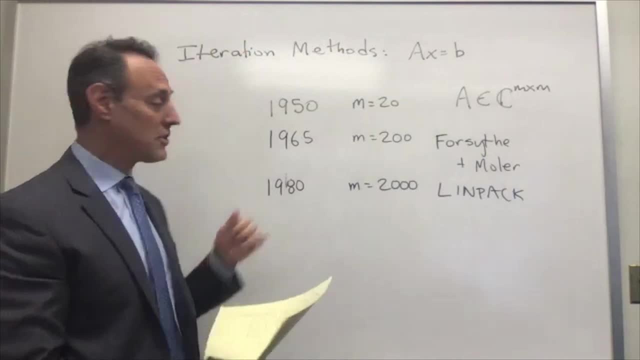 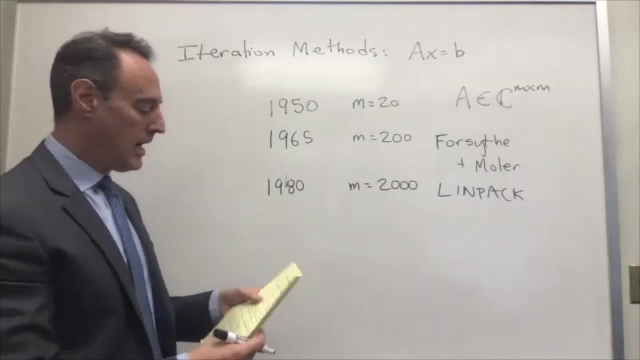 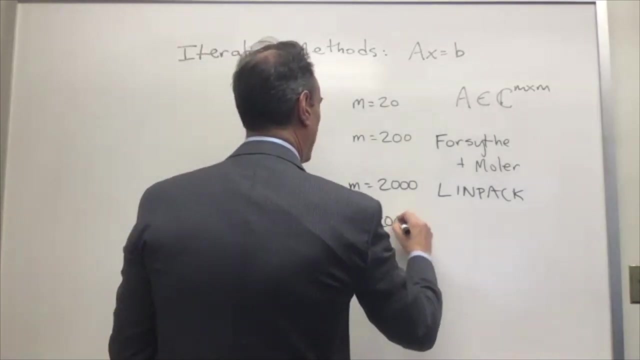 it's a long time ago, right? so this is like 40 years ago, and so we're starting to get bigger patches, but still pretty small for what we want to be doing. um, and then 1995, get yet another word of magnitude: now you're in the 20 000 by 20 000 range, and this is done with. 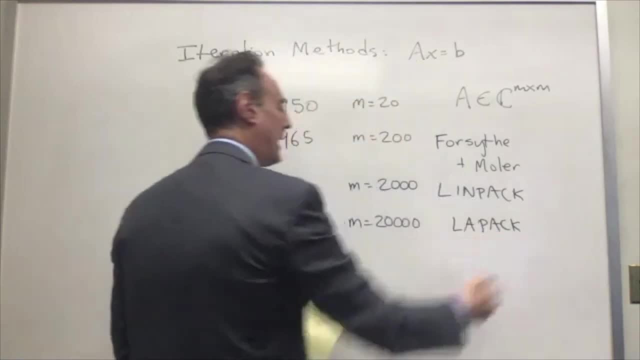 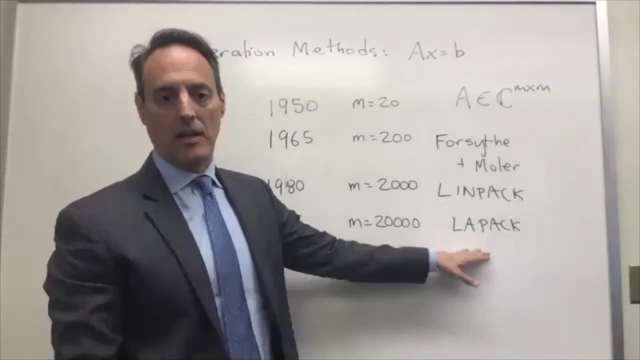 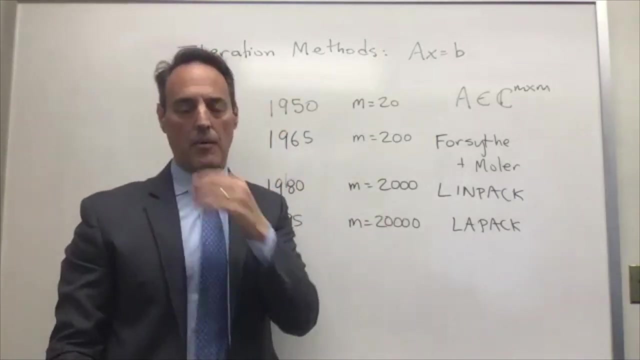 la pac linear algebra package, and this is still sort of the state of the art stuff. so a lot of the best packages always get migrated to l la pac so that you can actually use them, okay, so there's this migration. now the here's. the here's the thing i want to highlight, and this is something that was 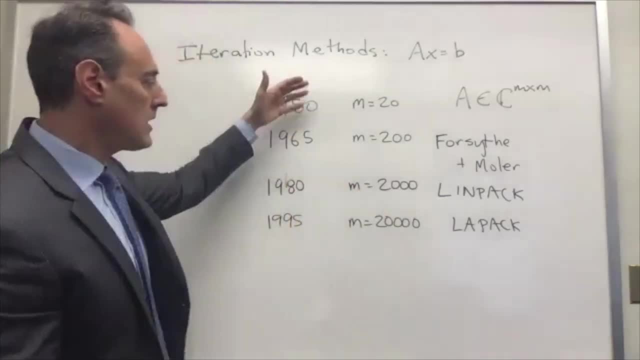 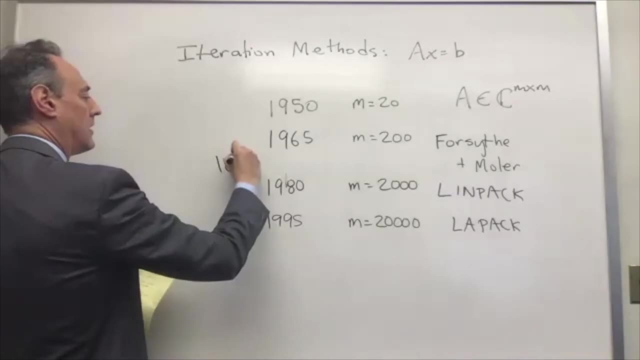 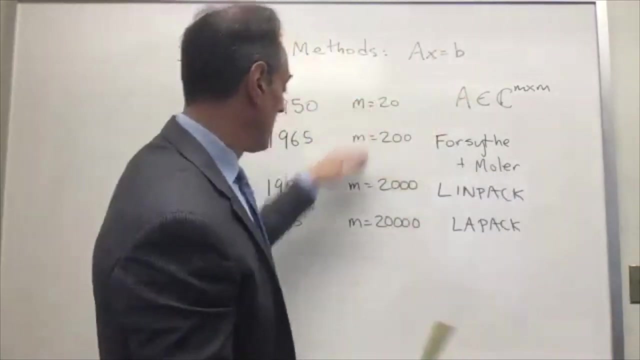 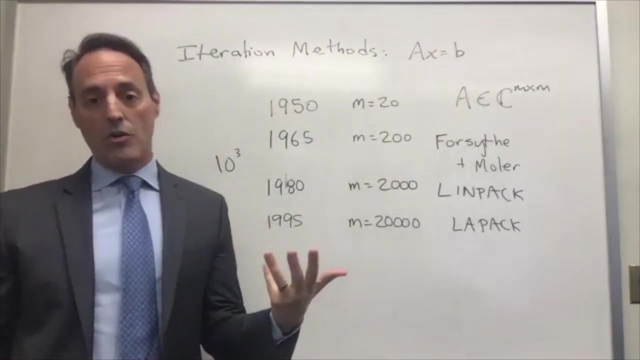 highlighted by trefethen in his book is that if you notice over this time period, you notice we got three decimal places, so this is like a ten to the three increase, so three orders of magnitude larger problems in this 45 year span. now what's interesting is that: well, how did hardware do how much? 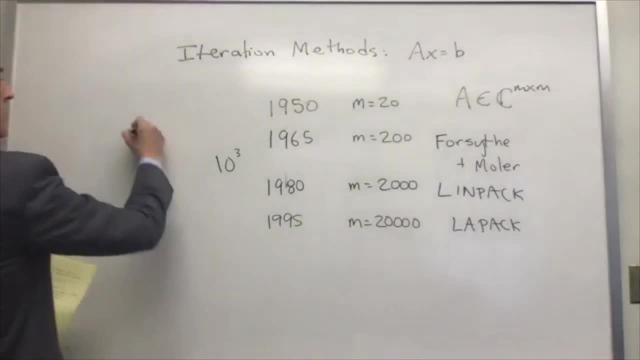 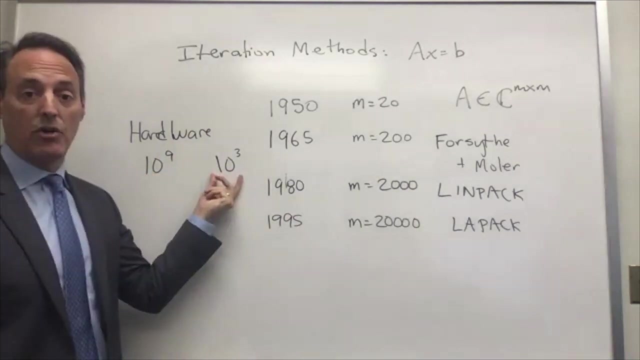 faster and bigger was hardware going and on the hardware side hard, where you got an increase of like to ten to the nine up. so this got ten to three bigger in problems. this is ten to the nine. so this is interesting. this got a really big increase. this actually only went three average. 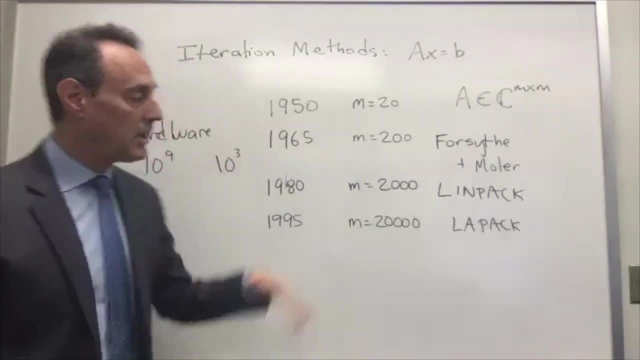 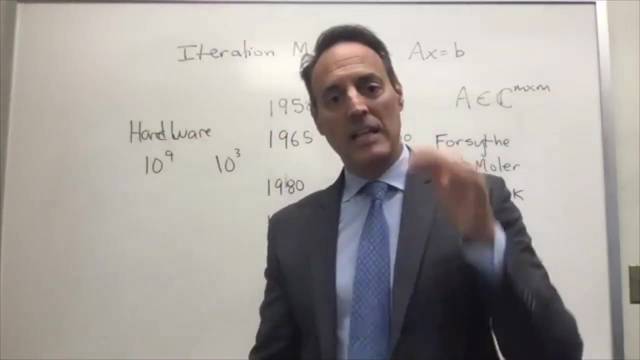 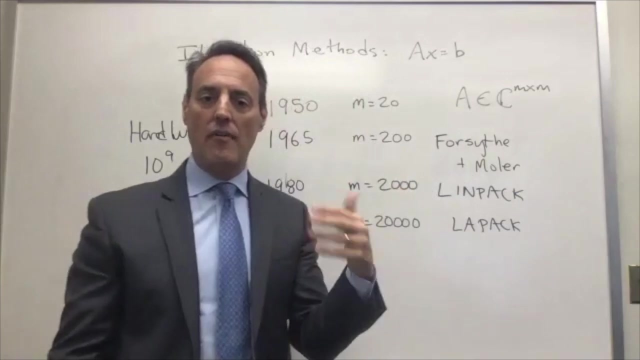 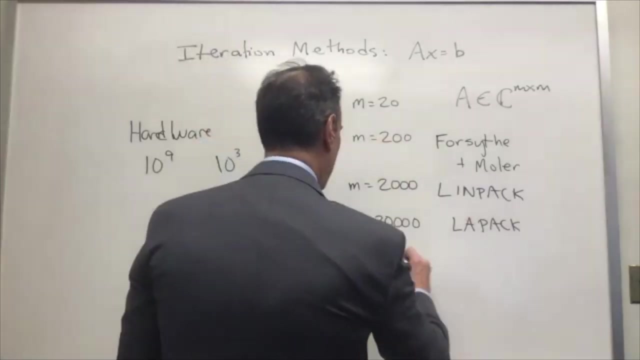 magnitude, that with nine order from magnitude. and why is that? because if you notice most the packages here or most of the methods we used here, like lu decomposition, like gaussian elimination, like svd or qr, these things are often is m by m, their size, order, m, cubed operations, right. so we're still talking about 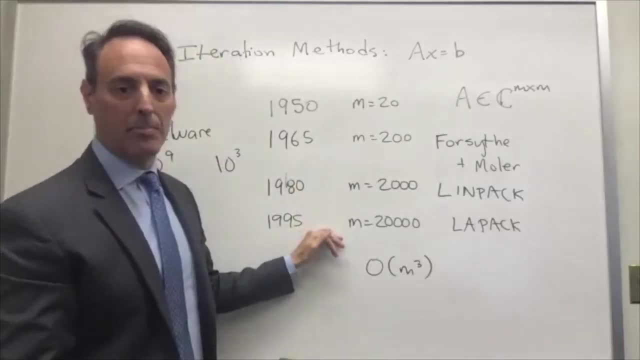 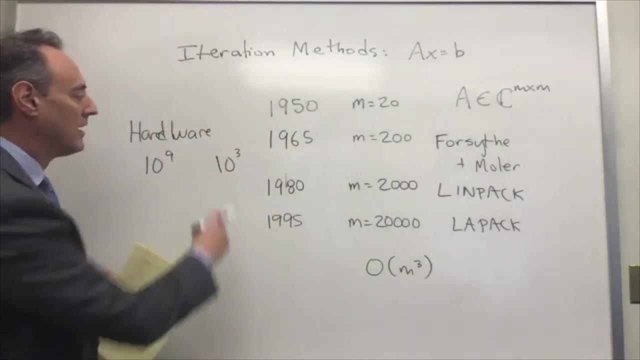 to compute ax equal to b solves cost you m cubed. so look at this went up by 10 to the 3. but since these are like m cubed, this is like 10 to the 3 to the cube power, which is 10 to the 9. 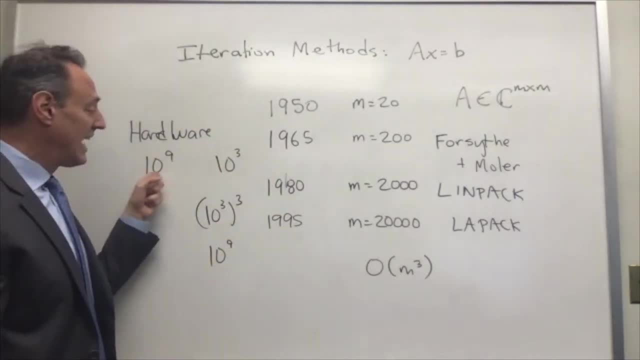 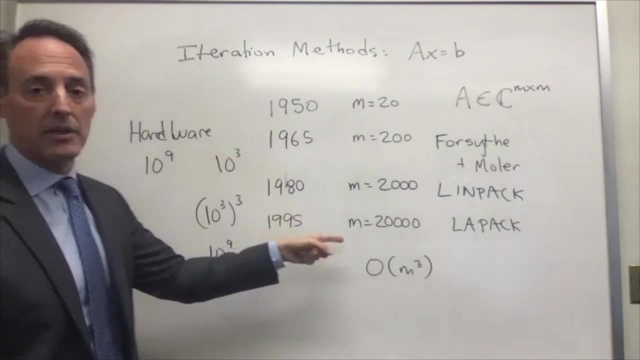 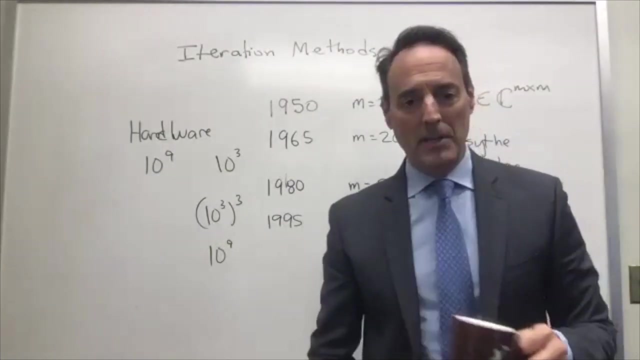 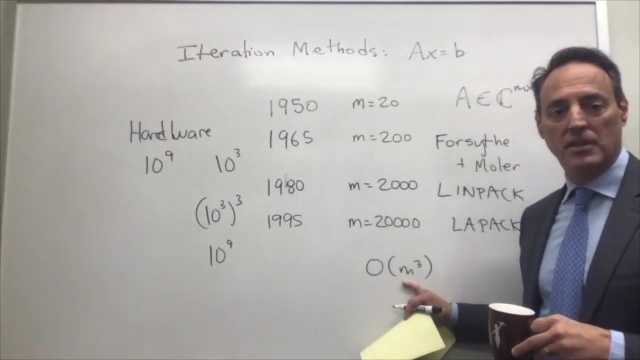 so there you go. we had to get a 10 to the nice increase in computational hardware abilities to get a 10 to the 3 increase in solving matrix sizes. so what's the problem? the problem is that this is the bottleneck right there. this is a bottleneck for solving large-scale computational problems. it costs you 10 to the 3. 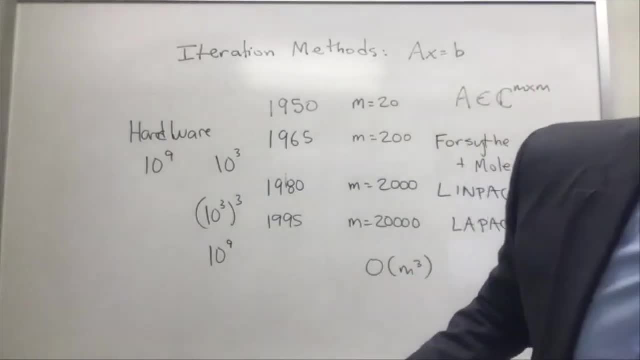 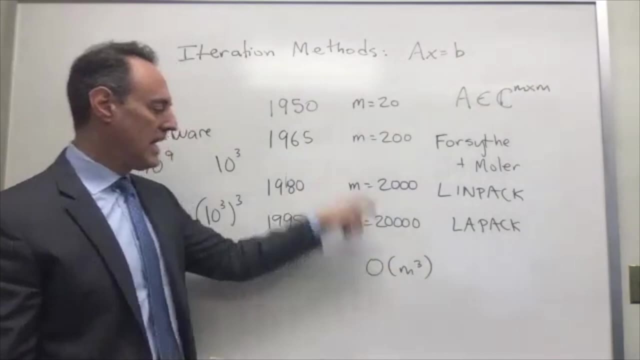 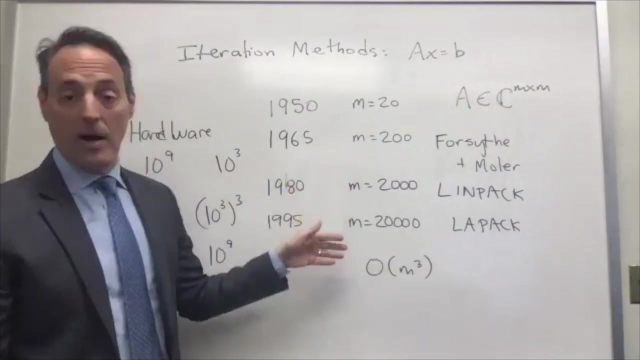 so the entire game around scientific computing is to figure out. is there a way to circumvent this? how do i beat this? because as long as this is sitting there, right, if you look at our advances, every time you want to go up one order of magnitude, you're going to have to do 10 to 3 orders of magnitude in your hardware. 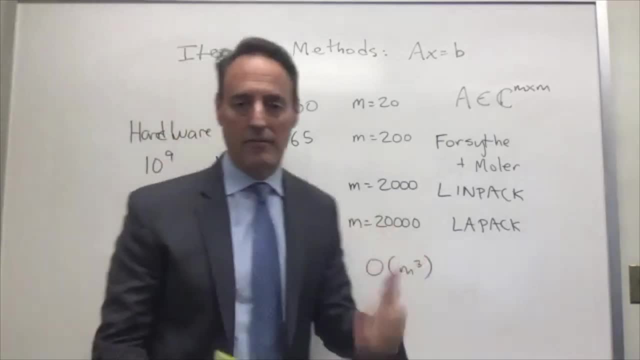 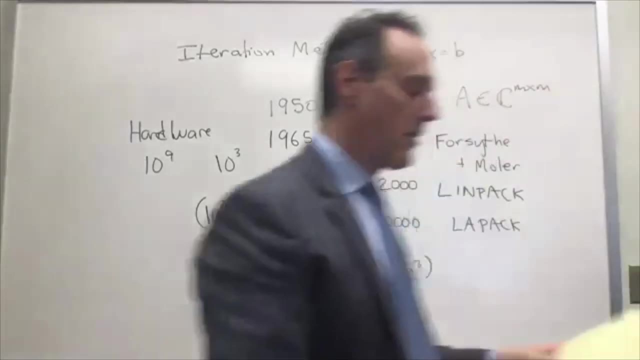 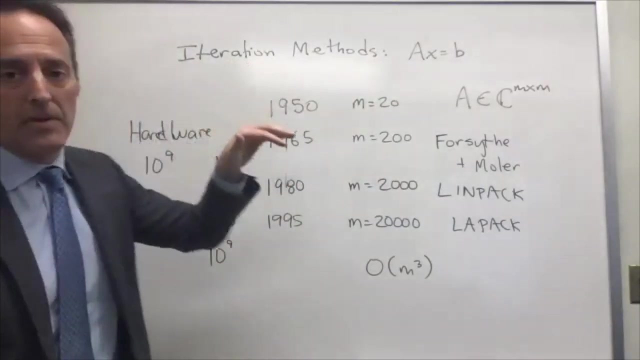 development. okay, that's a really tough uh thing to keep up with. okay, so you really want to to get around this 10 to the 3.. So people started thinking about other ways to solve a x equal to b, and that's why we're talking about these iteration methods, because the iteration methods are methods. 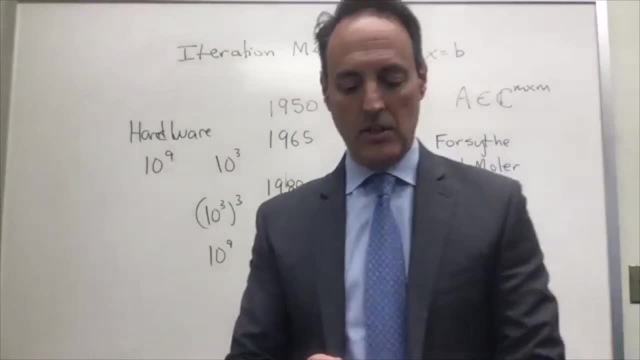 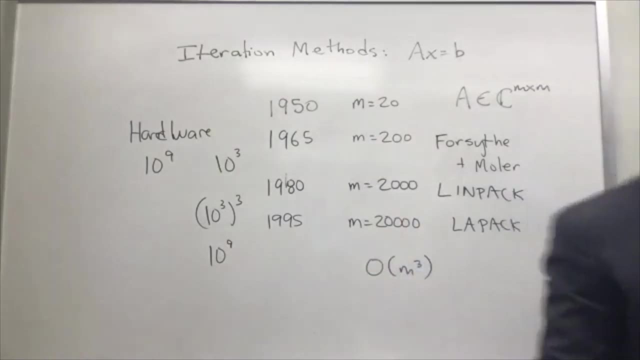 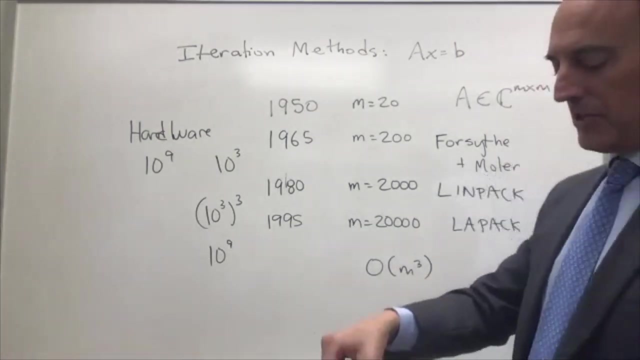 which gives us at least the potential in certain cases to beat this m cubed operation counts to solve a: x equal to b. Okay, so let's go ahead and talk about some of the methods out there. We already talked about Jacobi Gauss-Seidel, but let's talk about more sophisticated methods. 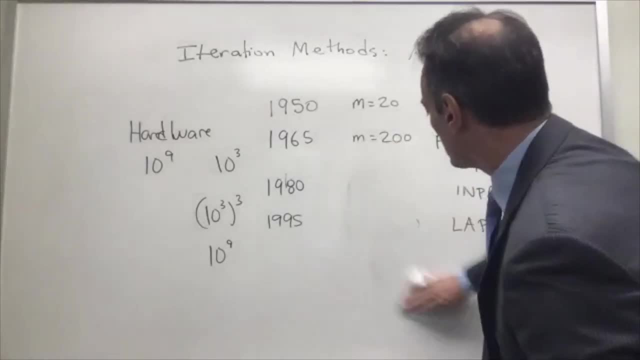 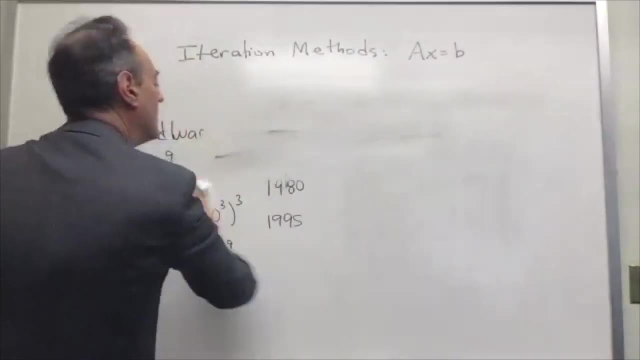 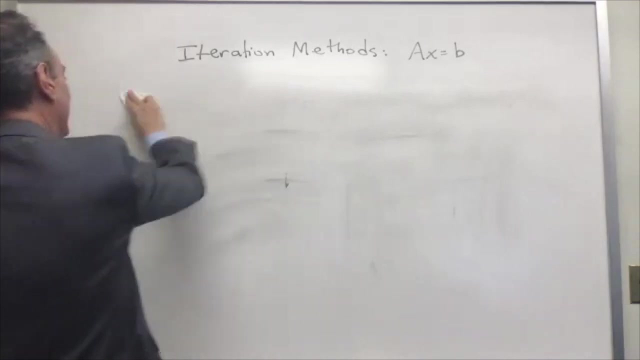 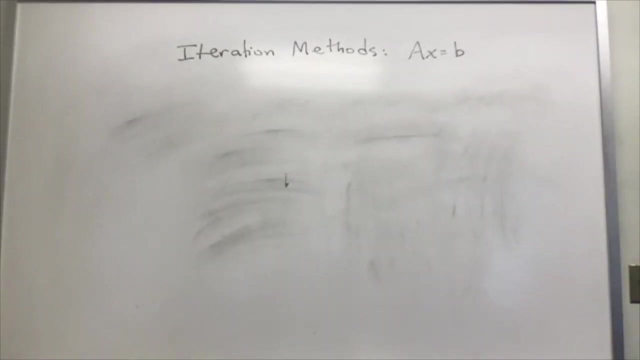 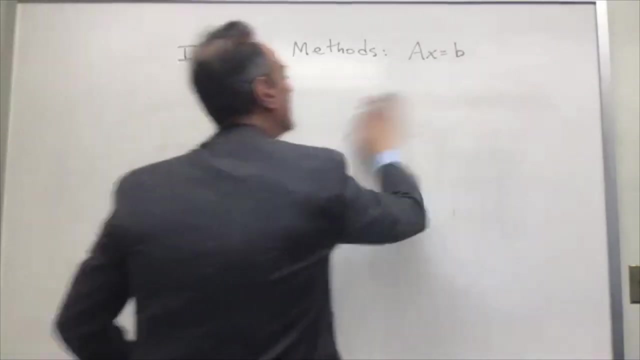 that you'd actually use in practice. Uh-oh, that didn't erase very well What's going on there. All right, All right, Let me get some water on that board. Can I ask a question? Yes, So you mentioned. it basically goes up to 20,000 by 20,000 or 200,000 by 200,000.. I'm just wondering. 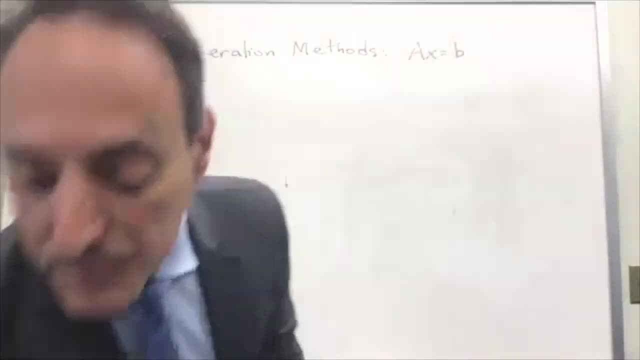 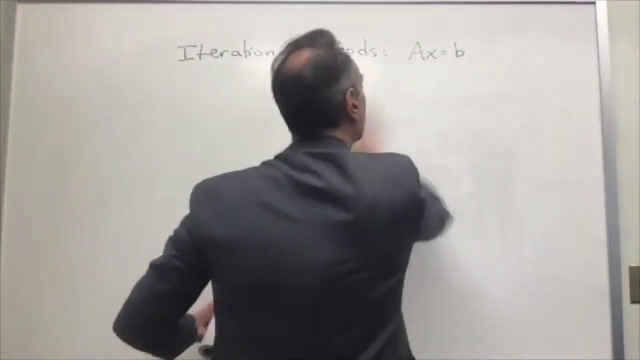 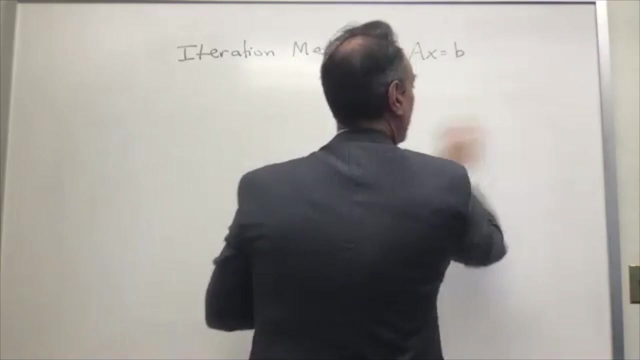 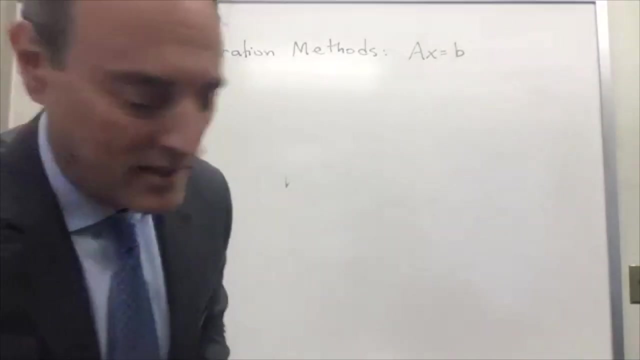 20,000 by 20,000. That was 1995.. Okay, So is it common for the real port problem to be that size, or it actually exceedingly greater than that? Nowadays it's much, much bigger. You know, we want to solve, for instance, if you work for Boeing and you want to solve for fluid flow. 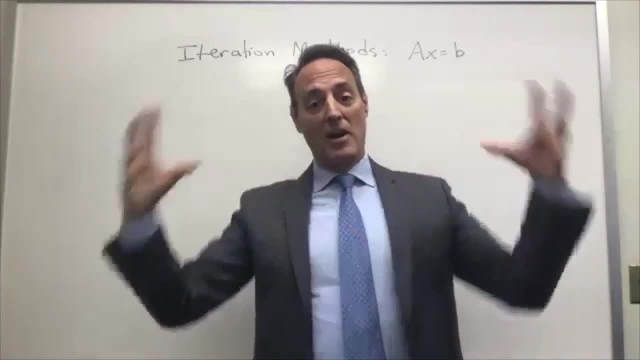 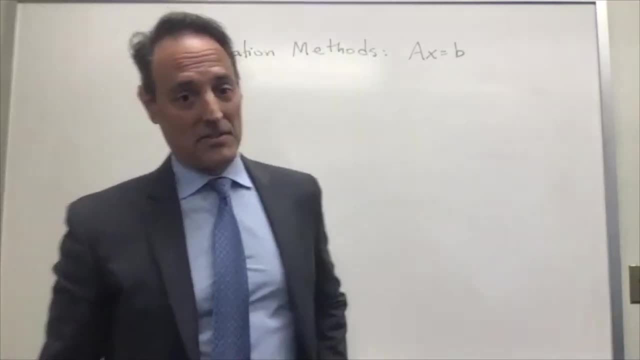 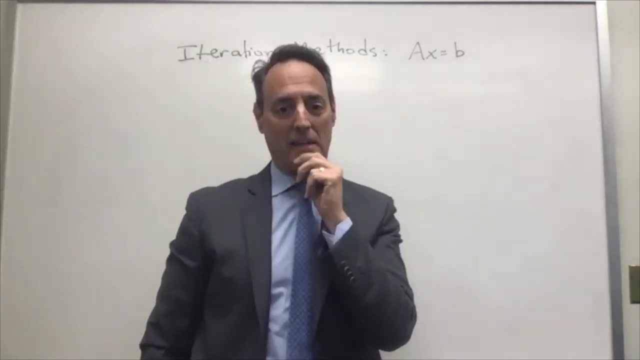 around a design in airplane right and start numerically solving for this. you know, for the fluid flow around airplane you might want matrices that are billions by billions. Let me say it this way: There's no matrix you can make. that's big enough that people would go. that's too big. 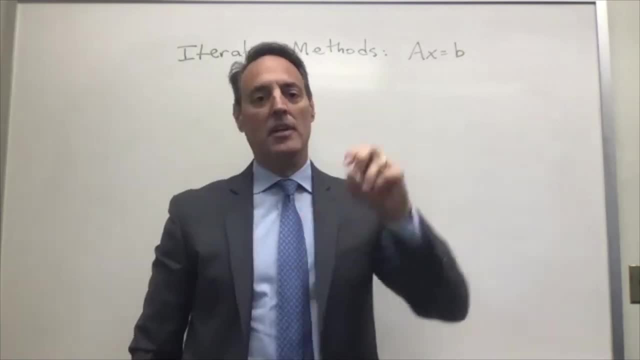 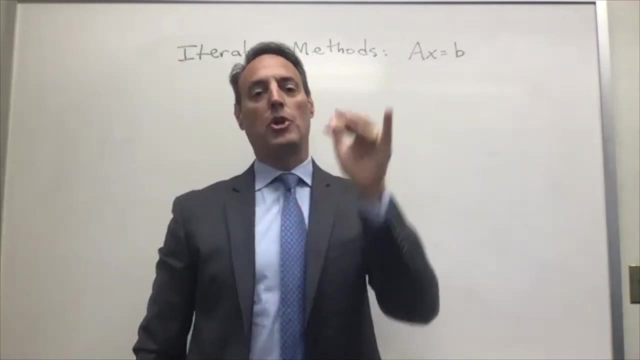 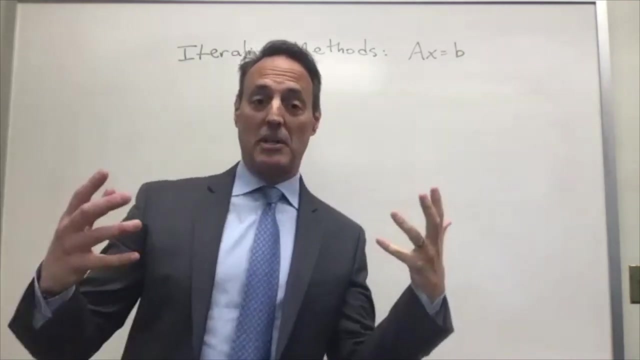 What everybody wants is they want bigger, faster. If you tell people I can solve trillion by trillion matrices, tomorrow people will show up to you and say: here's my problem, that I need a trillion by trillion matrix. You know people are doing now simulations of galaxies, right? 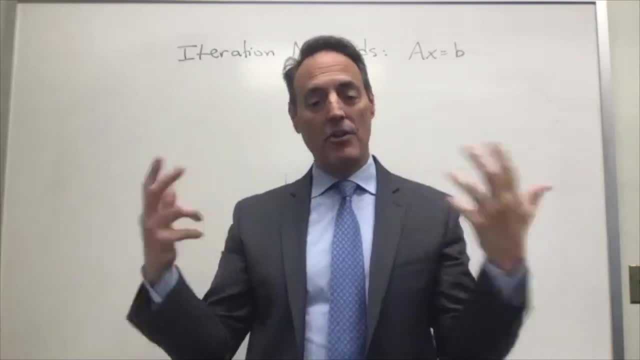 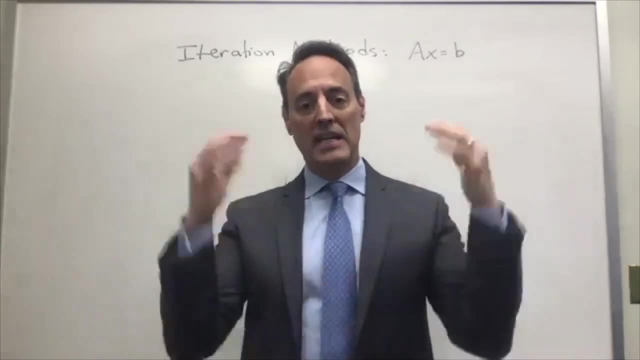 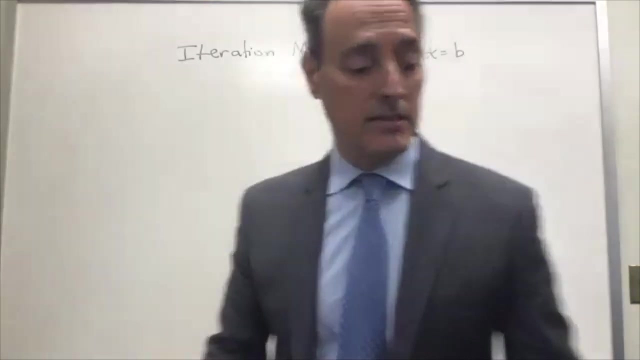 This is massive simulation And the only thing limiting them is they can only do certain size simulations limited by the largest supercomputers in the world, And that's their hard limit. That's the biggest they can do with memory and solutions and solution techniques. 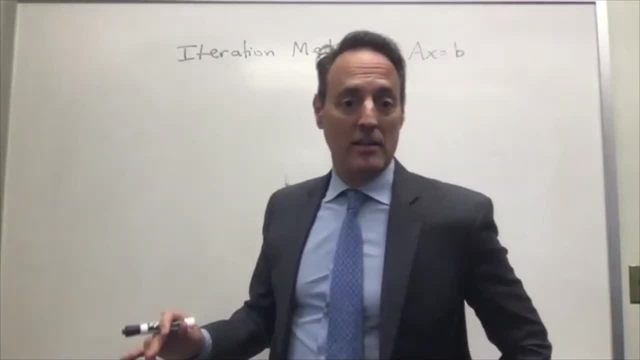 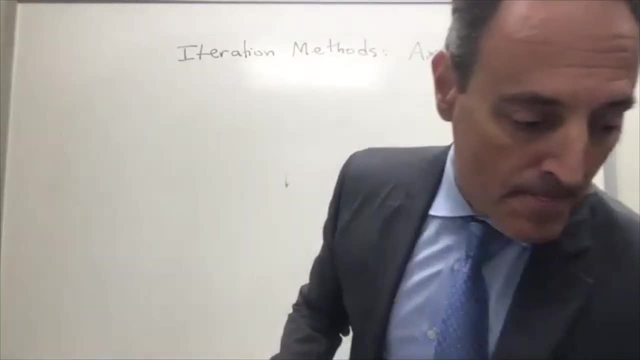 So there's no. there's no upper limit is the way I think about it. You build it, people show up with problems And they want to do it fast, So all the algorithm that you use today are basically limited to one computer. 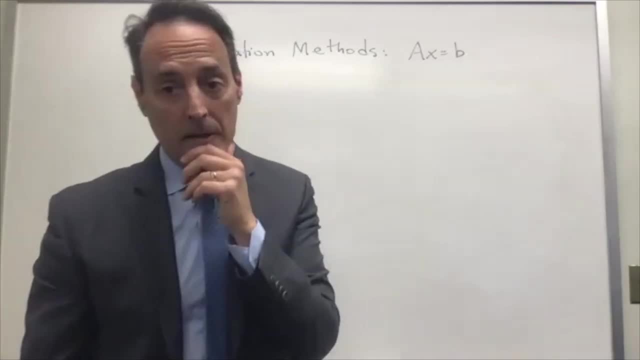 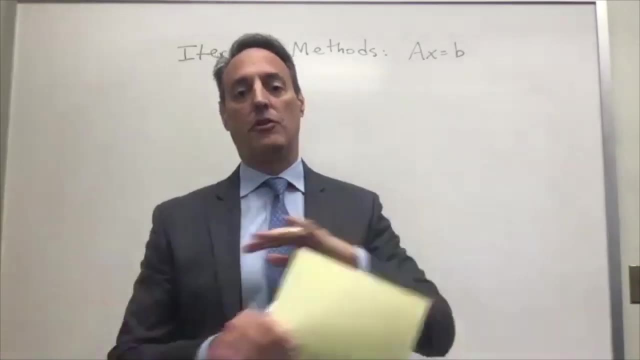 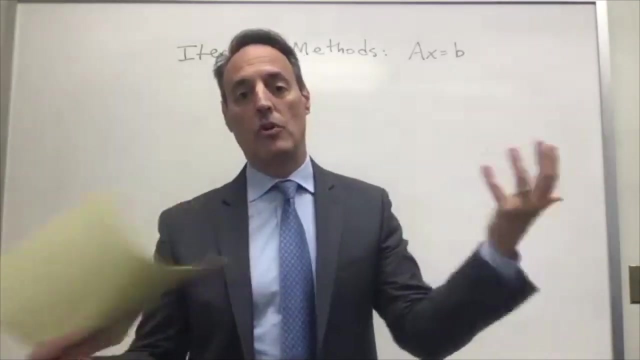 We never thought about, like, for example, Harz. People do all kinds of methods where they can also. Oh no, no. people do all kinds of methods where they can also. They do whatever multi threading right, And so you spread out the computation across across GPUs or CPUs, and then you so multiprocessors. 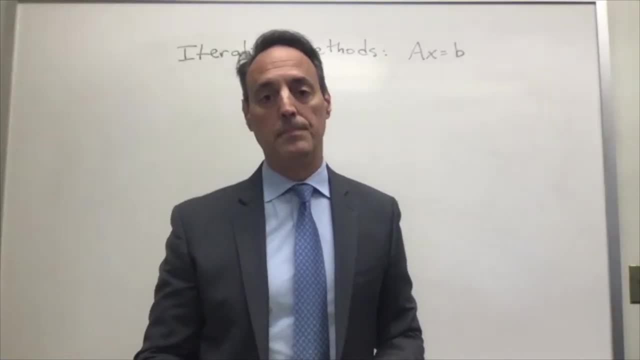 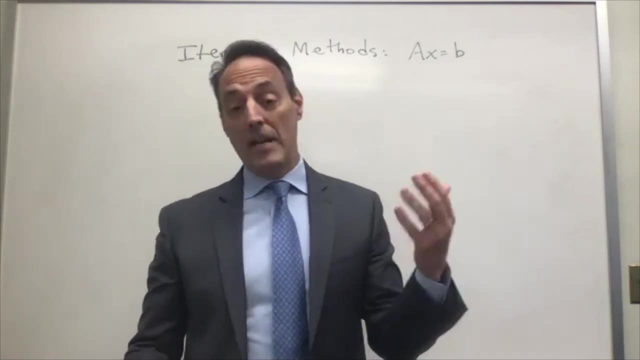 Yeah, you can do. you can do lots of algorithms that take advantage of this too. So in that sense there should be no limit at all. right, Because you can, theoretically, Theoretically, you can, you know, but then there's limits of hardware communication, right. 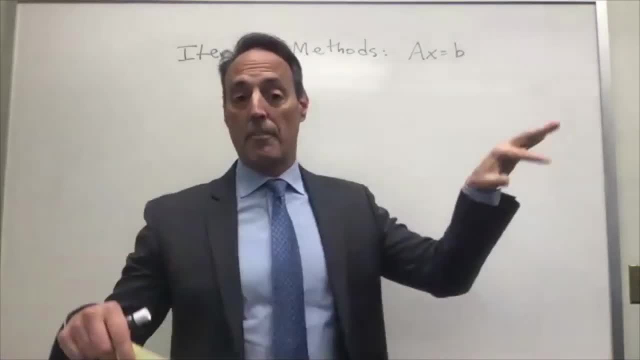 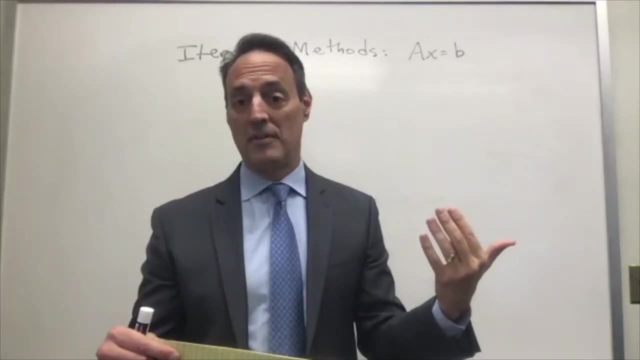 So oftentimes when you solve these, Even if you can solve them, You can break it apart. So iterative methods are really nice for paralyzing, Except for you still have to make them talk to each other At some point. all the local computations still have to be integrated into the final solution. 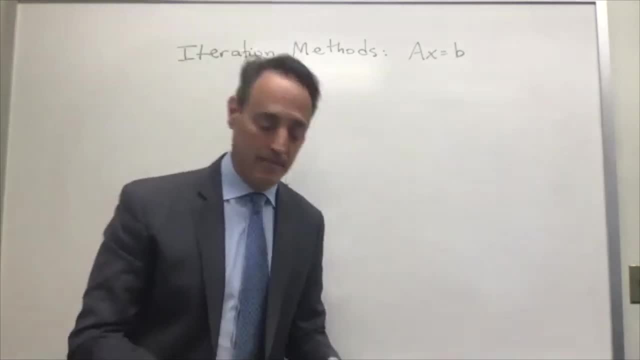 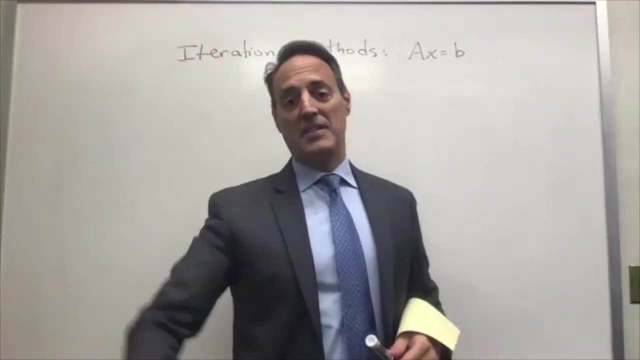 I see, So that becomes a bottleneck. eventually Got it, Thank you, Yeah, So we're going to, really. So what we're talking about with iterative methods is exactly all these things is, how do we get around this issue of this M cubed? 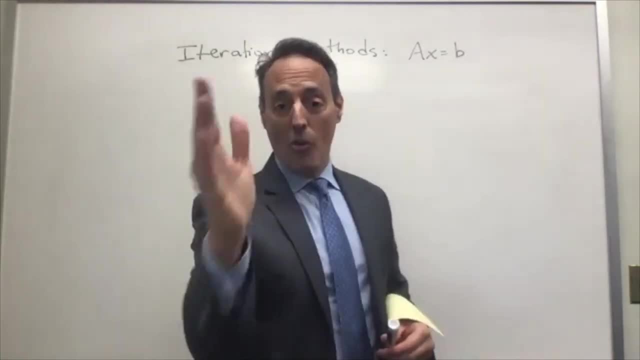 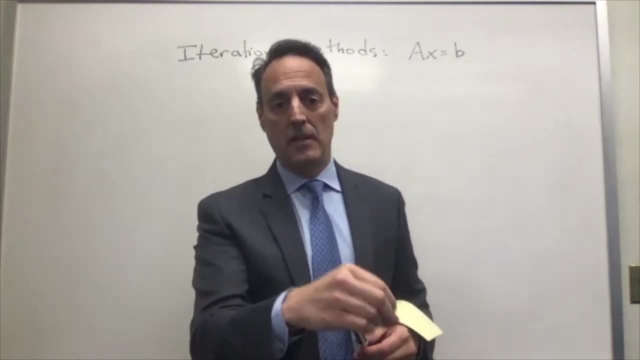 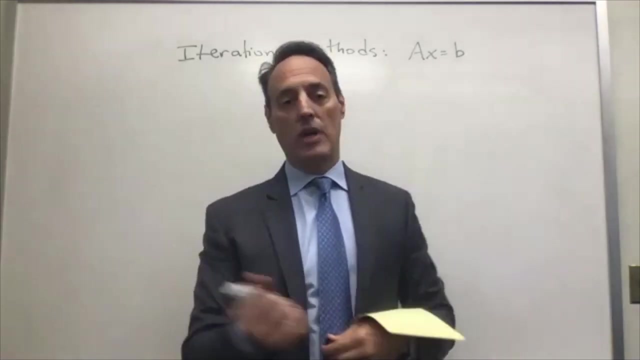 In other words any of the really large scale problems. Nobody is doing Gaussian elimination. Nobody. You're always doing something else that's faster. Nobody can afford, even today's problems, to say: let me go do this big fluid flow example, You're not going to do Gaussian elimination on it. 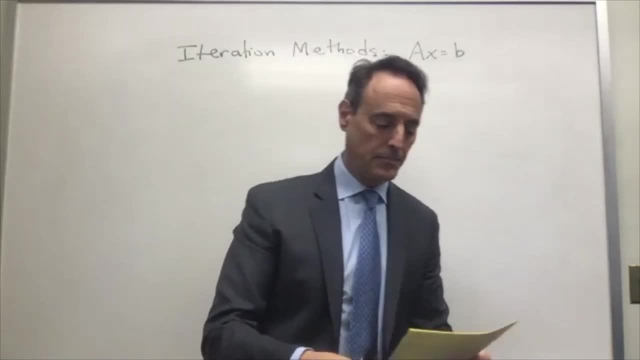 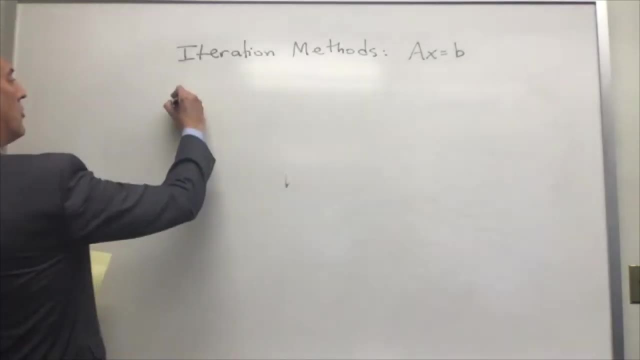 You're going to do something much more sophisticated, And so this gets us into the iterative techniques, and let's talk about it in a more formal way. I'm going to introduce to you The idea of what's called a Krylov Subspace. 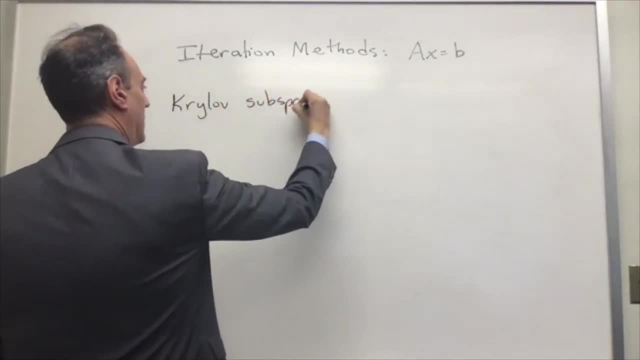 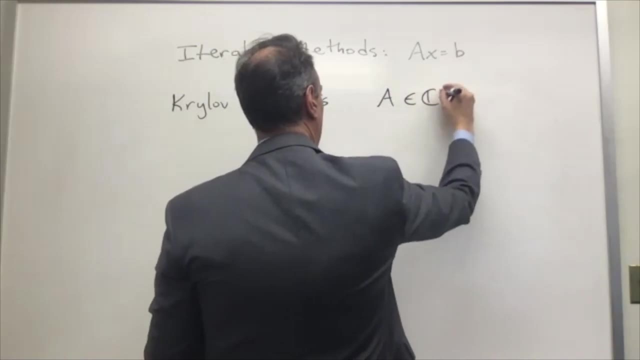 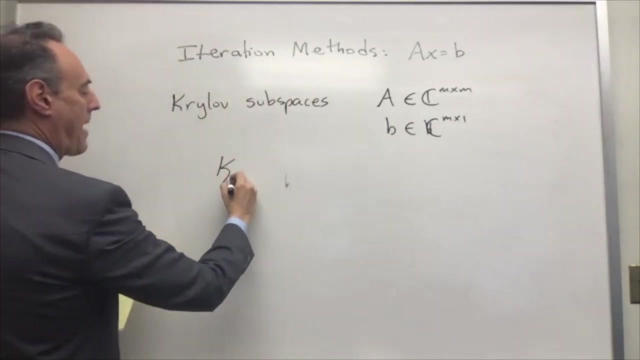 So I'm given a matrix A And some vector B And what I want to do is think about what a Krylov subspace is. And this is a Kappa And the N. I'll tell you what this is in a minute. 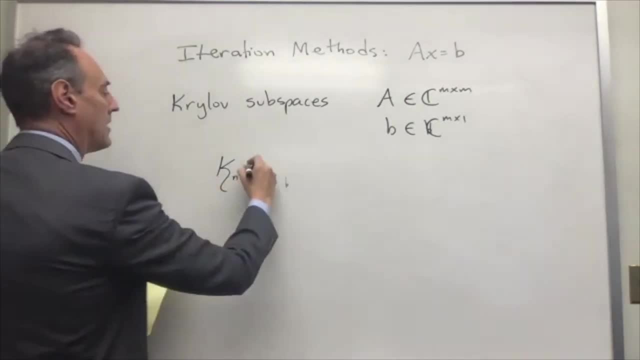 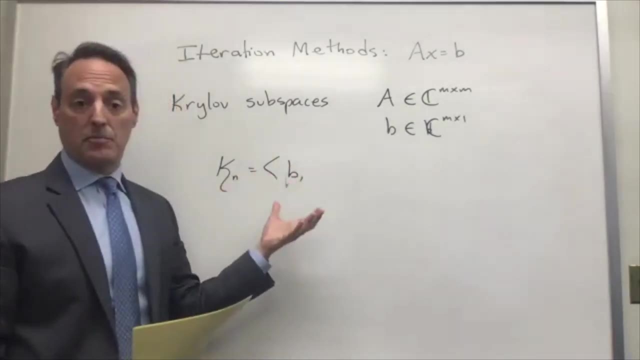 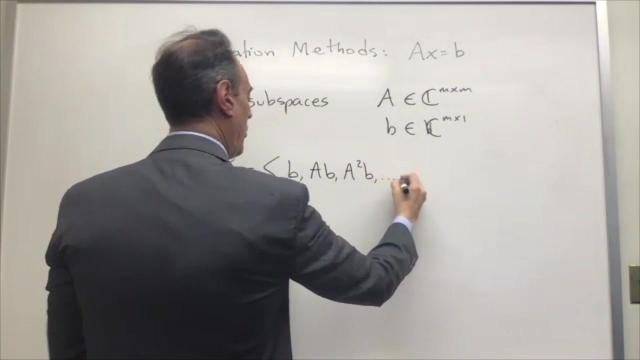 The Krylov subspace is span here, or the subspace of this is given by the following set of vectors that spam this subspace. So the vector B, A times B, A squared B, All the way up to A, to the N minus one times B. 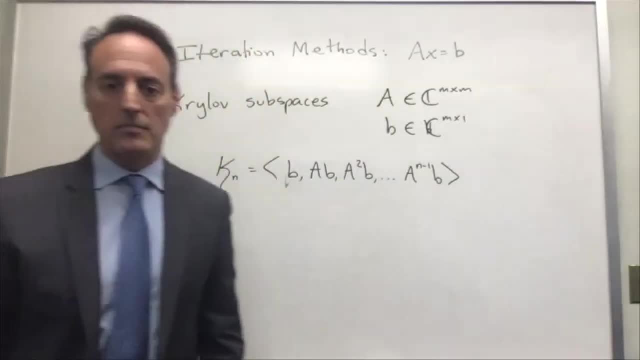 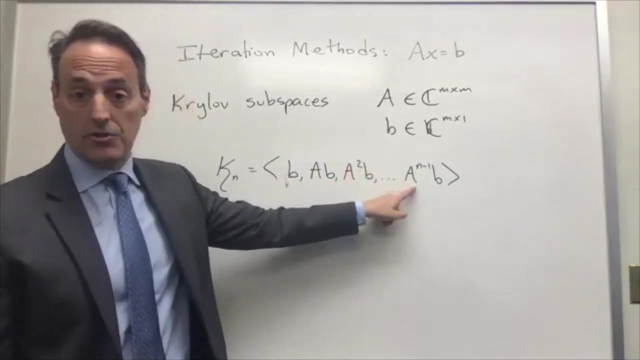 So I'm looking at the subspace that this forms. Okay, So this is what I'm doing- is a squared. So this is, in some sense, This is an iteration structure. right, I hit B with a, hit it again, Hit it again. 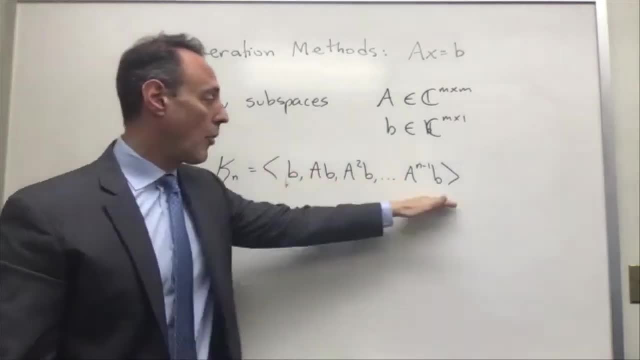 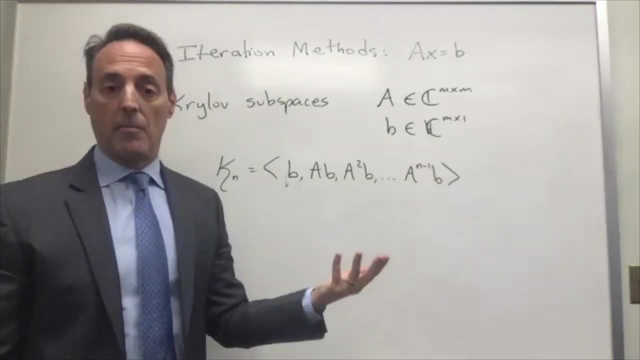 Hit it again And minus one times, And then what I'm looking for is the set of vectors. This is the Krylov subspace. How am I going to take advantage of them? But the other thing you know about this Krylov subspace, since I have 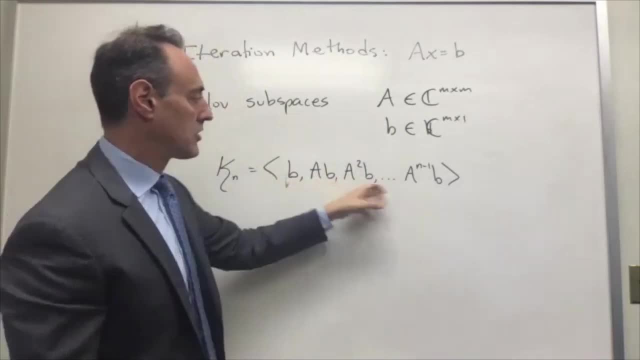 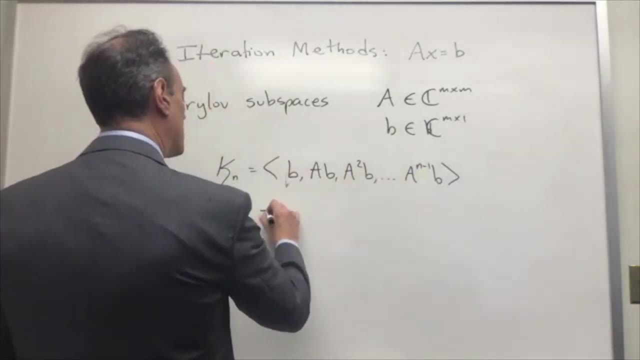 These In directions right, First direction, second direction, all the way to N minus one. I started with. N equals zero, So this N of them total. I could, in fact Span this with a set of vectors that are: Or the normal: 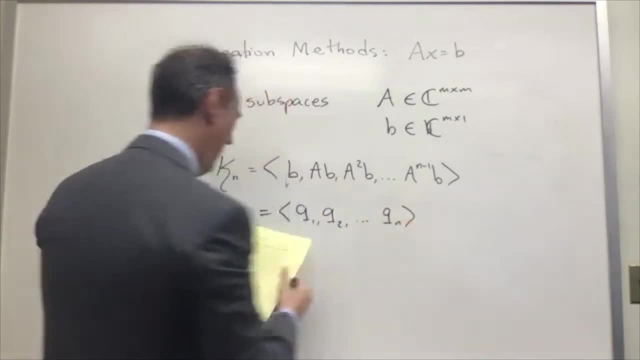 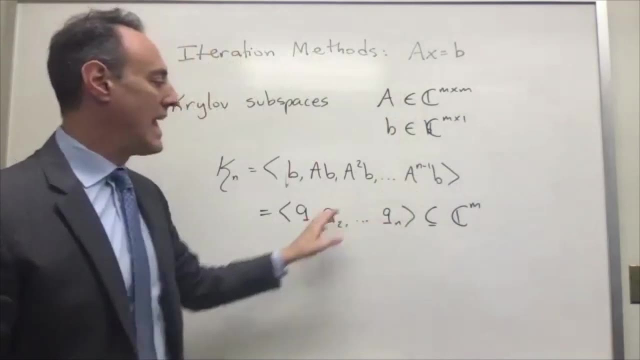 Okay, And these are a subset Of the end dimensional space. Notice, I'm only going to end dimensions. So out of this end dimensional space, I define An end dimensional subspace in this fashion, Which brings me to the next step. 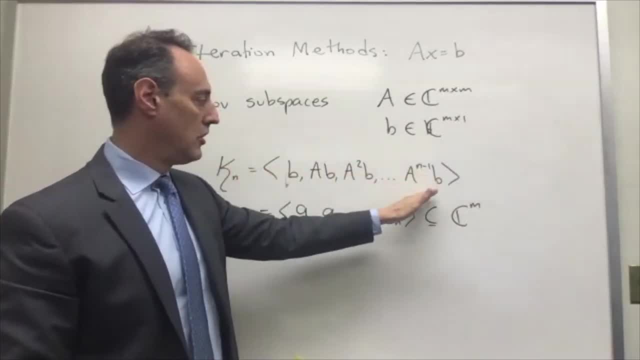 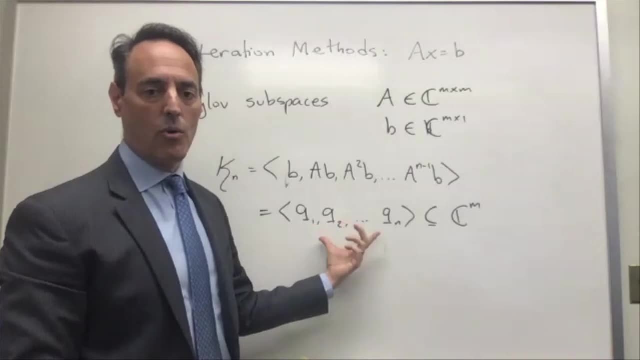 Which brings me to the next step. Which brings me to the next step, Which brings me to this end dimensional subspace. Which brings me to the next step, Which brings me to this end dimensional subspace, Which brings me to the next step. 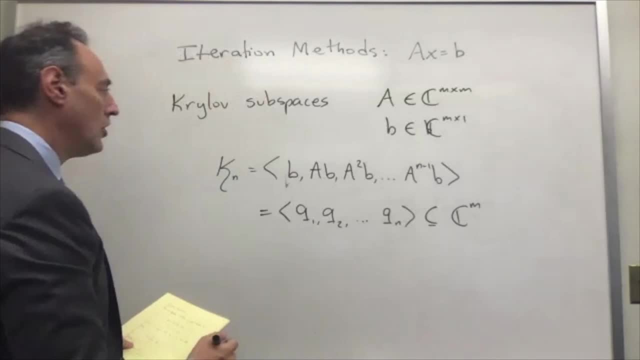 Which brings me to the next step, And that is, by the way, I could say: well, if this is an end dimensional subspace I could come up with, instead with an orthogonal vectors, By the way. how would I do that? 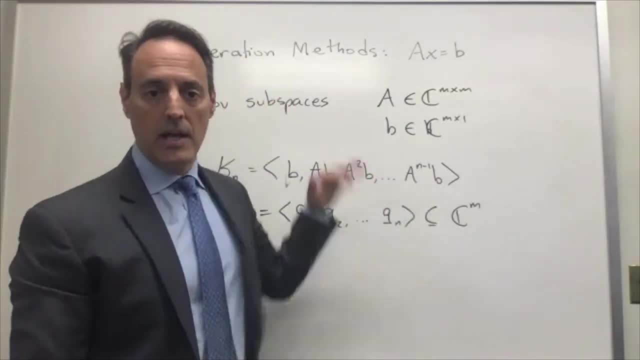 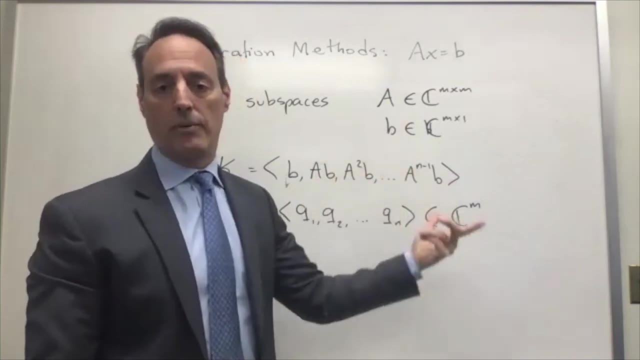 Well, I would define. I'm going to do this with the QR decomposition, Remember. the QR takes a set of vectors that aren't necessarily orthogonal And then I can move into a coordinate system In which I had set up in these directions. 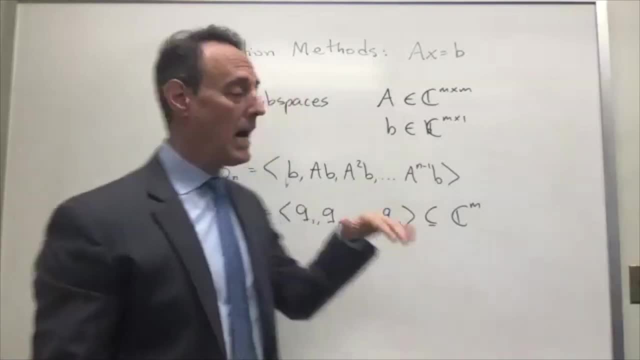 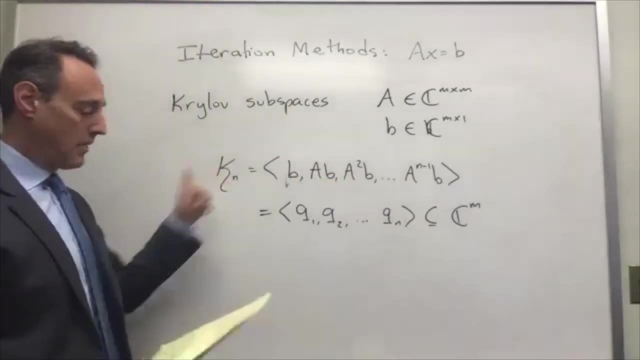 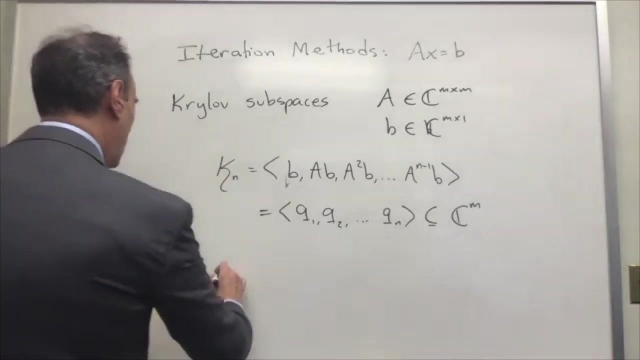 use of qr here in thinking about how do i want to take advantage of these krylov subspaces? okay, so that's the space i want to work in, and so we're going to start defining some things. in particular, what i want to do is define the krylov matrix. so this is kappa, this is k. 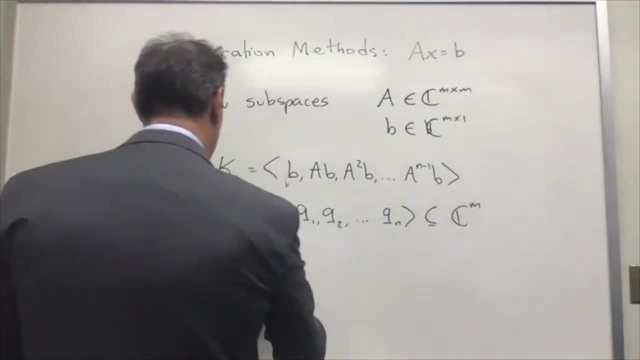 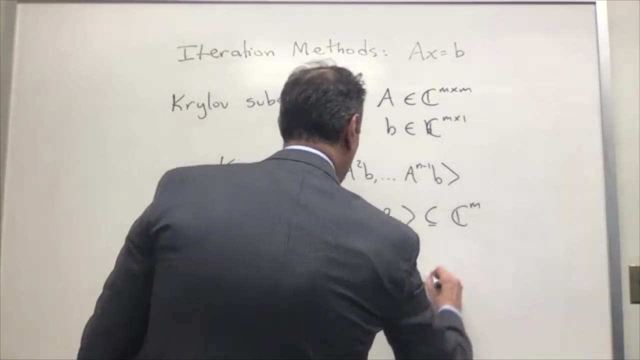 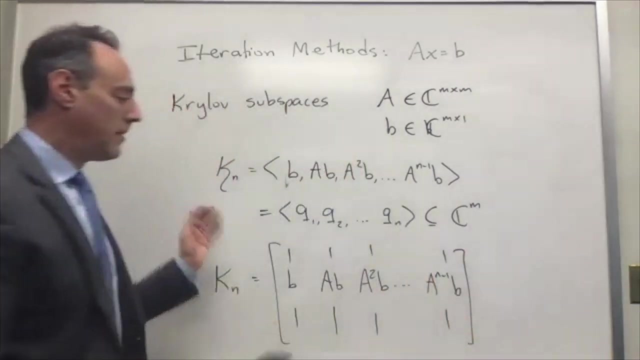 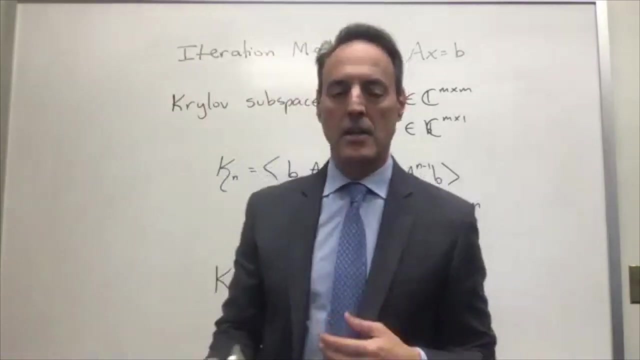 this is going to be a matrix, and the matrix i make here is b a, b a squared b, all the way to a1 is 1b. there it is. so this matrix is going to be really important for us as we start to look for solutions. 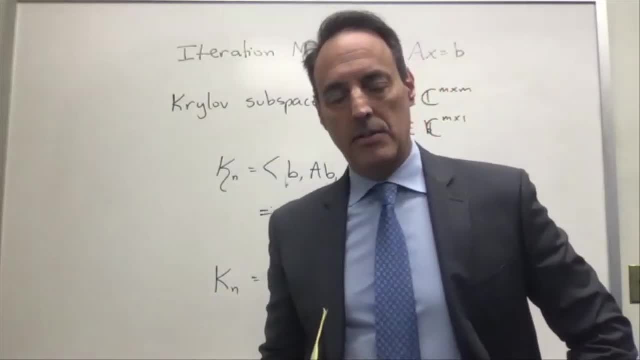 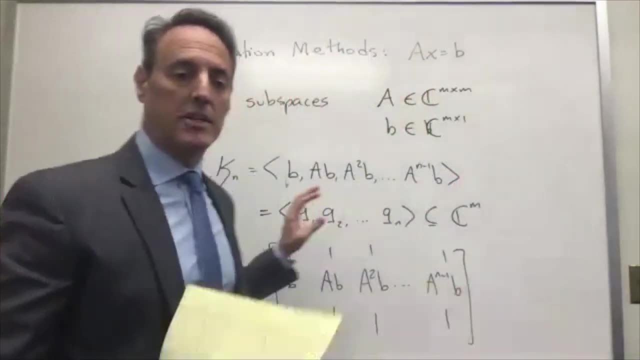 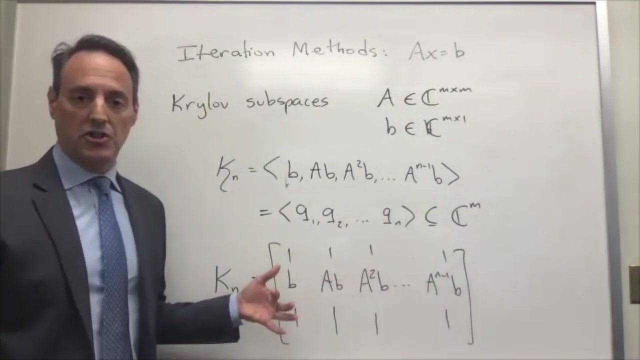 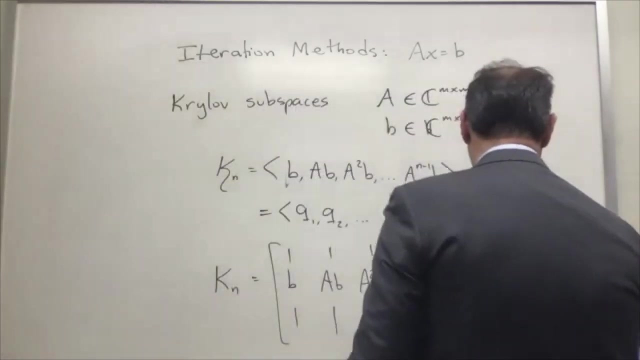 to ax equal to b, using iterative matrix techniques, and the method we're going to use is what's called this generalized method of residuals- okay, gm res- and it's going to exploit this kind of structure in this kind of space. by the way, a matrix such as this, i could in fact do a qr decomposition. so this thing here. 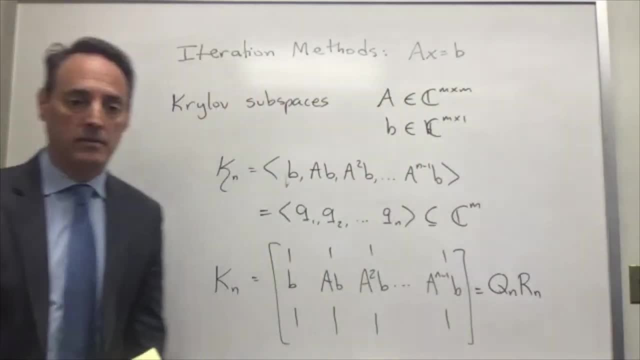 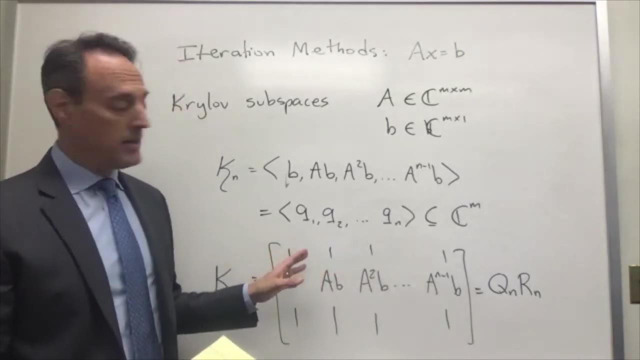 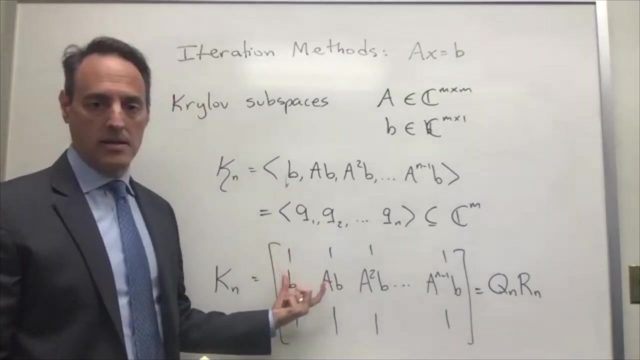 can be decomposed into q of n, r of n. okay, so notice that n is telling me how many of the columns i want. right, and remember that a is an m by m matrix and this is: this is m by n, and n is the number of iterations i do in this krylov subspace. 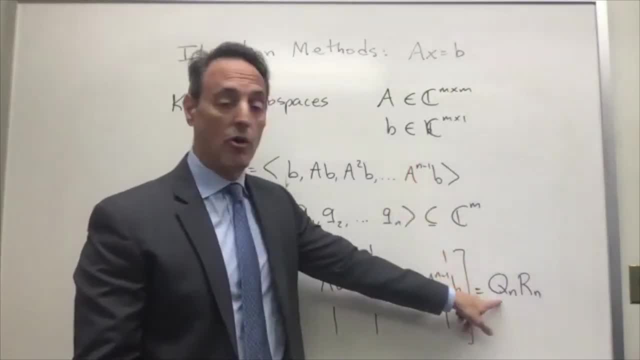 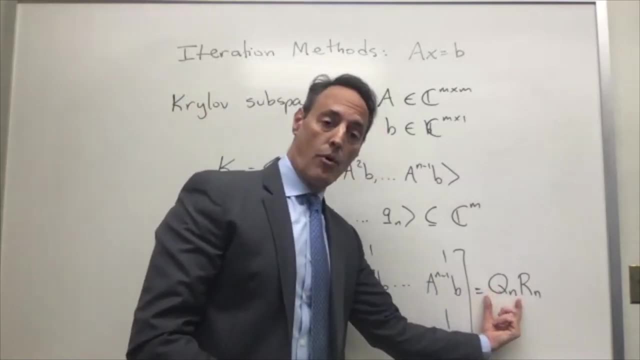 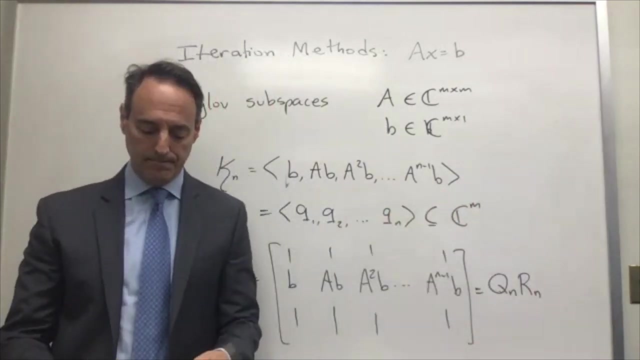 and notice that this subspace, i can in fact move me over by gram schmidt or orthogonalization to the qr, so that i get n orthonormal directions, times, some r of n, which is just the mapping from this space to that space. okay, so what this is actually telling you, what is it actually telling us? remember that. what we 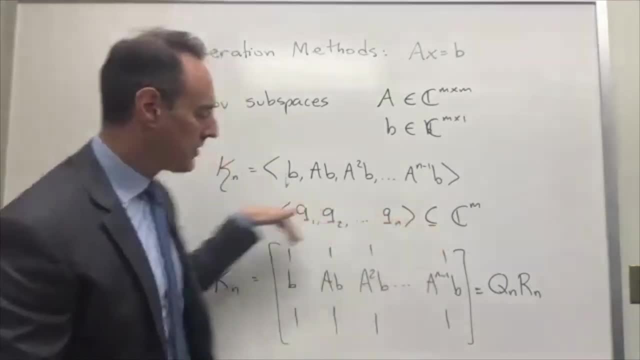 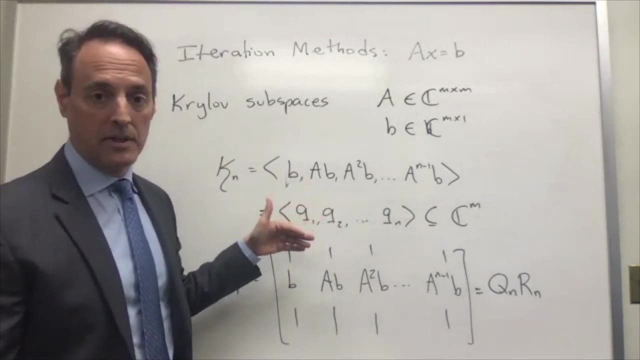 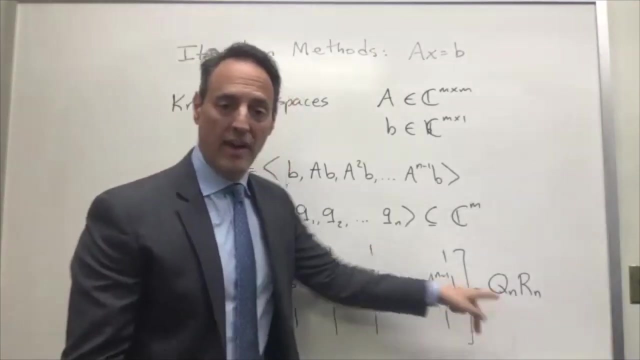 do in graham schmidt. graham schmidt says: i have all these vectors, they're not orthogonal. how do i basically make an orthonormal basis? they're not only not orthogonal, but they're not. you know, they're not normalized. so what i do, the first row of q of n is: you just take this vector b. 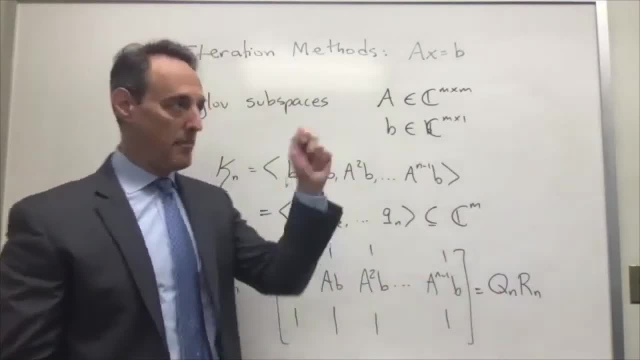 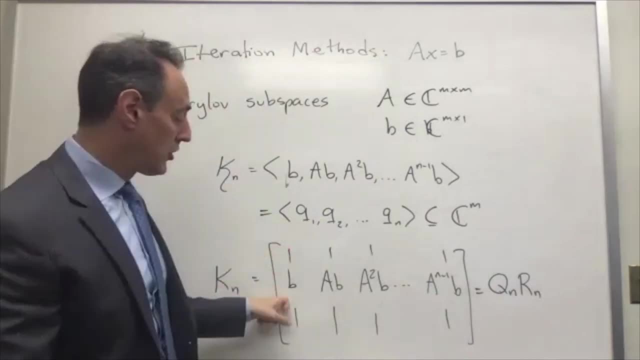 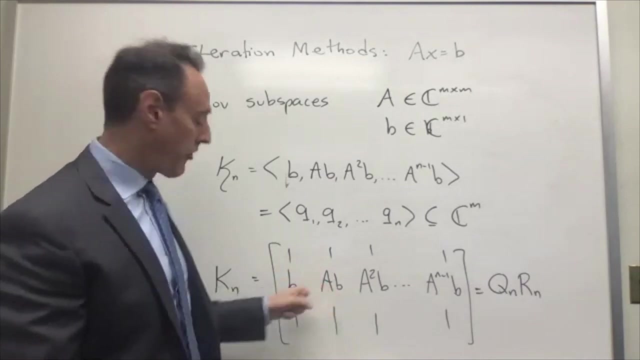 and you normalize it. that's that's how we did it before. we say, pick the vector b, normalize it. that is q1. how do i get q2, q2? i take the second vector and i project out the direction that's orthogonal. so i project out the direction that's already along b and i say what's the direction? that's? 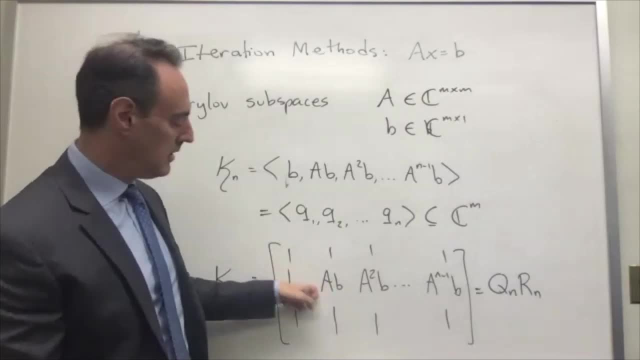 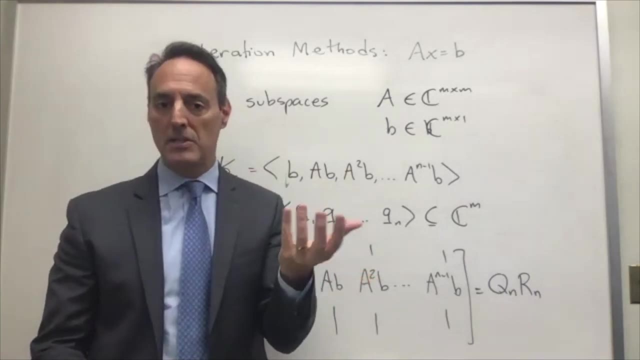 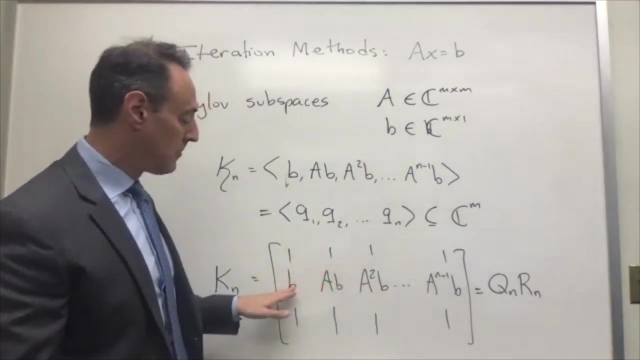 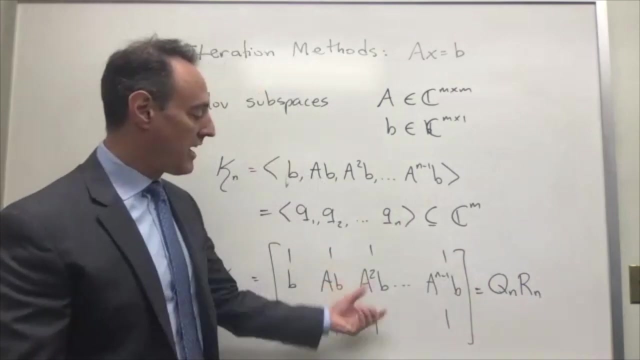 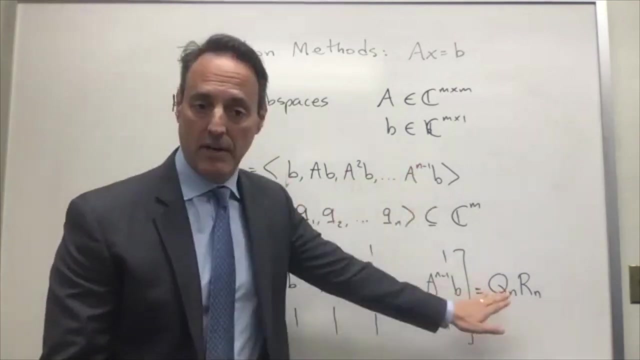 orthogonal to b to b or q1. now, and that's what remember, we worked with those orthogonal projections all this way, 하나� or all that simples win-win. so the first vector you can look at in this graph is the original, slightly misaligned vector being x, that's the second vector. you go with that. or you open up. when we say finalization, you're in the third vector. and then, Pulling on q2, let's say the third vector comes back to x-ättee. the answer: x-t, Alex's household trying colonization. that whole gram-schmidt business comes right back here to say: okay, go in my second vector, q2. i picked this vector, make it so it's orthogonal to my first vector, that's q2, normalized. then i pick the third vector. i make- this is my initial guess, but now make it orthogonal to the two previous, normalized and so forth. that's how i get this q event chemic. But enlightenment, piece 3, sub space ε, try x' forificant delas, while transformating the vector space, space, wowде. 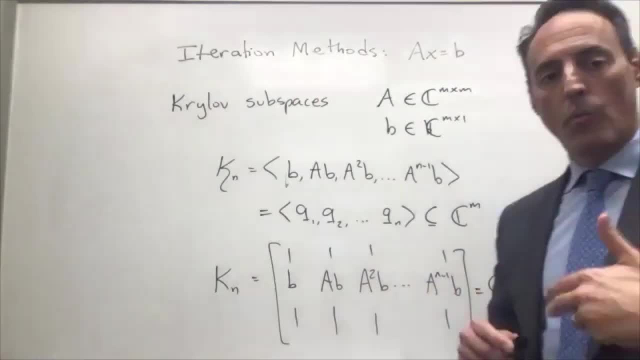 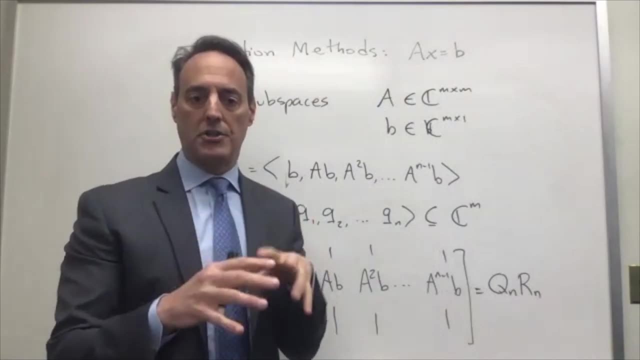 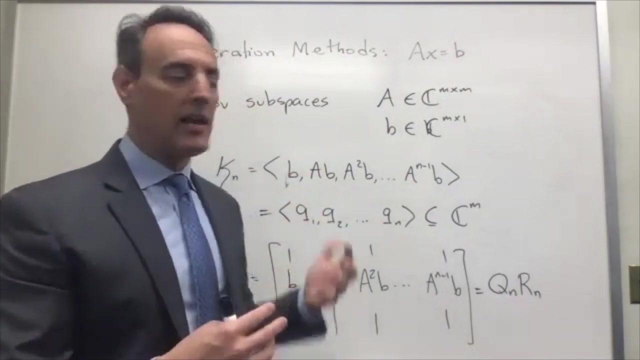 is sitting there and it turns out, what it's going to allow us to do is cry a lot of subspace. it's going to allow us to construct a recursion relationship- and i'll show you that in a little bit- which is going to allow us a very fast way to get a search algorithm for the best solution. 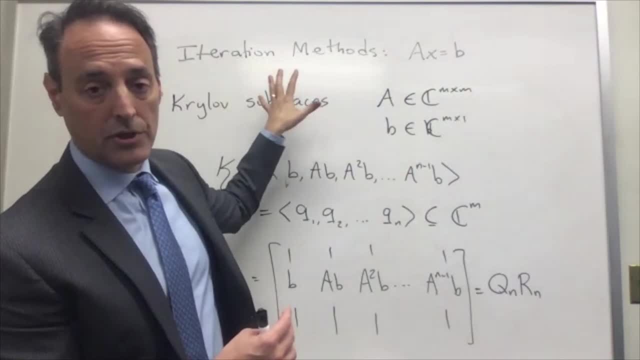 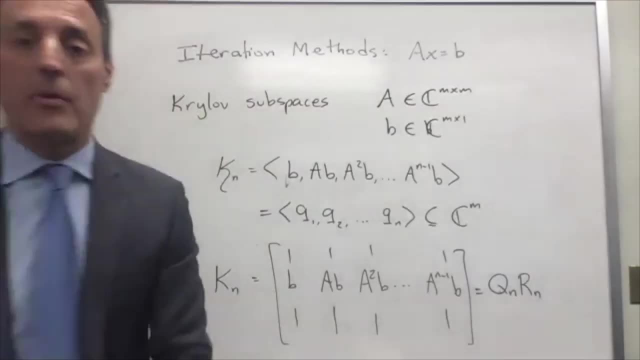 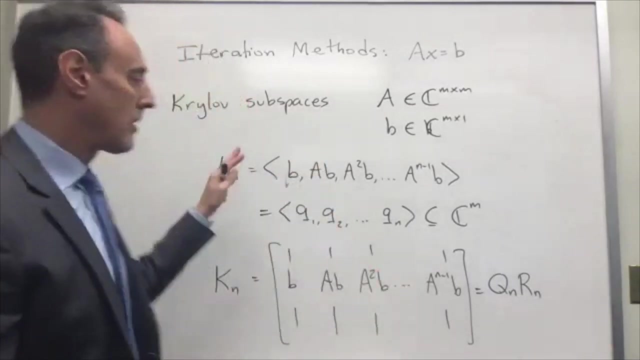 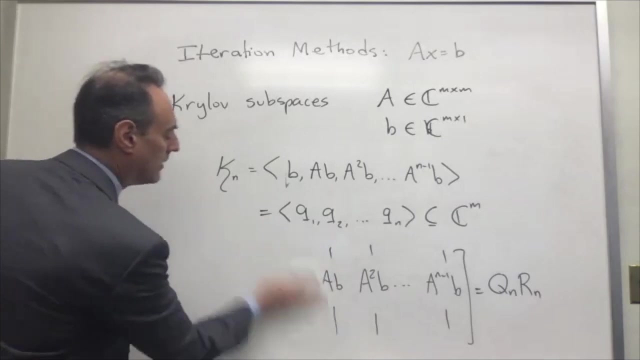 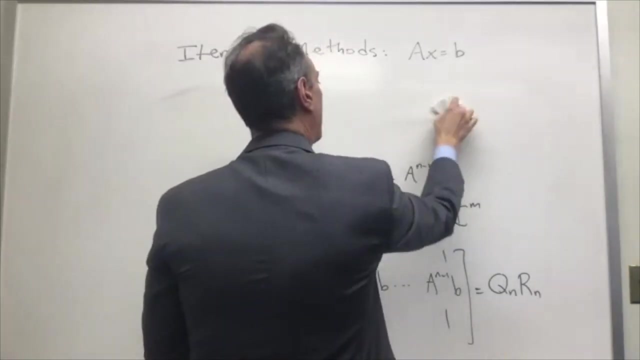 to find this ax equal to b solution through an iterative procedure. okay, so cry a lot of subspaces. you see them everywhere. anytime you're going to talk about iterations- iterative solves for ax equal to b- you're almost always going to talk about cry a lot of subspaces. they show up everywhere. okay, all right. so with that defined, let's move on. 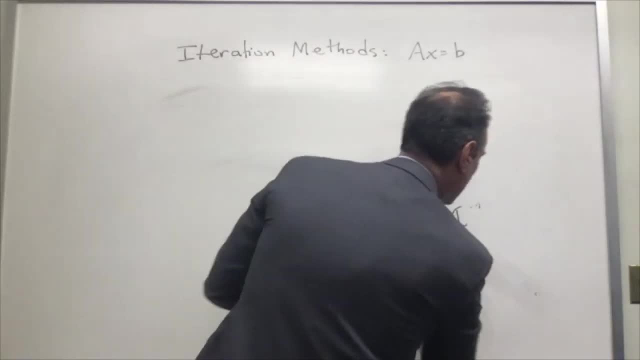 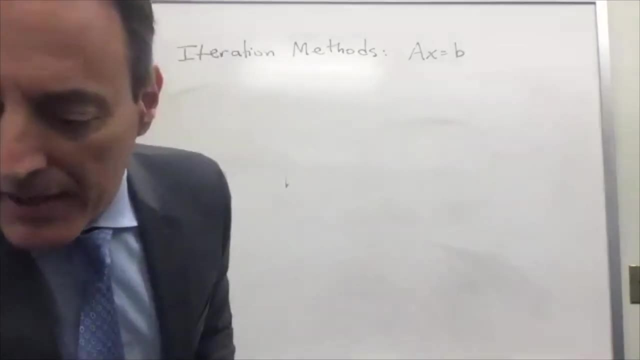 okay. so with that defined, let's move on. okay, so with that defined, let's move on. i'm not sure why my board is uh being so terrible today. i'm not sure why my board is uh being so terrible today. i'm not sure why my board is uh being so terrible today. it's pretty bad. 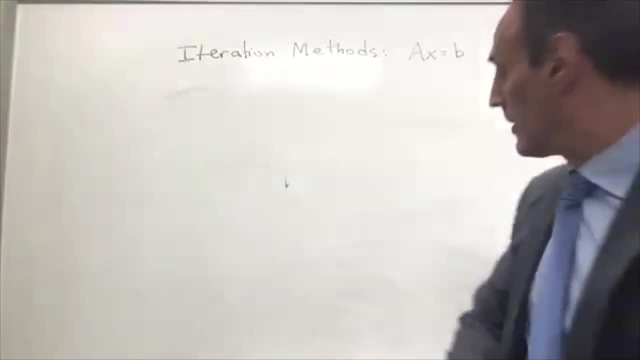 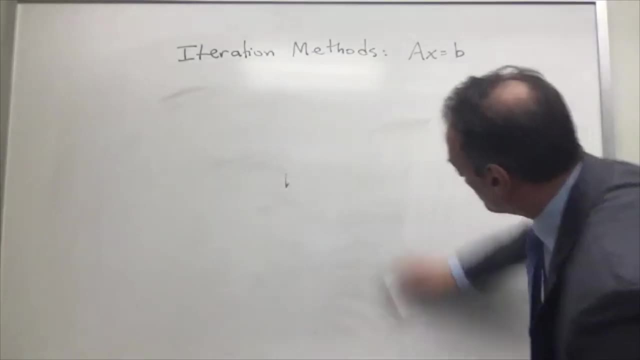 it's pretty bad. it's pretty bad. a lot of, a lot of a lot of black showing up here. i'm going to do one black showing up here. i'm going to do one black showing up here. i'm going to do one more wipe down. usually it's not this bad, especially with 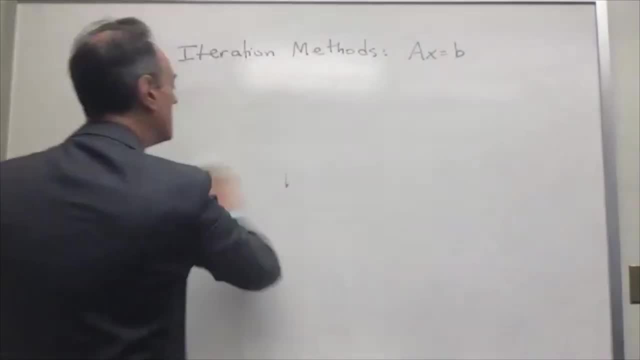 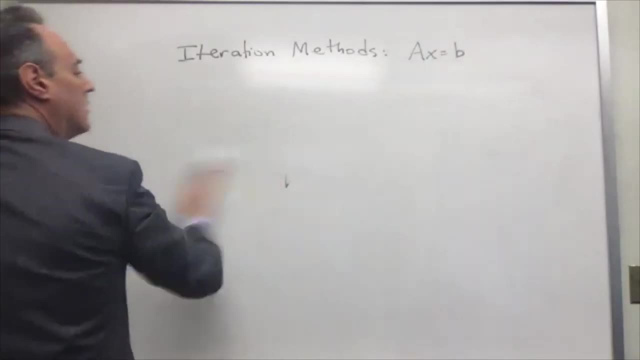 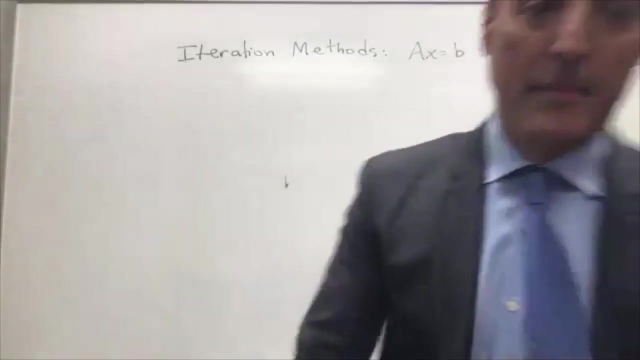 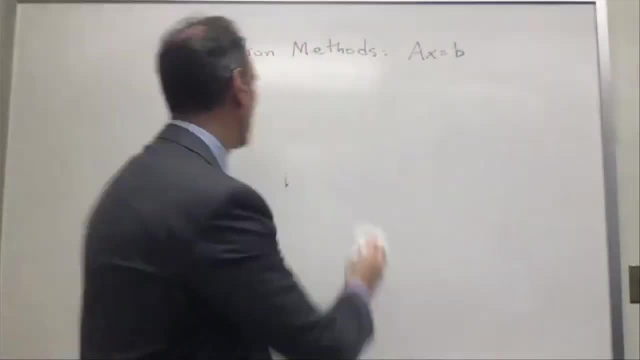 hopefully you're closer there now, okay. so now, hopefully you're closer there now, okay. so now we're going to do, we're going to do, we're going to do. let's turn our attention to this. let's turn our attention to this, let's turn our attention to this generalized method of residuals. 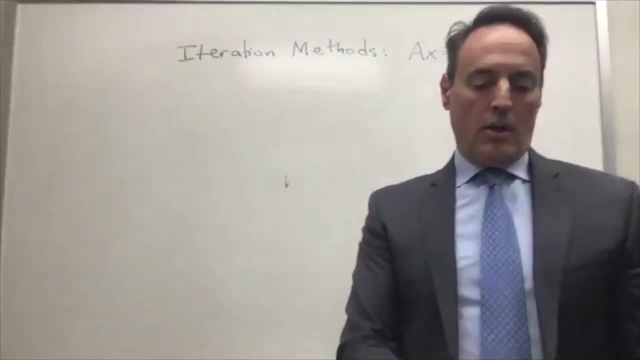 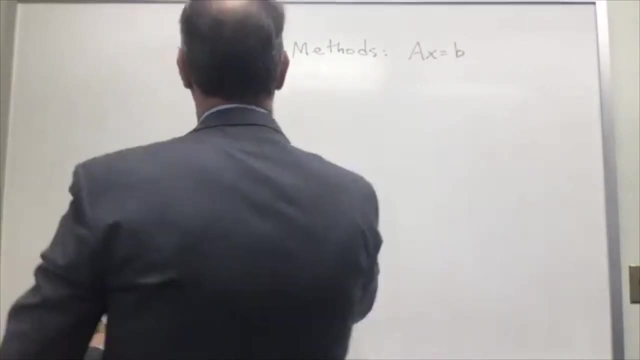 all right. what is it and how do we operate this? what is it and how do we operate this? what is it and how do we operate this? thing, thing, thing. remember what we want to do. solve x equal to b- that's almost always. solve x equal to b- that's almost always. 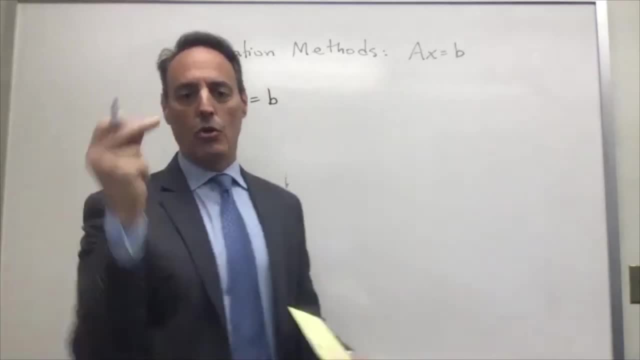 solve x equal to b. that's almost always what we want to do right. what we want to do right, what we want to do right. all these decompositions, this whole, all these decompositions, this whole, all these decompositions, this whole quarter. all we've talked about is 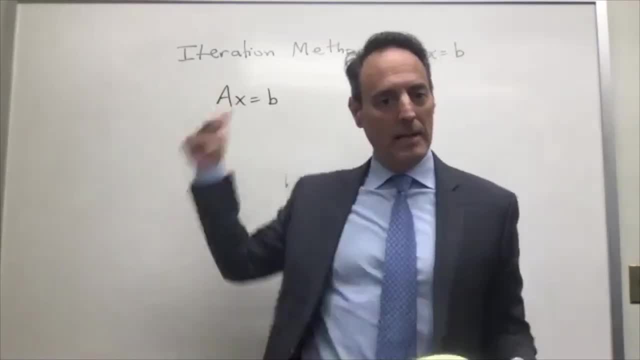 quarter. all we've talked about is quarter. all we've talked about is different algorithms, different algorithms, different algorithms, and they'll come back to solving this and they'll come back to solving this and they'll come back to solving this. right and the decompositions actually. right, and the decompositions actually. 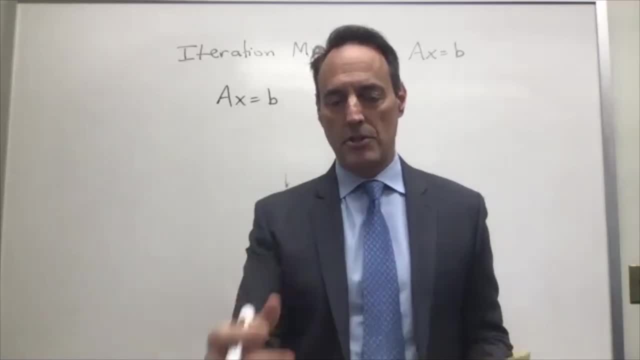 right, and the decompositions actually tell us a lot more like an eigenvector. tell us a lot more like an eigenvector. tell us a lot more like an eigenvector: decomposition, eigenvalue, decomposition, decomposition, eigenvalue, decomposition, decomposition, eigenvalue, decomposition. the svd: they tell us things about the. 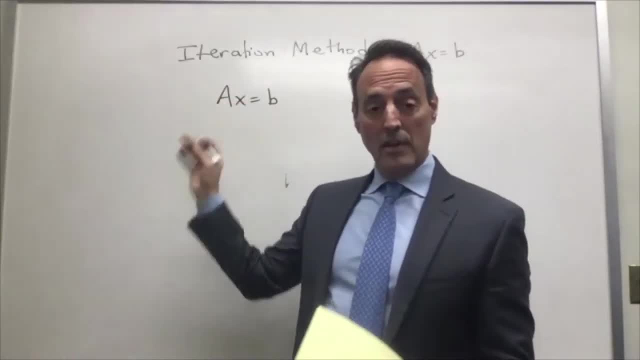 the svd. they tell us things about the the svd. they tell us things about the matrix. a matrix, a matrix, a like the spectrum, what the singular like the spectrum, what the singular like the spectrum, what the singular values are. tell us values are. tell us values are. tell us important directions, unitary matrices, that 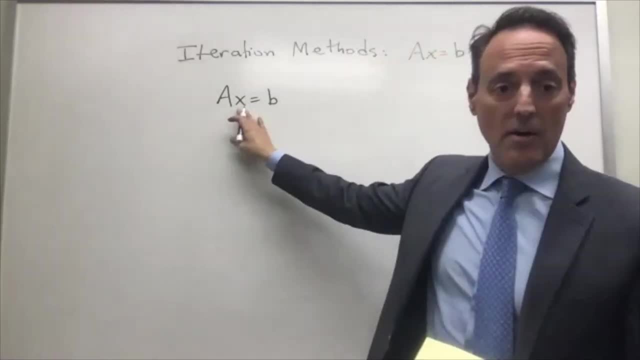 important directions, unitary matrices that important directions, unitary matrices that tell us interesting things, tell us interesting things, tell us interesting things, but really at the end of the day they, but really at the end of the day they, but really at the end of the day they all come back to. 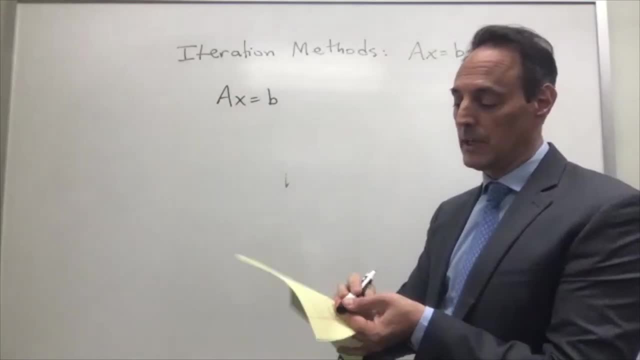 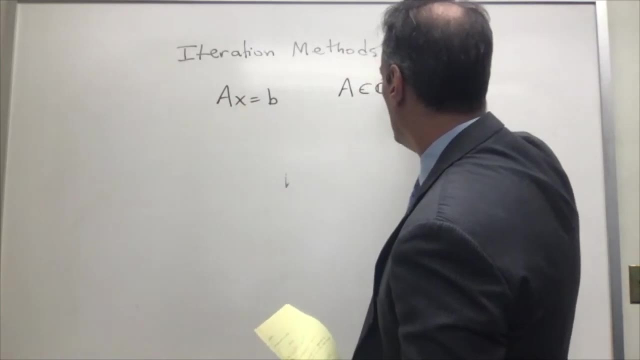 all come back to all. come back to solving x equal to b usually okay. solving x equal to b usually okay. solving x equal to b usually okay. and remember that a itself and remember that a itself and remember that a itself is some m by m and b here. 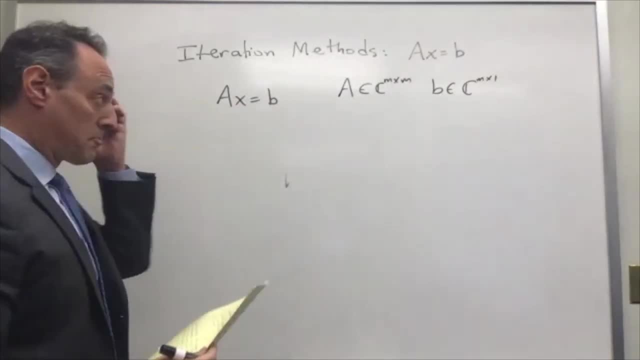 m by m and b here. m by m and b here. m by one, m by one, m by one now. let's suppose this actually has a now. let's suppose this actually has a now. let's suppose this actually has a solution. let's call it x star. 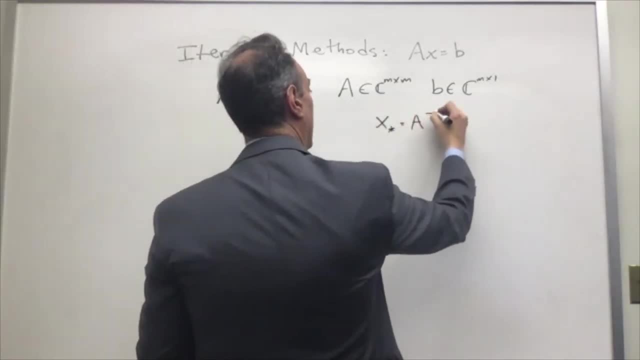 solution. let's call it x star solution. let's call it x star. so x star is equal to so x star is equal to so x star is equal to a inverse b. so there's, that's the truth: a inverse b. so there's, that's the truth. 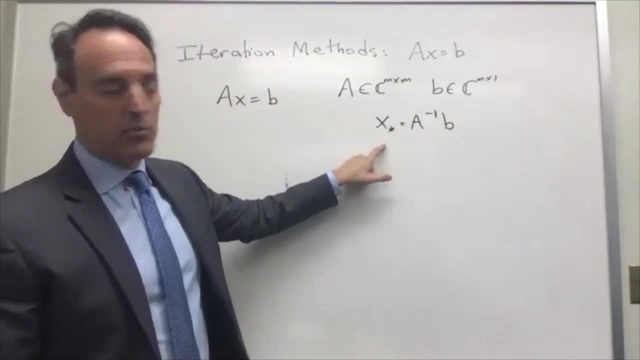 a inverse b. so there's, that's the truth. that's the ground truth. that's the ground truth. that's the ground truth. the question is: how do i compute this? the question is: how do i compute this? the question is: how do i compute this? because you wouldn't actually take the 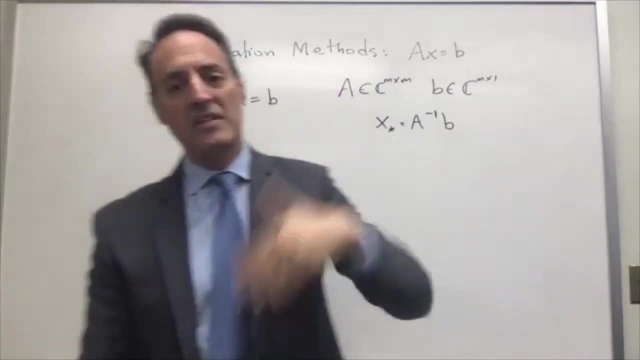 because you wouldn't actually take the, because you wouldn't actually take the inverse of this thing. it's inverse of this thing. it's inverse of this thing. it's super expensive. remember the entire goal. super expensive. remember the entire goal, super expensive. remember the entire goal. here is not to say: can i get a solution? 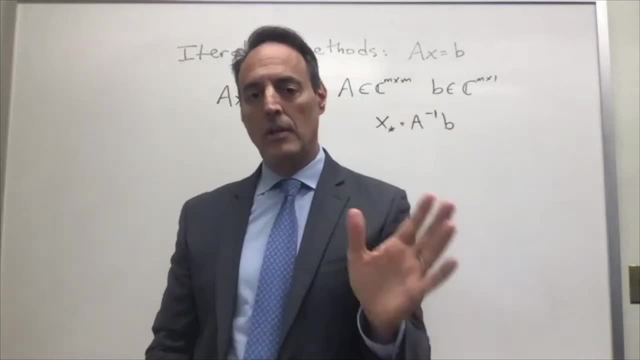 here is not to say: can i get a solution. here is not to say: can i get a solution. it's how fast can i get a solution. it's how fast can i get a solution. it's how fast can i get a solution. hopefully everybody understands that. the 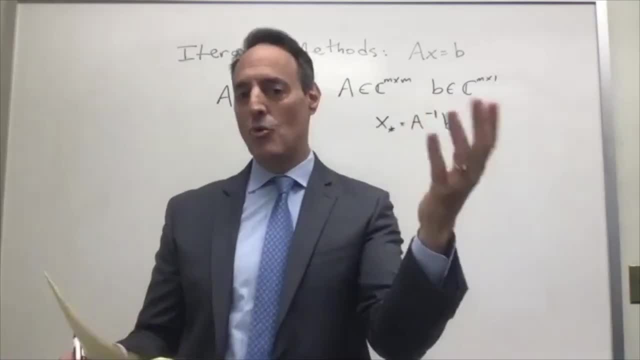 hopefully everybody understands that the hopefully everybody understands that the whole game of a lot of this linear whole game, of a lot of this linear whole game, of a lot of this linear algebra is not algebra is not, algebra is not, can i do get a solution? it's always about 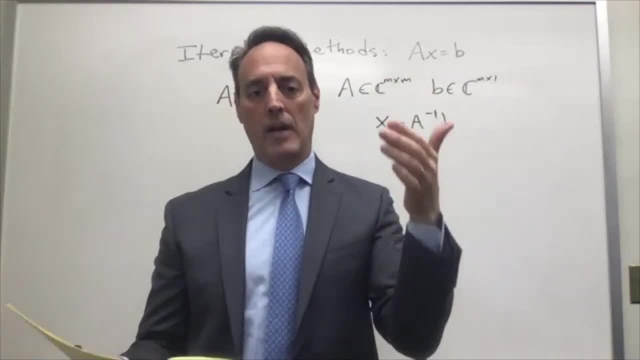 can i do get a solution. it's always about can i do get a solution. it's always about how fast can you do it. how fast can you do it, how fast can you do it right computational speed? remember i right computational speed. remember i right computational speed. remember i showed you that chart. 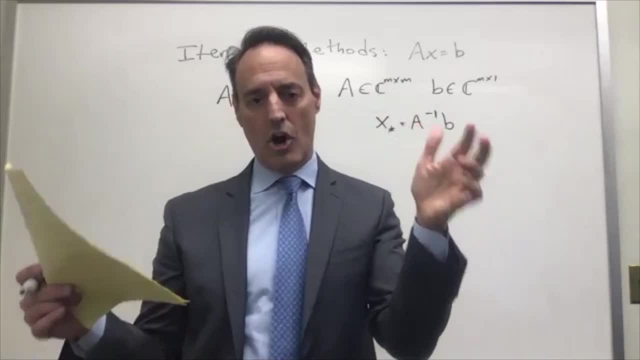 showed you that chart. showed you that chart. it took 10 to the 9 increase in. it took 10 to the 9 increase in. it took 10 to the 9 increase in hardware to get us 10 to the 3 hardware to get us 10 to the 3. 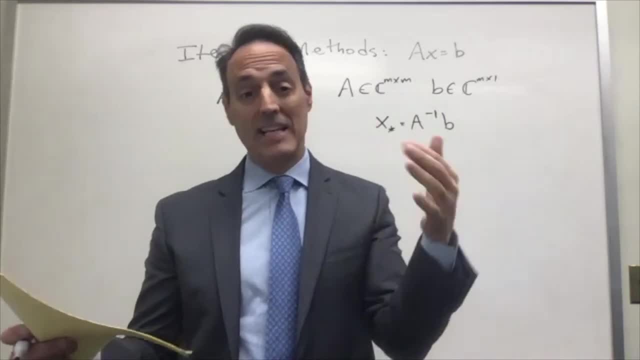 hardware to get us 10 to the 3 increase in matrix size. this is a really tough growth rate if we- this is a really tough growth rate if we- this is a really tough growth rate if we have to get, have to get, have to get 10 to the 9 every time on the hardware. 10 to the 9 every time on the hardware. 10 to the 9 every time on the hardware, just for a 10 to 3 increase. so we're just for a 10 to 3 increase. so we're just for a 10 to 3 increase. so we're trying to beat that. 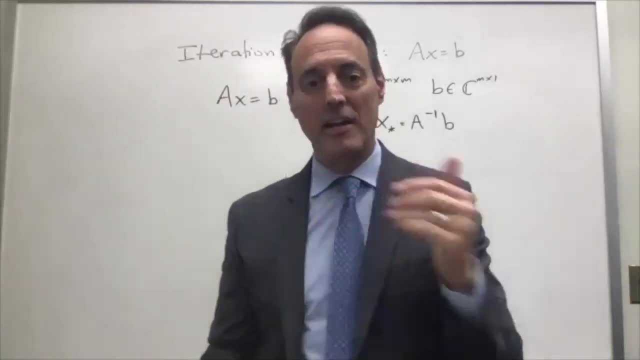 trying to beat that. trying to beat that. what we'd love to have is if you. what we'd love to have is if you. what we'd love to have is if you increased your hardware by 10 to the 9, increased your hardware by 10 to the 9. 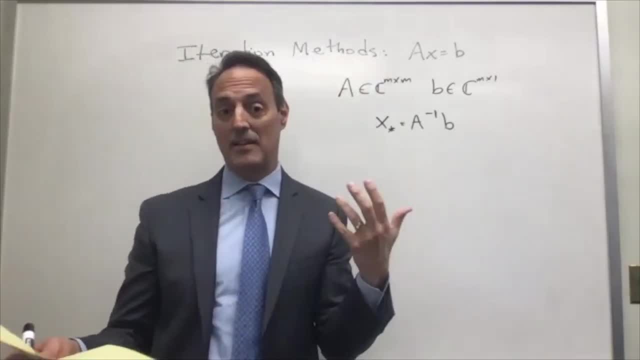 increased your hardware by 10 to the 9. your matrices went up by 10 to the 9. your matrices went up by 10 to the 9. your matrices went up by 10 to the 9. that'd be fantastic, right, but that'd be fantastic right, but. 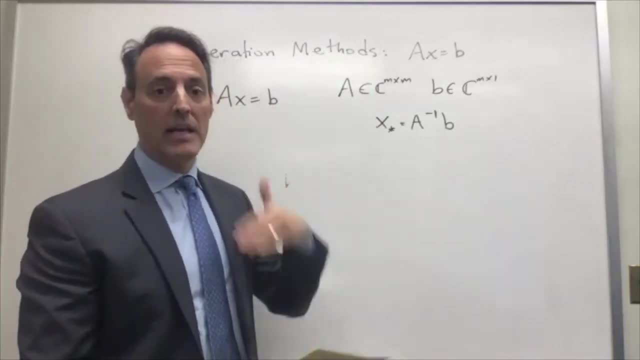 that'd be fantastic, right, but we're trying to figure out methods. that we're trying to figure out methods. that we're trying to figure out methods that just get us the solution, just get us the solution, just get us the solution and do it faster. this is about the 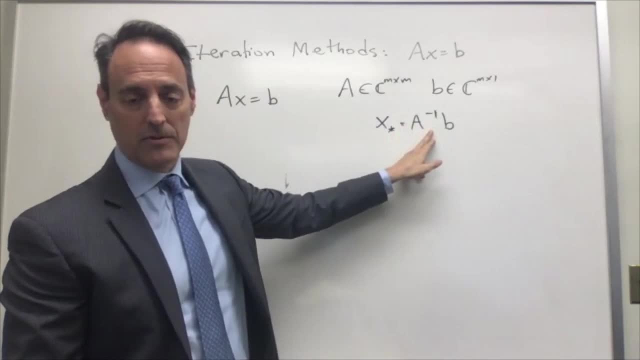 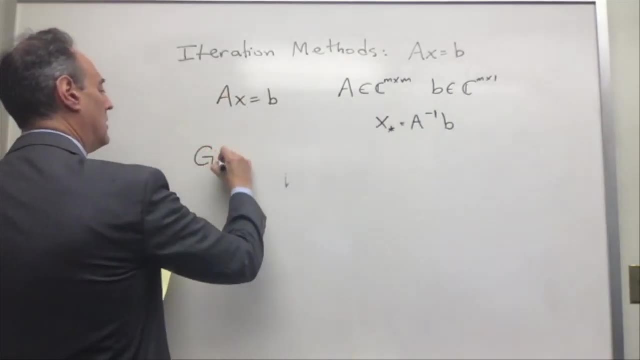 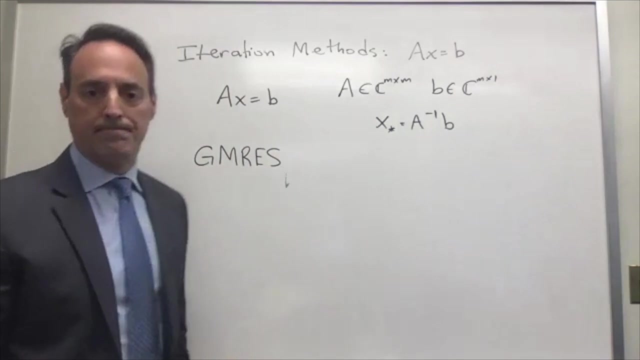 and do it faster. this is about the and do it faster. this is about the slowest way you could possibly solve slowest way you could possibly solve. slowest way you could possibly solve: generalized method of residuals. generalized method of residuals. generalized method of residuals. so what it is is a method that's pretty. 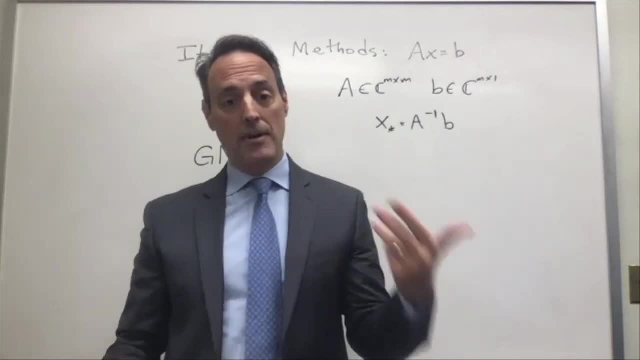 so what it is is a method that's pretty. so what it is is a method that's pretty simple, simple, simple. all we're going to do is start an. all we're going to do is start an. all we're going to do is start an iterative procedure. 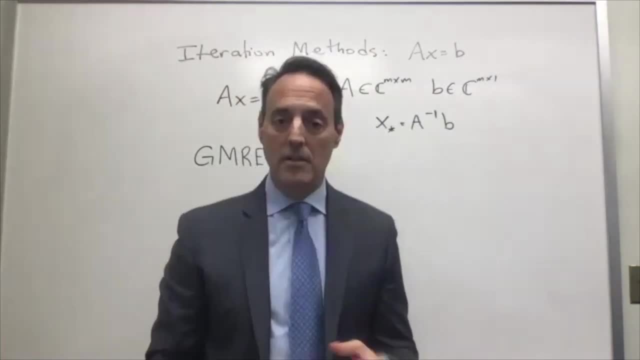 iterative procedure. iterative procedure, where every iteration we're going to, where every iteration we're going to, where every iteration we're going to minimize, minimize, minimize the residual. what do i mean by that, the residual? what do i mean by that, the residual? what do i mean by that? i want a of x equal to b. 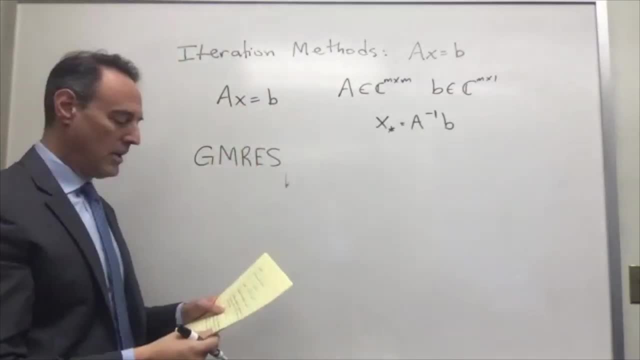 i want a of x equal to b. i want a of x equal to b, or a x minus b to be zero, or a x minus b to be zero, or a x minus b to be zero. but when i give it a guess x of n. but when i give it a guess x of n. 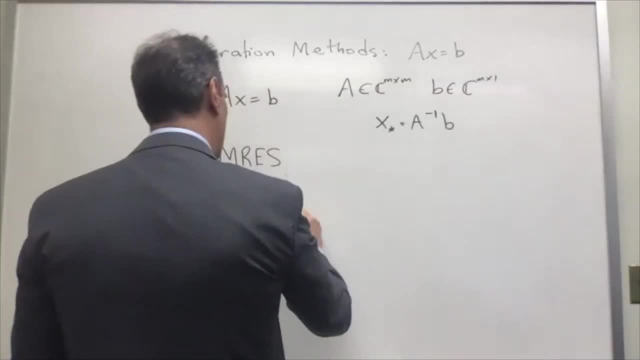 but when i give it a guess, x of n, this isn't satisfied. this isn't satisfied. this isn't satisfied. so the residual called r of n is equal. so the residual called r of n is equal. so the residual called r of n is equal to to. 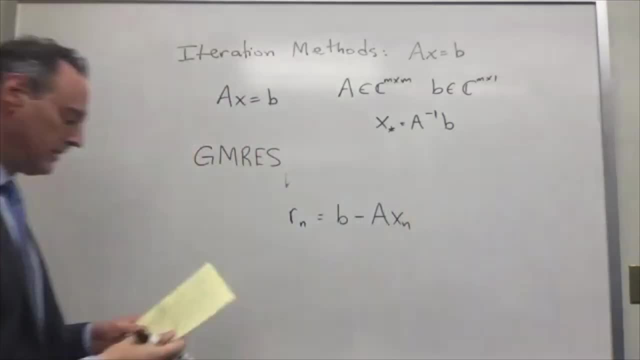 to b minus a of x of n okay. b minus a of x of n okay. b minus a of x of n okay. so there you go. this is the residual. so there you go. this is the residual. so there you go. this is the residual. if you got the right solution, if this is. 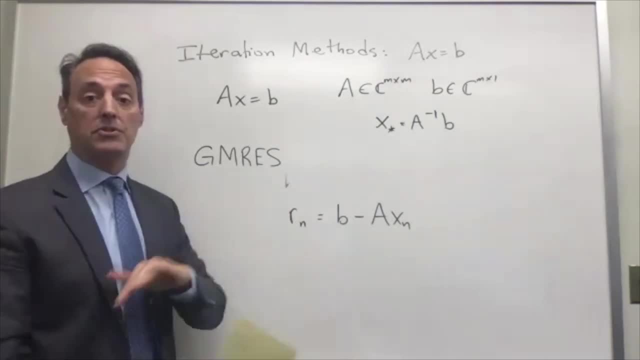 if you got the right solution. if this is if you got the right solution, if this is x star, then x minus b is zero. x star, then x minus b is zero. x star, then x minus b is zero and the residual is zero in the meantime, and the residual is zero in the meantime. 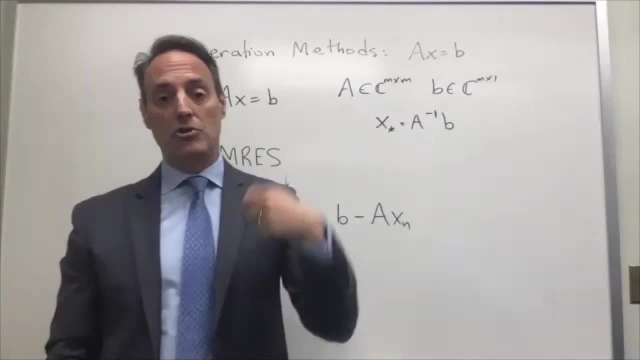 and the residual is zero. in the meantime, remember how these iteration procedures, remember how these iteration procedures. remember how these iteration procedures work. you give it a guess work. you give it a guess work. you give it a guess. you start with x0, which gets you to x1. you start with x0, which gets you to x1. you start with x0, which gets you to x1, which gets you to x2, which gets you to x2, which gets you to x2, and what you would like to do is figure, and what you would like to do is figure. 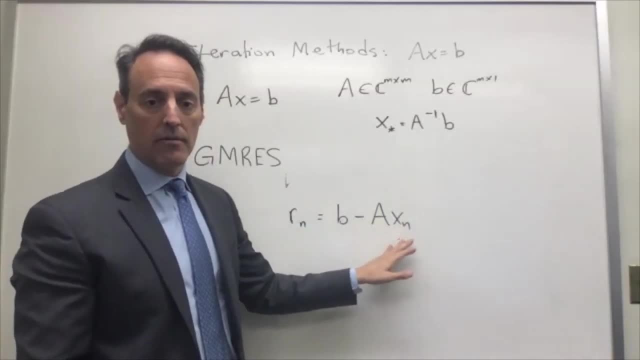 and what you would like to do is figure out. how do i out, how do i out, how do i determine an update rule for the x of n? determine an update rule for the x of n, determine an update rule for the x of n, so that this thing will iterate and 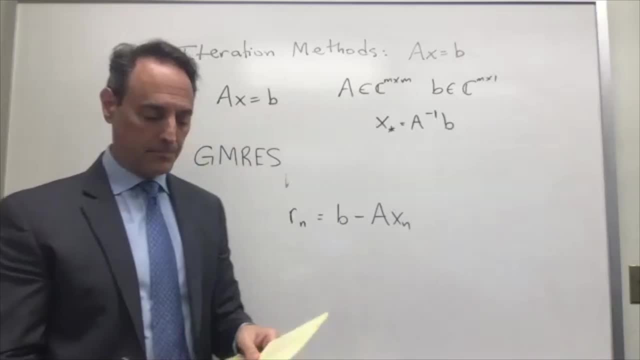 so that this thing will iterate and so that this thing will iterate and converge to the solution, converge to the solution, converge to the solution: x, star okay, x, star, okay, x, star, okay. so the entire idea here is, by the way. so the entire idea here is, by the way. 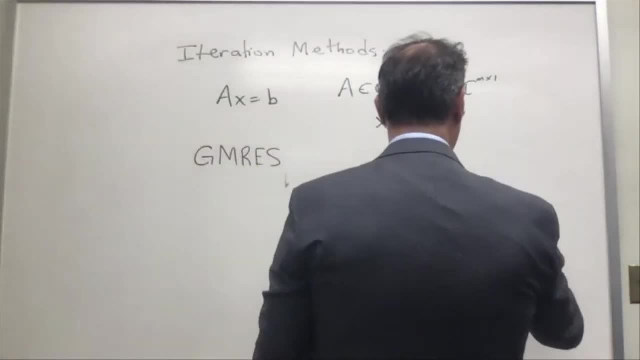 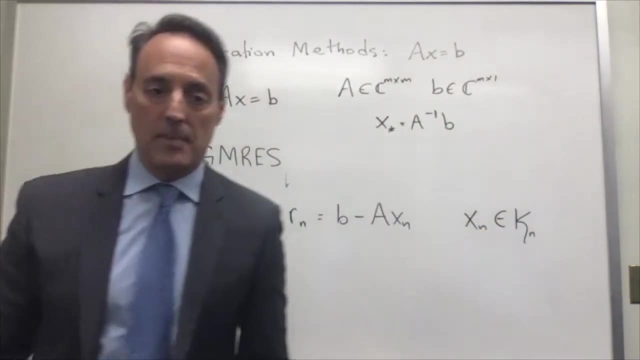 so the entire idea here is, by the way, the x of n, the x of n, the x of n is going to live, is going to live, is going to live in the space and the krylov subspace, and the krylov subspace and the krylov subspace. okay, so that's, i get to pick a vector. okay, so that's, i get to pick a vector. okay, so that's, i get to pick a vector out of here, out of here, out of here, out of this krylov subspace. so this is out of this krylov subspace, so this is. 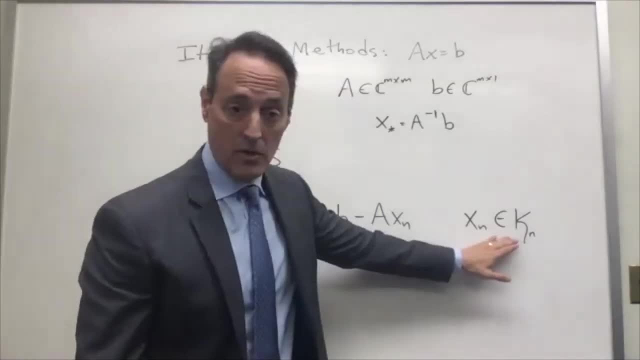 out of this krylov subspace. so this is where the krylov subspace comes in, where the krylov subspace comes in, where the krylov subspace comes in. this is my subspace for representing each. this is my subspace for representing each. 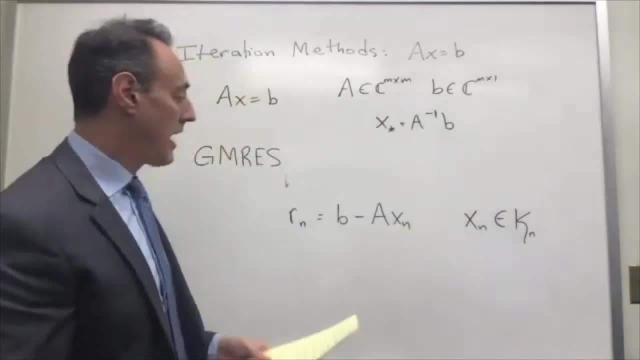 this is my subspace for representing each pick, pick, pick, and what i want to do is basically put, and what i want to do is basically put, and what i want to do is basically put each x of n, each x of n, each x of n, and i want to pick x of n. 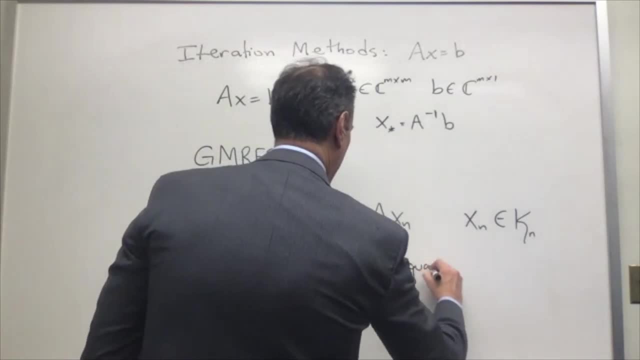 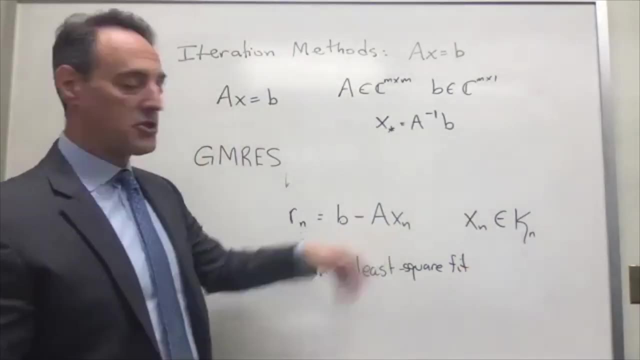 and i want to pick x of n and i want to pick x of n through a least square fit. okay, least square fit and remember i'm going to least square fit and remember i'm going to least square fit. and remember i'm going to start off with x. 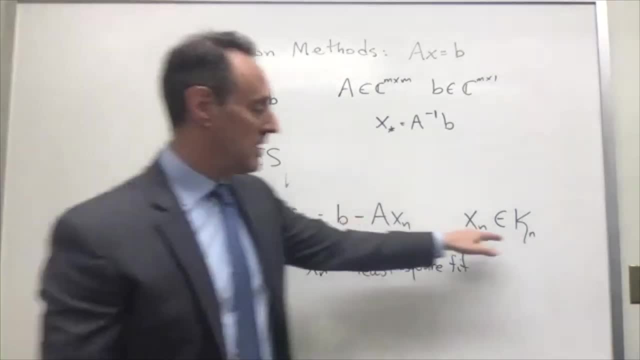 start off with x, start off with x- zero, and i'm going to get x1, so in zero, and i'm going to get x1, so in zero, and i'm going to get x1. so in other words, other words, other words, it's going to have to live in the first. 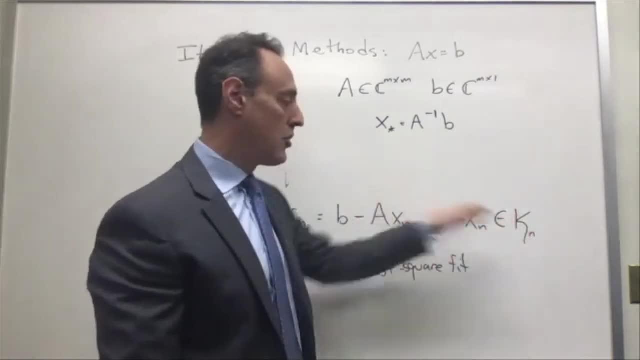 it's going to have to live in the first. it's going to have to live in the first krylov subspace, krylov subspace, krylov subspace, k1, and then when i go to two, it can live- k1, and then when i go to two, it can live. 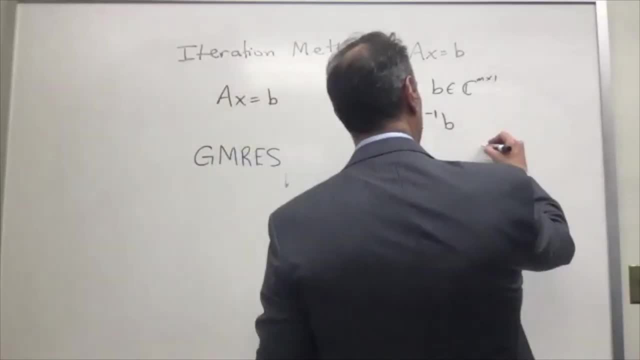 k1 and then when i go to two, it can live in the space, in the space, in the space. remember the krylov subspace. look like. remember the krylov subspace. look like. remember the krylov subspace. look like it was spanned by b. 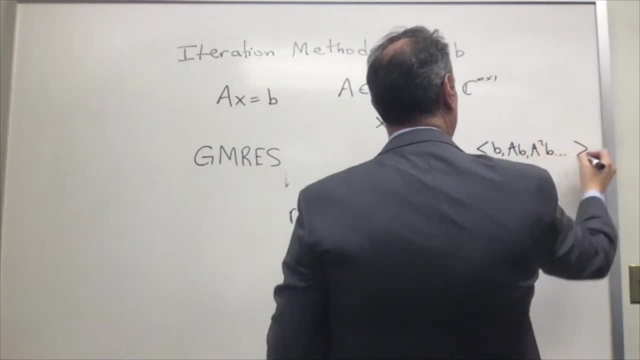 it was spanned by b. it was spanned by b a, b a squared b a, b a squared b a, b a squared b, so forth. so i am constrained. this x, so forth, so i am constrained, this x, so forth. so i am constrained, this x event has to live. 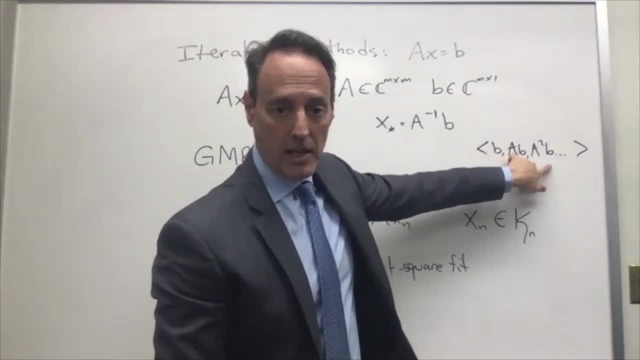 event has to live. event has to live. each time i iterate, i get to broaden my. each time i iterate, i get to broaden my. each time i iterate i get to broaden my krylov subspace, krylov subspace, krylov subspace. so first it only can live in here, then in. 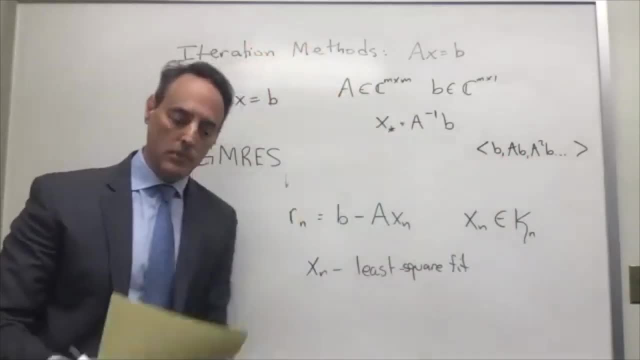 so first it only can live in here, then in. so first it only can live in here, then in here, then in here, here, then in here, here, then in here. okay, so that's the idea behind this. okay, so that's the idea behind this. okay, so that's the idea behind this. so this is going to be some 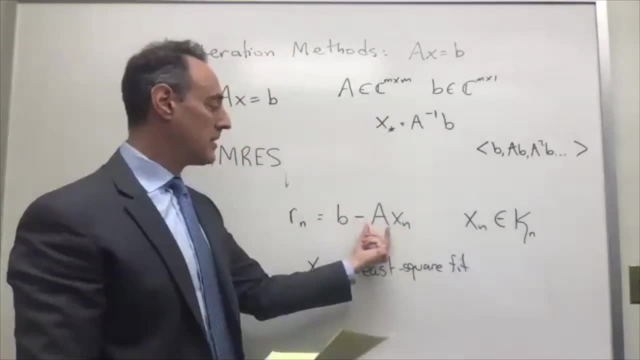 so this is going to be some, so this is going to be some n-dimensional space trying to represent n-dimensional space. trying to represent n-dimensional space, trying to represent this thing is m by m, but this thing here, this thing is m by m, but this thing here. 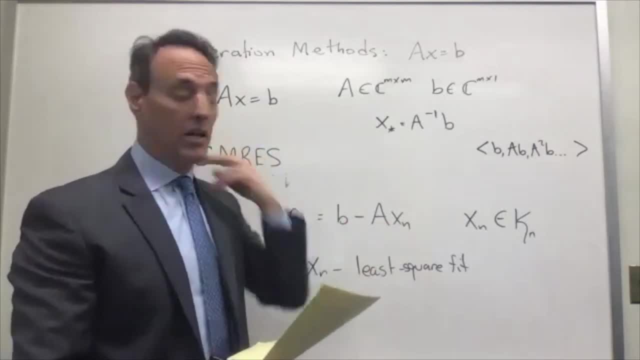 this thing is m by m, but this thing here is a is a is a small space, you know it's. it only spans small space, you know it's. it only spans small space, you know it's. it only spans an n-dimensional space of that, an n-dimensional space of that. 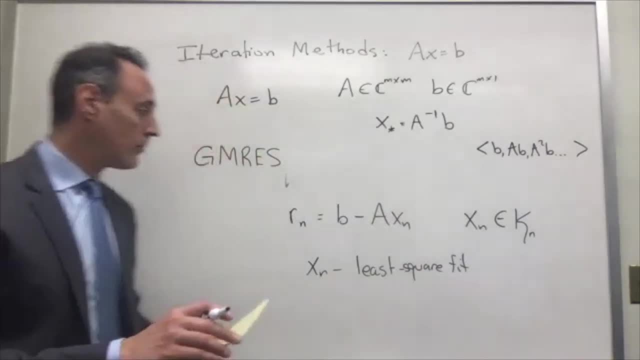 an n-dimensional space of that, out of that m-dimensional space, out of that m-dimensional space, out of that m-dimensional space. so that's the main idea, that's it so. so, that's the main idea, that's it so. so, that's the main idea, that's it. so then the question really comes down to. 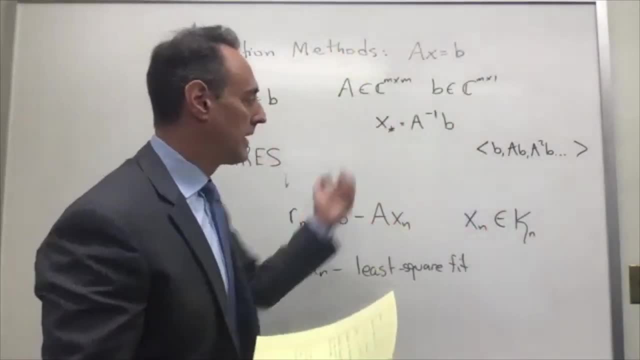 then the question really comes down to. then the question really comes down to is: is: is all right so, given that this vector x of all right, so, given that this vector x of all right so, given that this vector x of m lives in that krylov subspace. 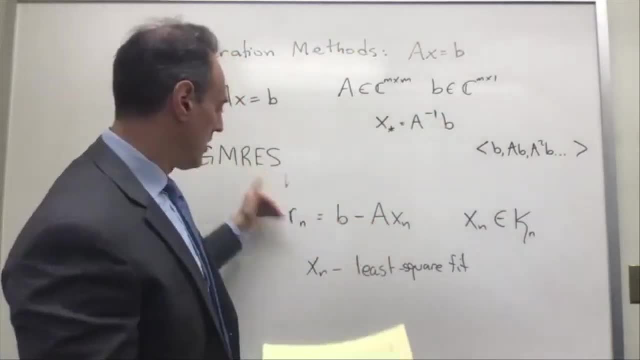 m lives in that krylov subspace. m lives in that krylov subspace. how do i determine the x of n at each? how do i determine the x of n at each? how do i determine the x of n at each iteration, iteration, iteration that minimizes this at each step? 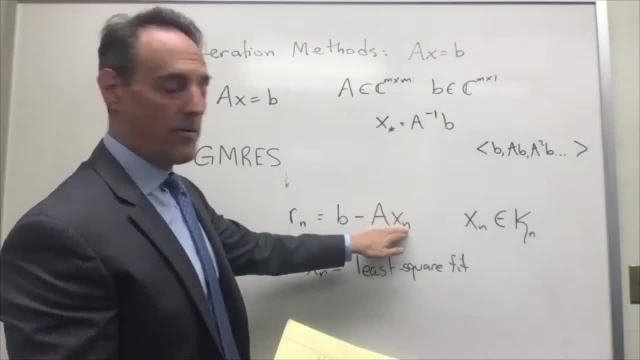 that minimizes this at each step. that minimizes this at each step. and the idea is that, and the idea is that, and the idea is that if i start off with an x of zero, i get a. if i start off with an x of zero, i get a. 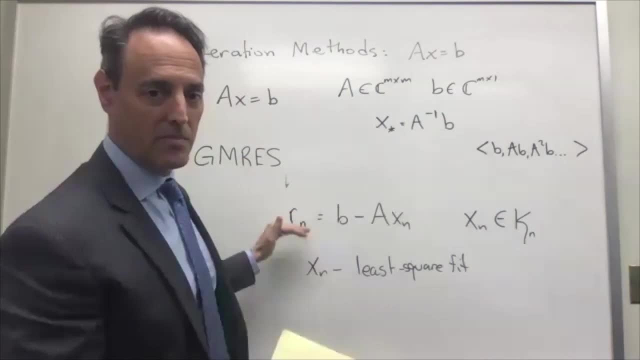 if i start off with an x of zero, i get a number, number, number, and i go to x1- x2 and this should get, and i go to x1- x2 and this should get, and i go to x1- x2 and this should get smaller and smaller and smaller in the 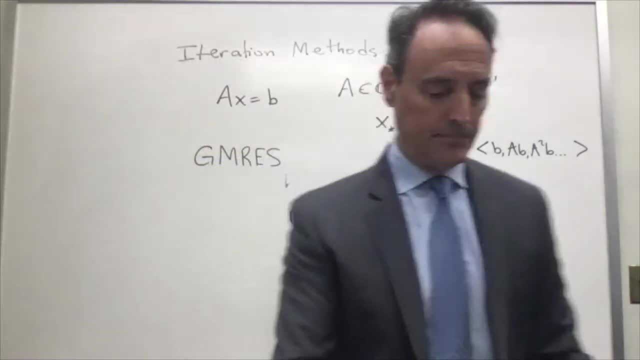 and i go to x1, x2 and this should get smaller and smaller in the residuals to just start to decrease residuals, to just start to decrease residuals, to just start to decrease, and then you're going to stop this when, and then you're going to stop this when. 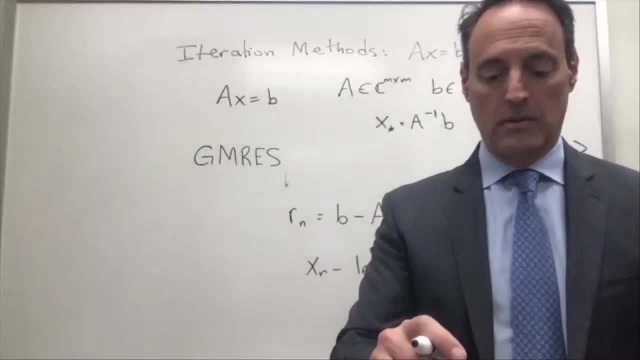 and then you're going to stop this when you get, you get, you get close enough to the real solution. okay, close enough to the real solution, okay, close enough to the real solution, okay. so that's the main idea, so that's the main idea, so that's the main idea behind gm res. 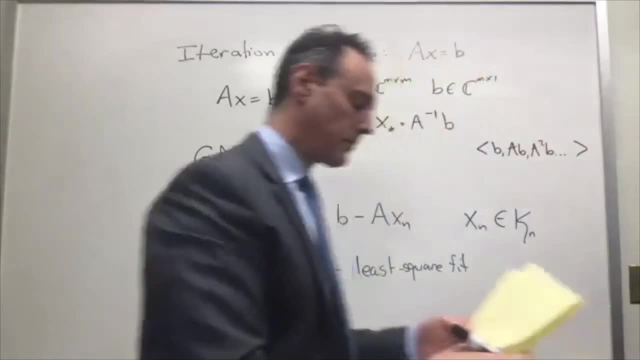 behind gm res, behind gm res. all right, let me get the next paper here. all right, let me get the next paper here. all right, let me get the next paper here. all right, so let's start setting this up. all right, so let's start setting this up. 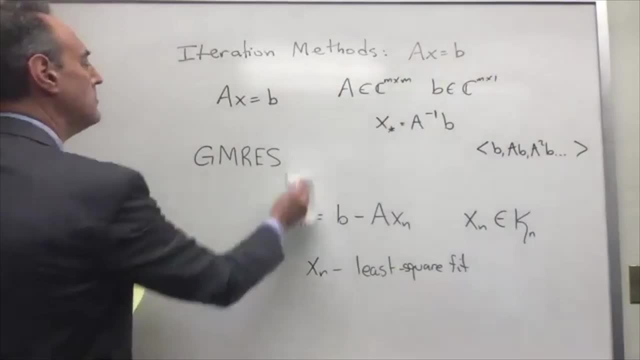 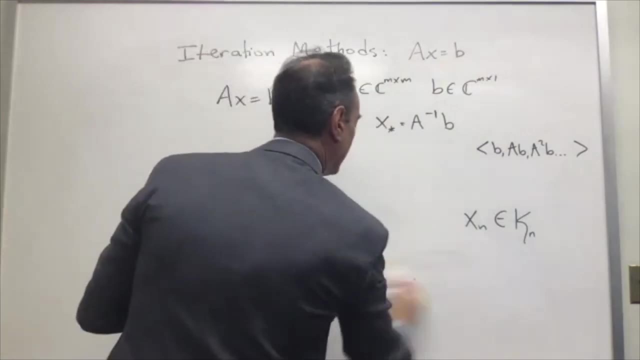 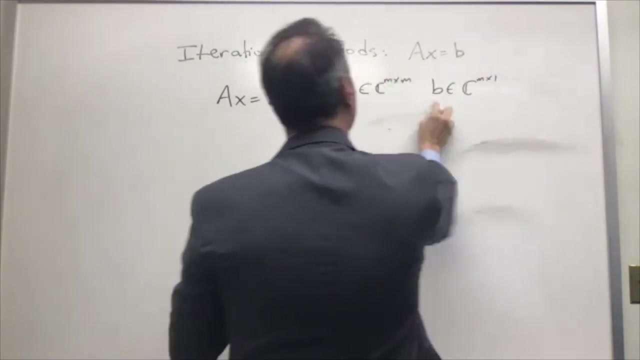 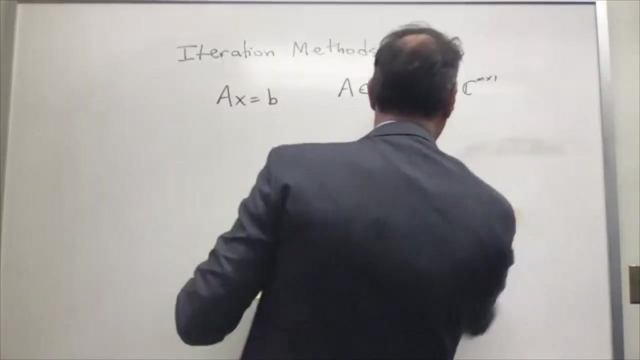 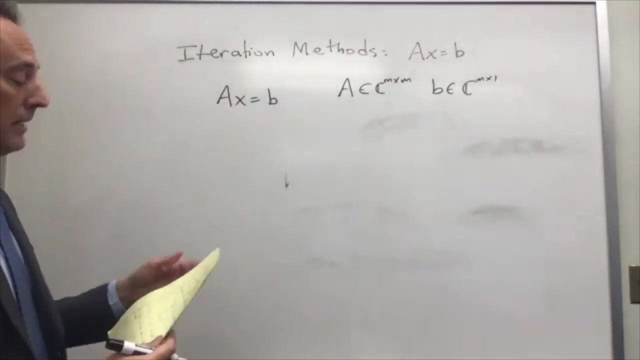 all right. so let's start setting this up, so we can solve, so we can solve, so we can solve. oh man, this is a bad day for board. okay, let's leave it like that, all right. okay, let's leave it like that, all right. okay, let's leave it like that, all right. so we're going to solve: x equals b. 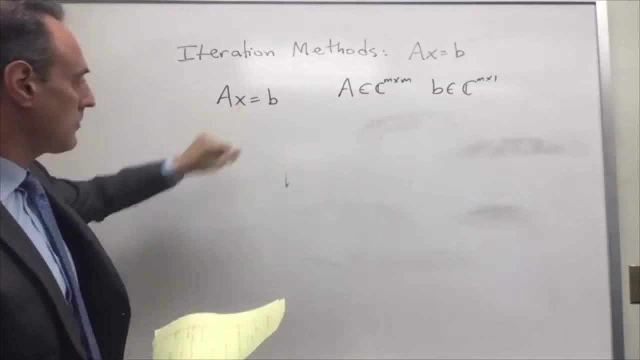 so we're going to solve x equals b, so we're going to solve x equals b. and remember i'm trying to play around and remember i'm trying to play around and remember i'm trying to play around with this x, with this x, with this x, and so 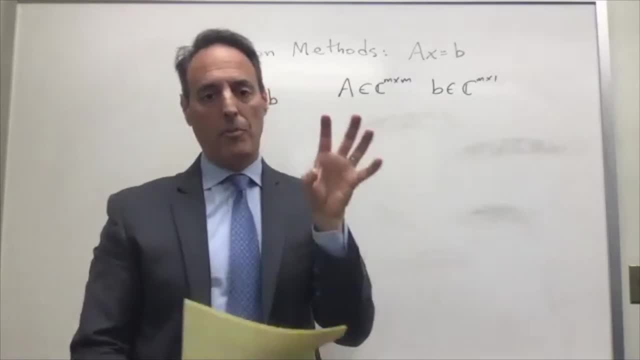 and so, and so i want to ask the question: what happens? i want to ask the question: what happens? i want to ask the question: what happens when i, when i, when i multiply that matrix a, multiply that matrix a. multiply that matrix a against the krylov matrix? 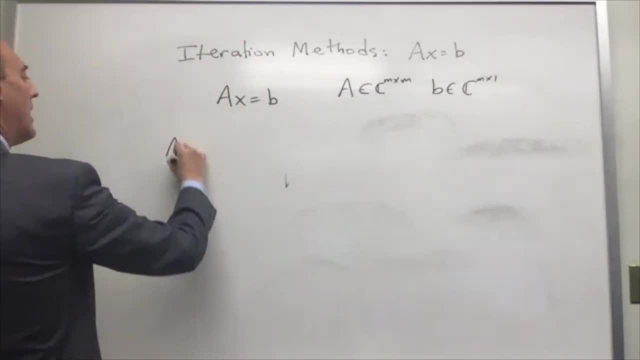 against the krylov matrix, against the krylov matrix, okay, the krylov matrix. so in other words, okay, the krylov matrix. so in other words, okay, the krylov matrix. so in other words, a acting on a acting on a acting on k of n. remember, k of n is b. 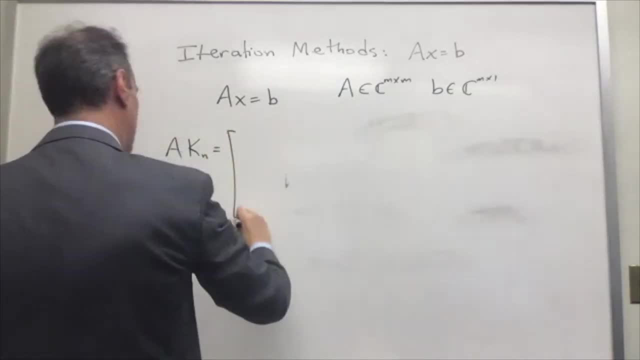 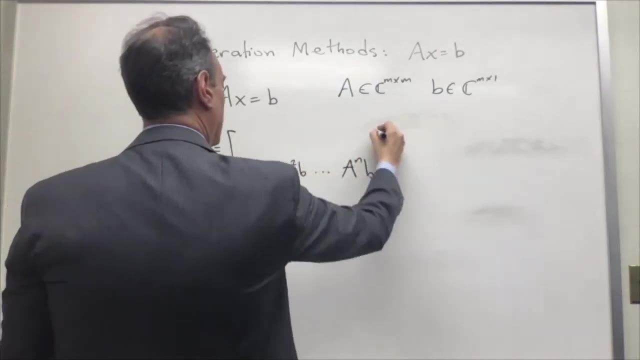 k of n. remember k of n is b. k of n. remember k of n is b a b a squared b. so this here becomes: a b a squared b. a to the n b. a b a squared b. a to the n. b a squared b a squared b. a to the n b. 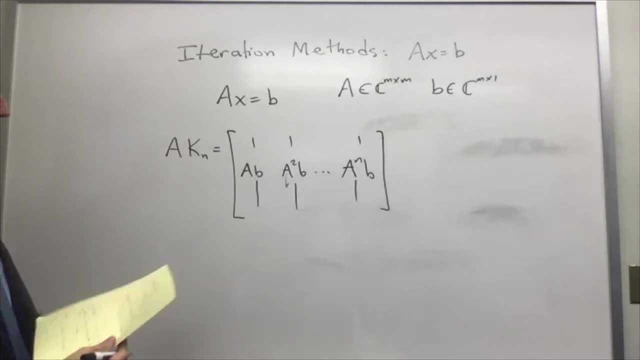 okay, okay, okay, and so really, what i want to do is think, and so, really, what i want to do is think, and so really, what i want to do is think about like well, my vector x, about like well, my vector x, about like well, my vector x is going to live in this krylov subspace. 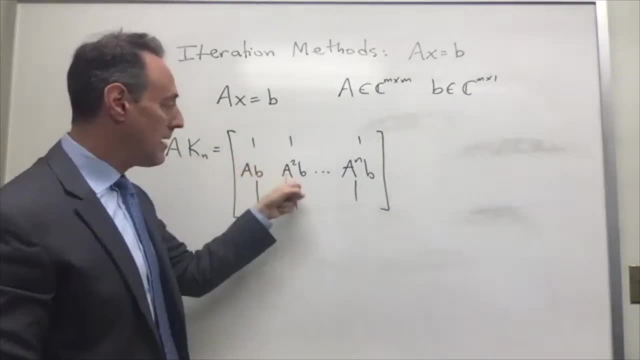 is going to live in this krylov subspace, is going to live in this krylov subspace, which is a linear combination of those, which is a linear combination of those, which is a linear combination of those vectors b, vectors b, vectors b, a b, all the way through here, and so one. 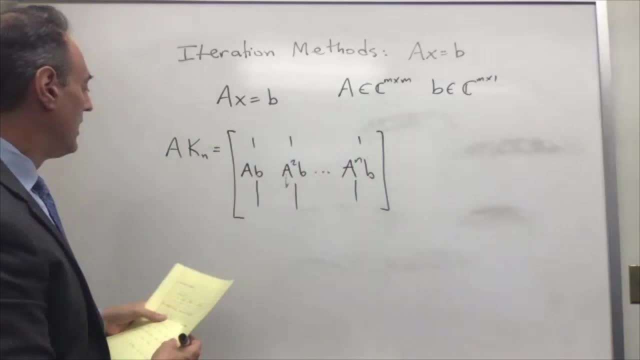 a b all the way through here, and so one a b all the way through here, and so one way to think about this is way to think about this is way to think about this is what i'd really like to do, then, is to. what i'd really like to do, then, is to. 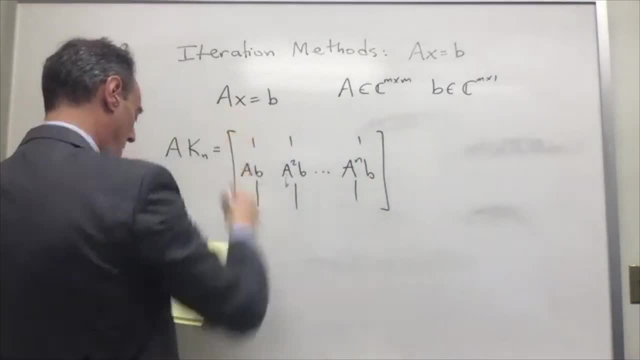 what i'd really like to do, then, is to minimize, minimize, minimize, in other words, the vector x. one way to, in other words, the vector x. one way to, in other words, the vector x. one way to think about it is, think about it is, think about it. is x of n is going to be a linear. 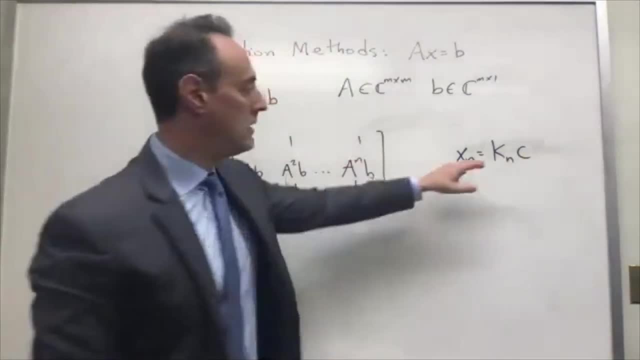 x of n is going to be a linear. x of n is going to be a linear combination. i'm going to live in this subspace k of n. i'm going to live in this subspace k of n. i'm going to live in this subspace k of n. so x of n is going to be a linear. 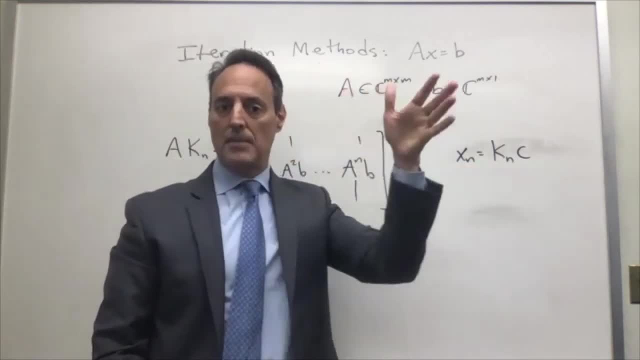 so x of n is going to be a linear, so x of n is going to be a linear combination, combination: combination of those krylov subspace vectors, which of those krylov subspace vectors, which of those krylov subspace vectors which are. 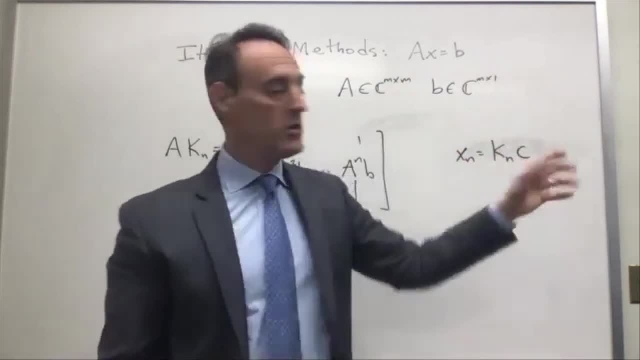 are are: how much of each column i need. how much of each column i need. how much of each column i need to represent x of n. to represent x of n. to represent x of n. the question is: how do i pick c? i want to. the question is: how do i pick c? i want to. 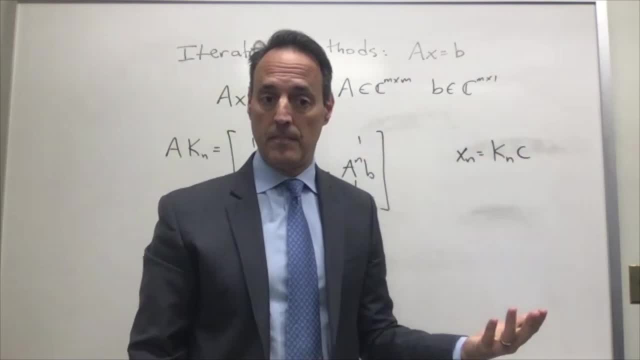 the question is: how do i pick c? i want to pick c, pick c, pick c so that minimizes the residual. okay, so that minimizes the residual. okay, so that minimizes the residual okay. so another way to think about it is this. so another way to think about it is this: 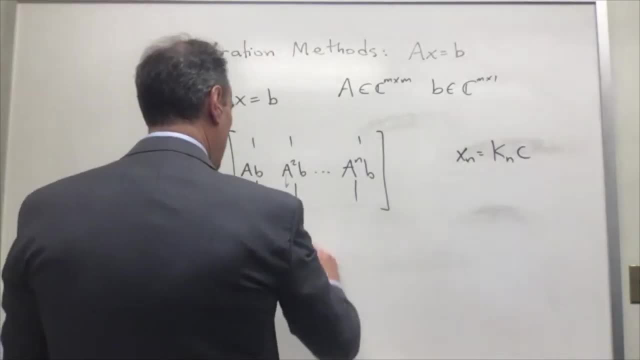 so another way to think about it is this: a k of n here, a k of n here, a k of n here. what i really want to do is say a k of n. what i really want to do is say a k of n. what i really want to do is say a k of n. c remember k of n. c is like my x. so 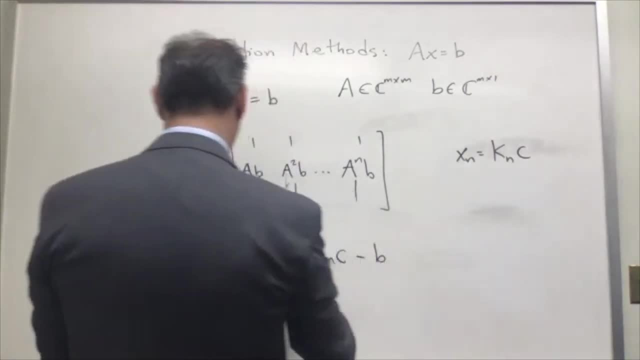 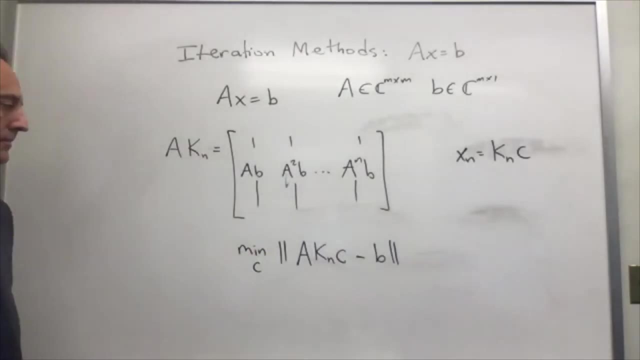 c remember k of n, c is like my x. so c remember k of n, c is like my x. so that's a x of n, that's a x of n, that's a x of n minus b, and i want to minimize this, minimize this, minimize this respect to the vector c, that's a least. 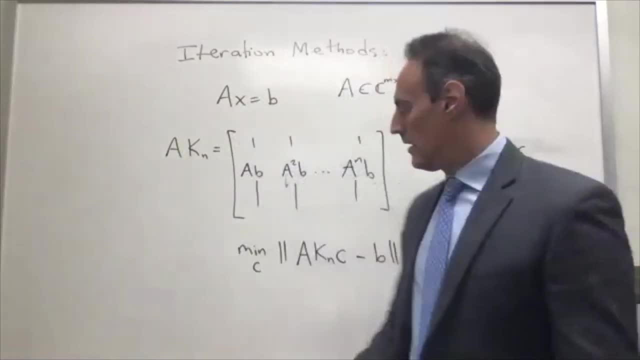 respect to the vector c. that's a least respect to the vector c, that's a least square fit right there, square fit right there, square fit right there. okay. and what c is doing is saying i am okay. and what c is doing is saying i am okay. and what c is doing is saying i am a linear. if i'm going to represent this, a linear. if i'm going to represent this a linear. if i'm going to represent this x of n, i'm going to pick c, which is a a linear. if i'm going to represent this x of n, i'm going to pick c, which is a. 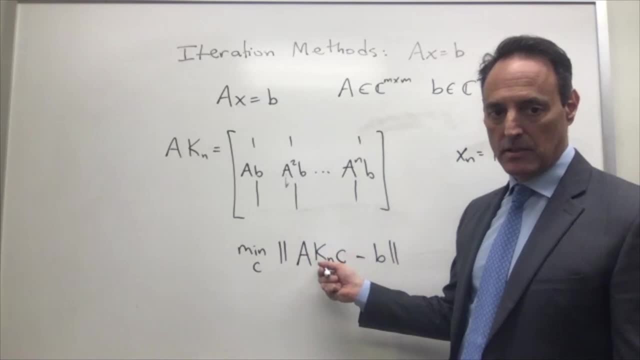 a linear. if i'm going to represent this x of n, i'm going to pick c, which is a linear combination. linear combination, linear combination on: crawl off subspace. crawl off sub on. crawl off subspace. crawl off sub on. crawl off subspace. crawl off sub vectors. 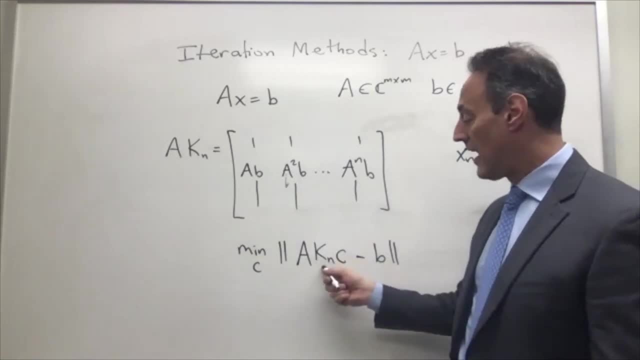 vectors. vectors: times a, i have b, i have a. i have times a, i have b, i have a, i have times a, i have b, i have a, i have k, so i have everything except for c, i k. so i have everything except for c, i k. so i have everything except for c. i want to determine those. c's those. 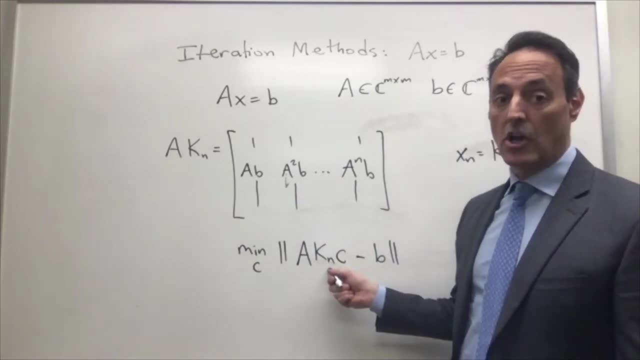 want to determine those c's, those want to determine those c's, those projections onto, projections onto, projections onto the k events, the columns of k of n, the k events, the columns of k of n, the k events, the columns of k of n, such that this quantity, here, the cell. 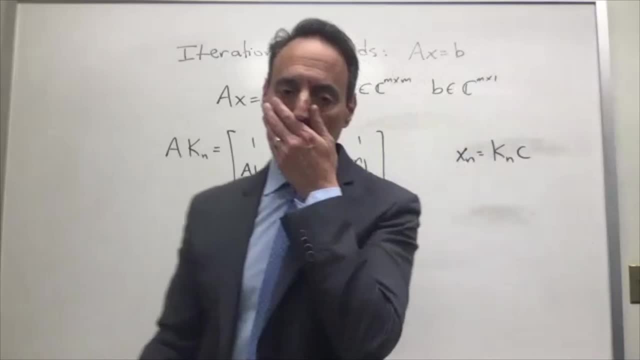 such that this quantity, here the cell, such that this quantity, here the cell, 2 norm, 2 norm, 2 norm- is minimized. okay, that's the, that's the high level. okay, that's the, that's the high level. okay, that's the, that's the high level idea. 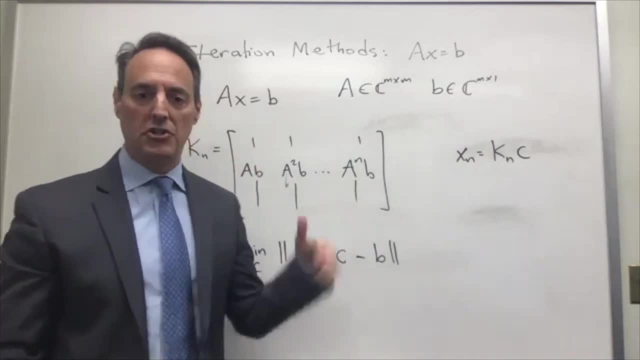 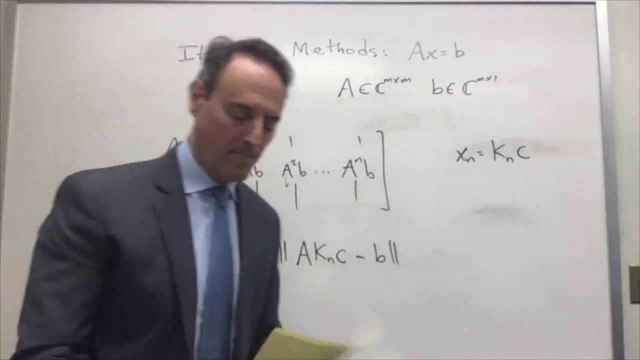 idea, idea of generalized method of residuals, of generalized method of residuals, of generalized method of residuals, that's it, that's it, that's it. you just at each step minimize the. you just at each step minimize the. you just at each step minimize the residual, residual, residual, that's the residual, okay. 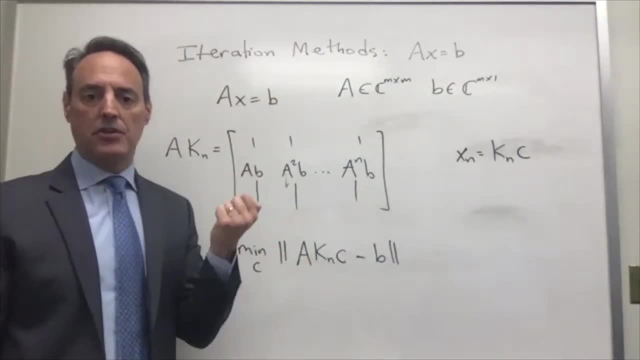 now we could work directly. now we could work directly. now we could work directly in this krylov matrix k event. but what's in this krylov matrix k event? but what's in this krylov matrix k event? but what's the problem with working with can of n? 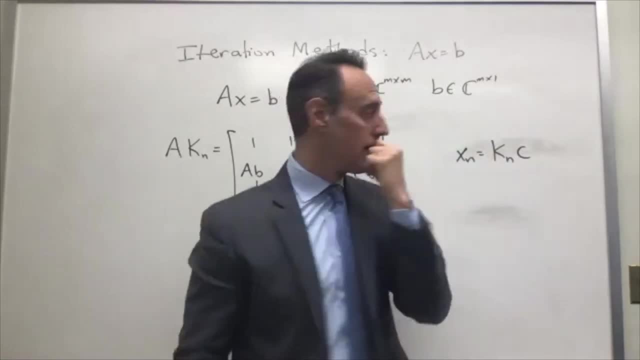 the problem with working with can of n. the problem with working with can of n directly, directly, directly. k of n is a bunch of columns right. k of n is a bunch of columns right. k of n is a bunch of columns, right. let me just draw it back here. 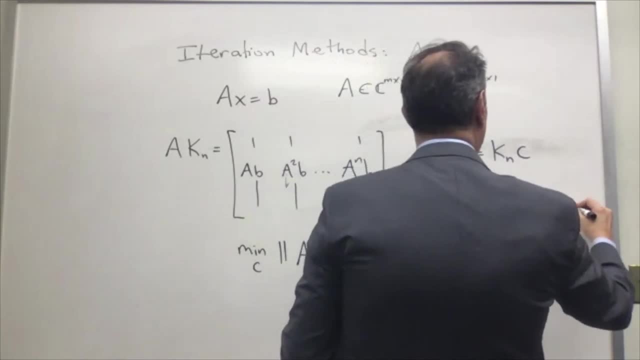 let me just draw it back here. let me just draw it back here: b a b- all the way to a of n minus one. b a b all the way to a of n minus one. b a b- all the way to a of n minus one b. 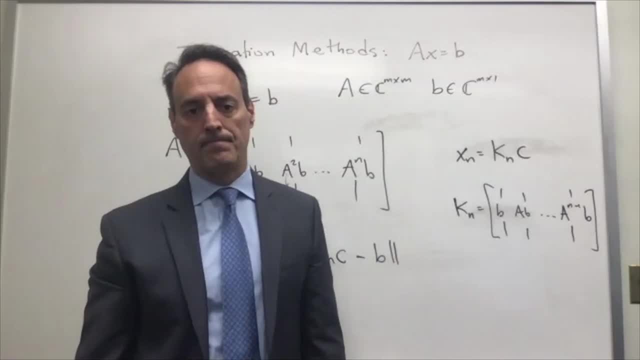 none of these are necessarily. none of these are necessarily. none of these are necessarily orthogonal to each other. orthogonal to each other. orthogonal to each other. right, they're just, they're not even right, they're just, they're not even right, they're just. they're not even normalized. so just, they're just a set. 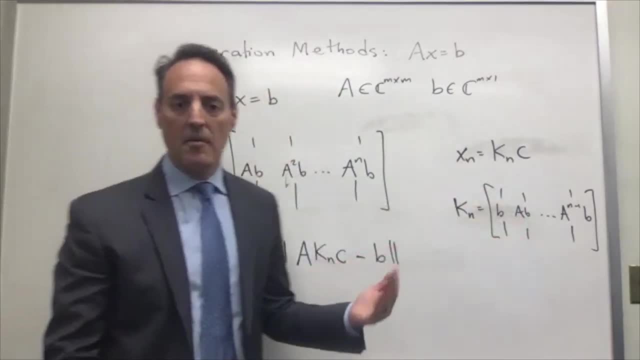 normalized, so just they're just a set. normalized, so just they're just a set of vectors. you can clearly do a linear of vectors. you can clearly do a linear of vectors. you can clearly do a linear combination of them, combination of them, combination of them. but we've started to learn in this class. 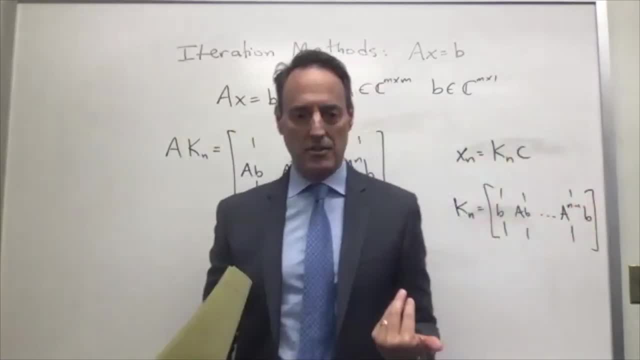 but we've started to learn in this class. but we've started to learn in this class, hopefully, hopefully, hopefully. that isn't it more advantageous? that isn't it more advantageous, that isn't it more advantageous to work with, to work with, to work with orthonormal vectors. 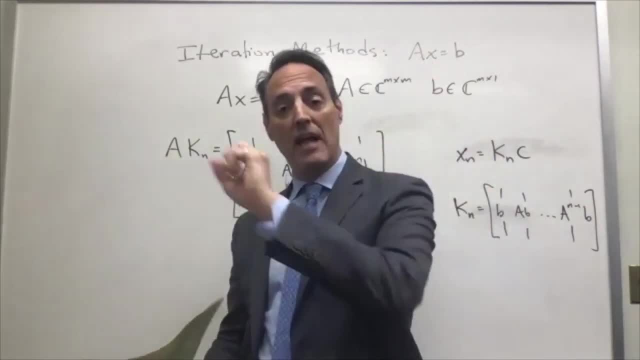 orthonormal vectors. orthonormal vectors: this is the power of the svd. it gives. this is the power of the svd it gives. this is the power of the svd it gives you, you, you and v, which are unitary transformations, and v, which are unitary transformations. 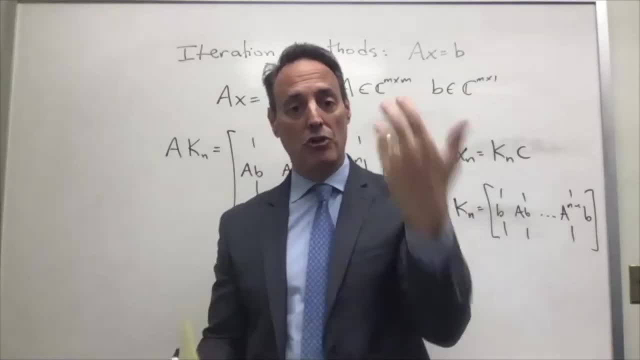 and v, which are unitary transformations. this was also the power of the qr. this was also the power of the qr. this was also the power of the qr. decomposition, decomposition, decomposition. it gave you a unitary transformation. it gave you a unitary transformation. it gave you a unitary transformation. times, an upper triangular, and we use 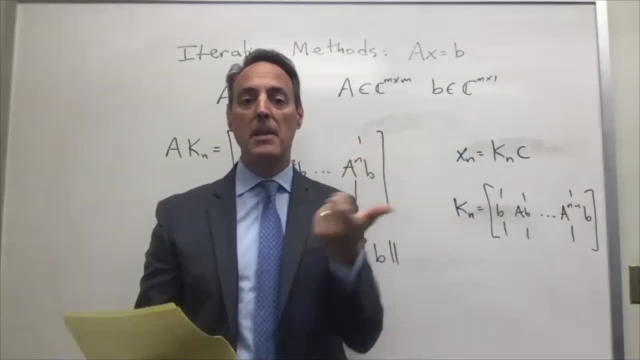 times an upper triangular and we use times an upper triangular and we use those to great effect. because those to great effect, because those to great effect, because those are very easy to manipulate, those are very easy to manipulate, those are very easy to manipulate. and we want to do the same thing here. 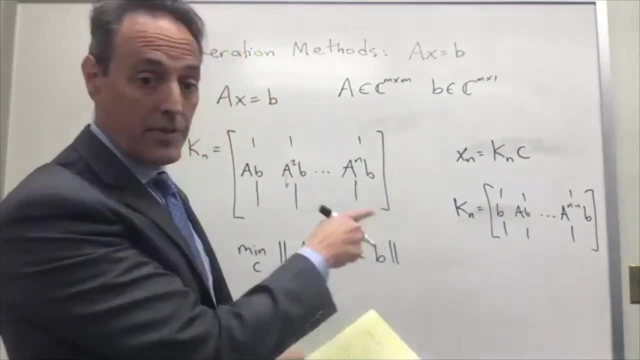 and we want to do the same thing here and we want to do the same thing here. what i mean by that is instead of what i mean by that is instead of what i mean by that is instead of working directly, with working directly, with working directly with this krylov matrix. we know that this 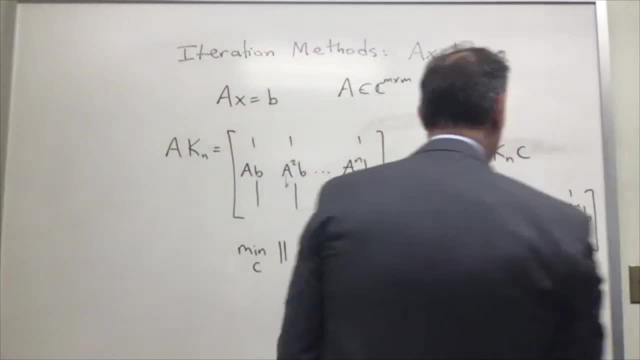 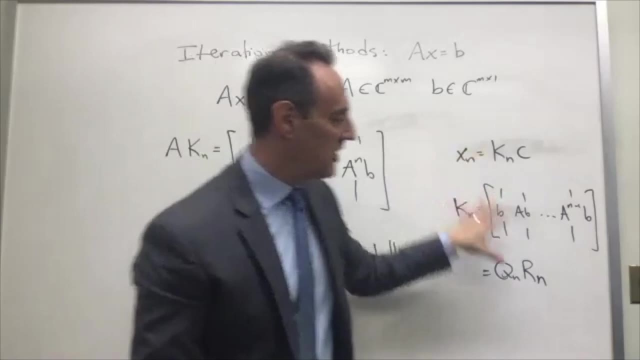 this krylov matrix. we know that this, this krylov matrix. we know that this thing here has a qr decomposition, and so, instead of has a qr decomposition, and so instead of has a qr decomposition. and so, instead of using these as basis elements, using these as basis elements. 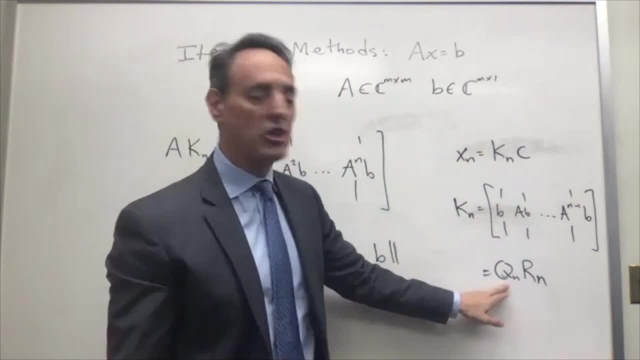 using these as basis elements. why not just use the qr? why not use? why not just use the qr? why not use? why not just use the qr? why not use these q events, these q events, these q events? they're orthonormal. this is a unitary. 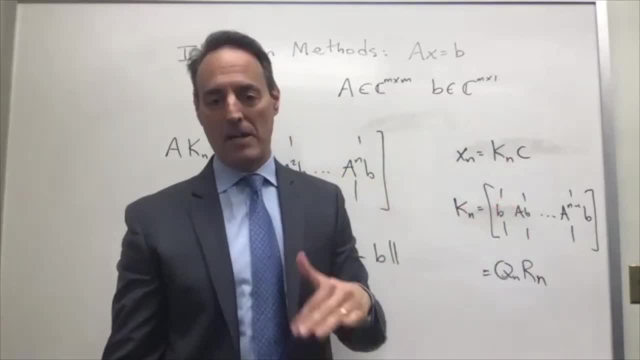 they're orthonormal, this is a unitary. they're orthonormal, this is a unitary. transformation, transformation, transformation. it is much better to work with that. it is much better to work with that. it is much better to work with that matrix, matrix, matrix, than the k of n. but this q event comes. 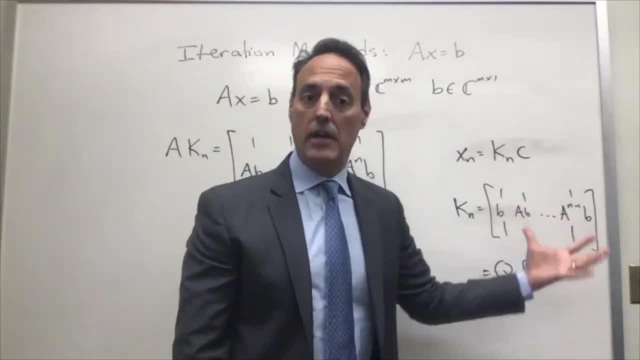 than the k of n, but this q event comes than the k of n, but this q event comes directly from the krylov subspace, directly from the krylov subspace, directly from the krylov subspace. okay, so this is a better representation. 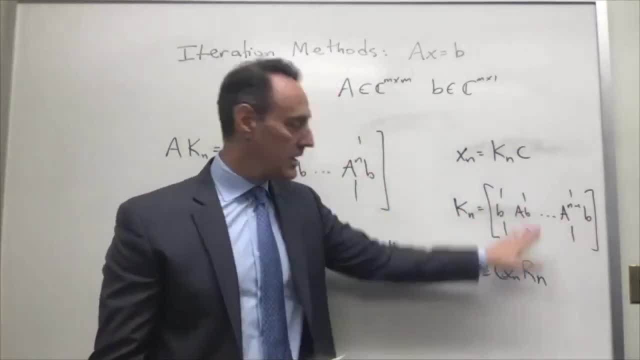 okay, so this is a better representation. okay, so this is a better representation of the krylov subspace, of the krylov subspace, of the krylov subspace, but nonetheless it's still coming from, but nonetheless it's still coming from, but nonetheless it's still coming from that. 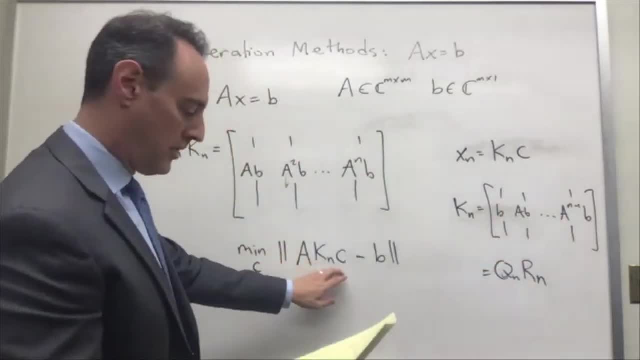 that that okay so, instead of solving this problem. okay, so, instead of solving this problem. okay, so, instead of solving this problem, what we know is we can say: well, what we know is we can say: well, what we know is we can say: well, another way to do it is this: here, which? 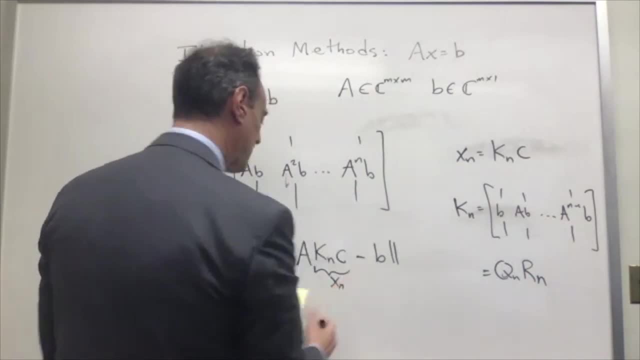 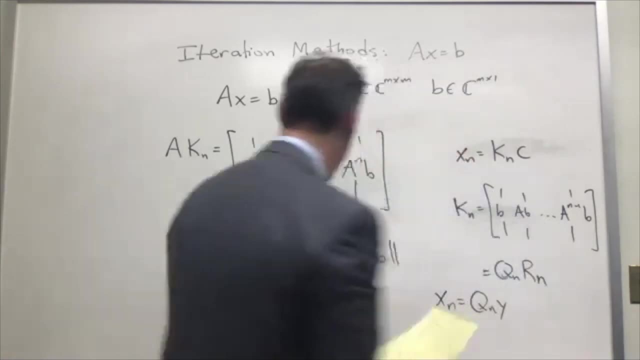 another way to do it is this here. which another way to do it is this here: which is my, is my, is my x of n. i could instead say x of n is equal. to say x of n is equal. to say x of n is equal to, instead of projecting c times q of n. 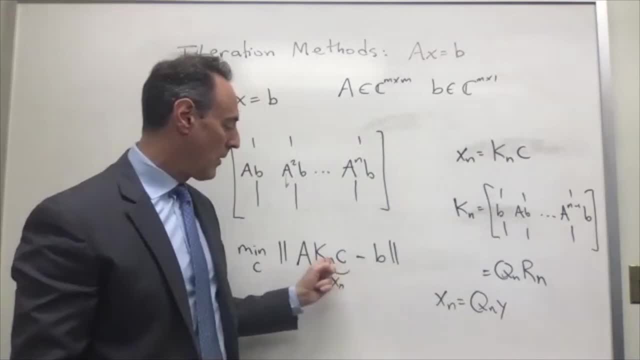 instead of projecting c times q of n, instead of projecting c times q of n as a linear combination, as a linear combination, as a linear combination, i could instead say: well, why work with? i could instead say well, why work with? i could instead say well, why work with that basis, when i could work with? 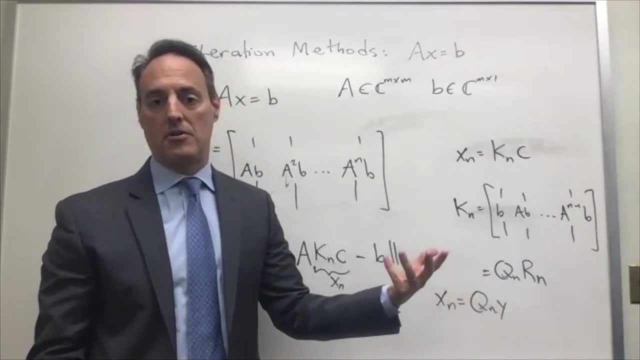 that basis, when i could work with that basis, when i could work with the q events and y is now what i try to the q events and y is now what i try to the q events and y is now what i try to determine instead of c. 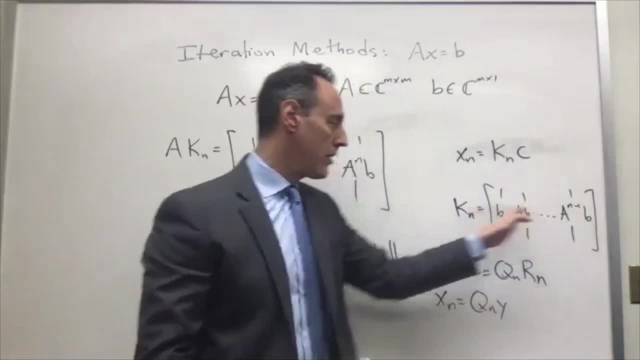 determine instead of c. determine instead of c. remember. c is just the loadings onto remember. c is just the loadings onto remember. c is just the loadings onto which one of these cop, which one of these cop, which one of these cop. the linear combination is columns. 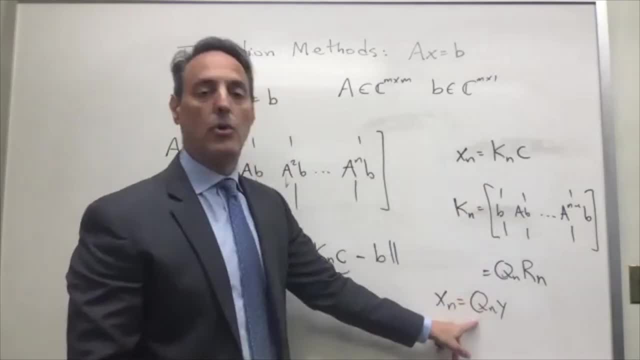 the linear combination is columns. the linear combination is columns: whereas y now is. whereas y now is. whereas y now is: same idea, but now onto an orthonormal same idea, but now onto an orthonormal same idea, but now onto an orthonormal basis basis. 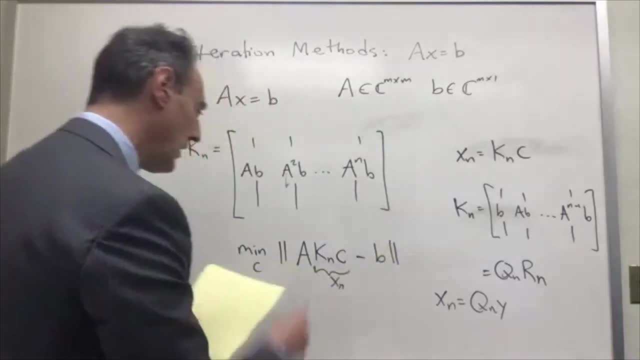 basis, which is much easier to work with, which is much easier to work with, which is much easier to work with. so really at the end of the day, so really at the end of the day, so really at the end of the day, what i would do, what i would do. 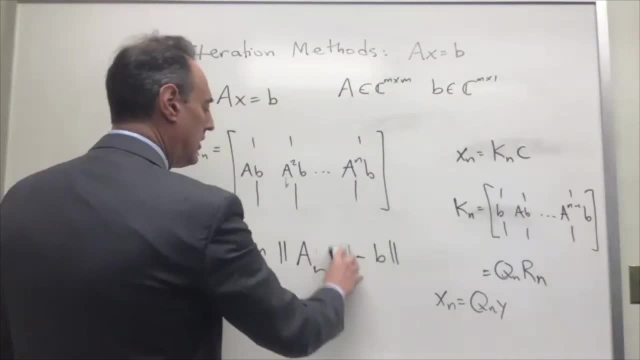 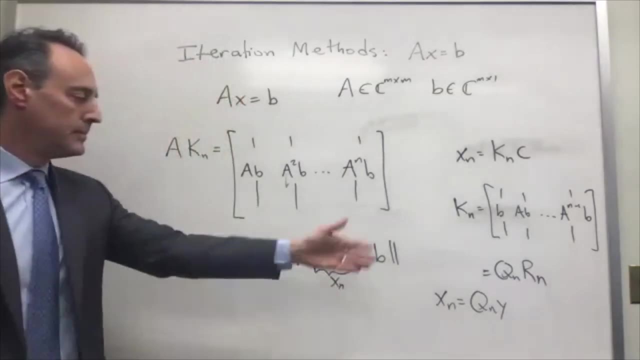 what i would do is, instead of using this x of n is, instead of using this x of n is, instead of using this x of n, you trade it out, you trade it out. you trade it out. or q of n, or q of n or q of n? y. 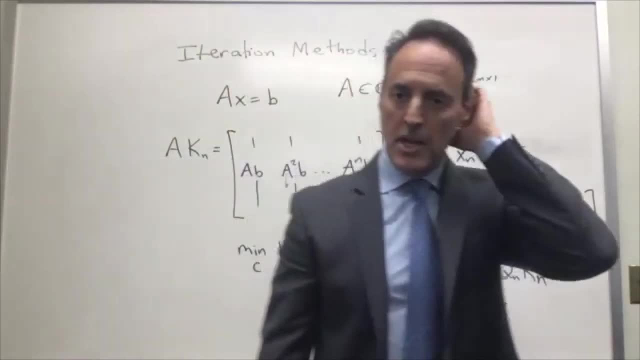 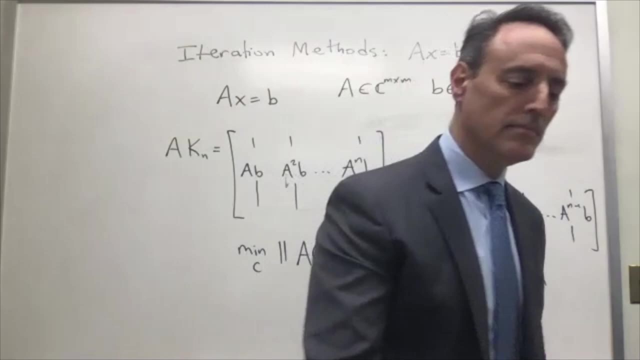 y y, okay, okay, okay. so this is a a nice representation. so this is a a nice representation, so this is a a nice representation of that krov krylov subspace. all right, there's a lot of pieces to. all right, there's a lot of pieces to. 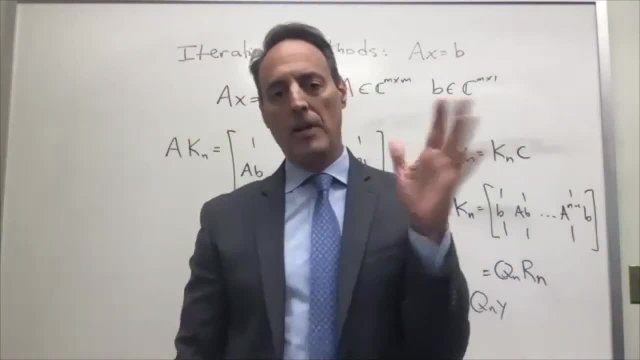 all right, there's a lot of pieces to this, by the way, and i'm going to also this, by the way, and i'm going to also this, by the way, and i'm going to also make this comment, make this comment, make this comment. i'm only doing a very superficial. 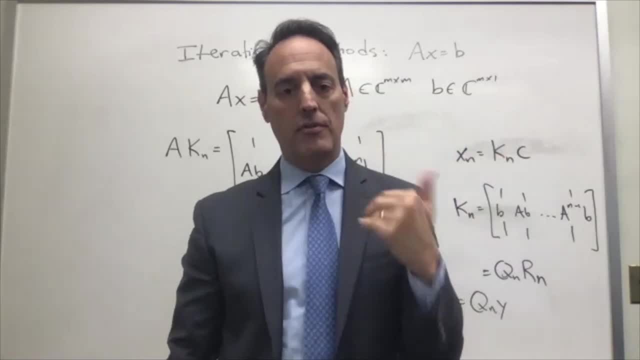 i'm only doing a very superficial, i'm only doing a very superficial: scratching the surface of iterative, scratching the surface of iterative, scratching the surface of iterative methods, methods, methods. if you look at trefethen's book, if you look at trefethen's book, 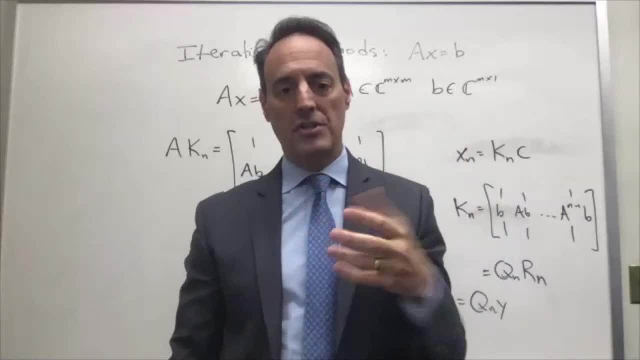 if you look at trefethen's book, there's a whole lot more there. there's a whole lot more there. there's a whole lot more there also. there's entire books on iterative also. there's entire books on iterative also. there's entire books on iterative techniques, one by anne greenbaum. 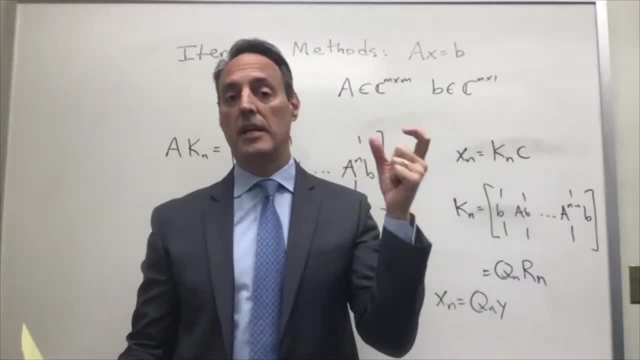 techniques- one by anne greenbaum. techniques- one by anne greenbaum. that is probably the the best in the. that is probably the the best in the. that is probably the the best in the field. it's all about just field. it's all about just field. it's all about just iterative solvers for linear systems. 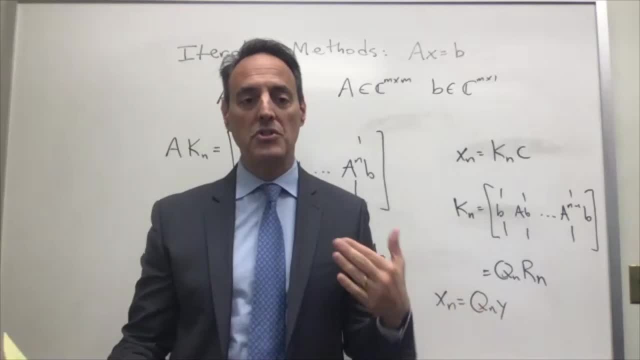 iterative solvers for linear systems, iterative solvers for linear systems, and that's a whole field in itself, and that's a whole field in itself, and that's a whole field in itself. okay, so we're just talking about some. okay, so we're just talking about some. 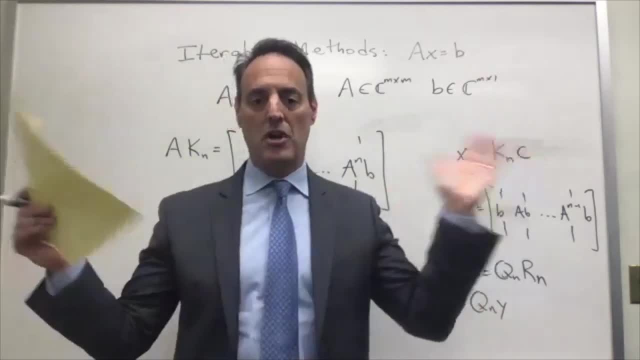 okay. so we're just talking about some very high level concepts here, very high level concepts here, very high level concepts here, because we have so much to talk about in, because we have so much to talk about in, because we have so much to talk about in the course. 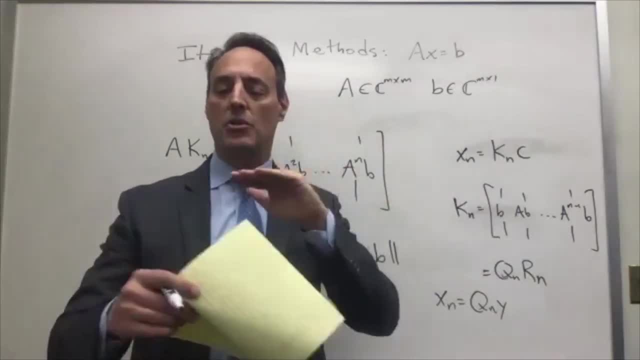 the course, the course, and so we're not going to get into a lot, and so we're not going to get into a lot, and so we're not going to get into a lot of depth here, of depth, here, of depth here. but i'm going to sort of sketch out for 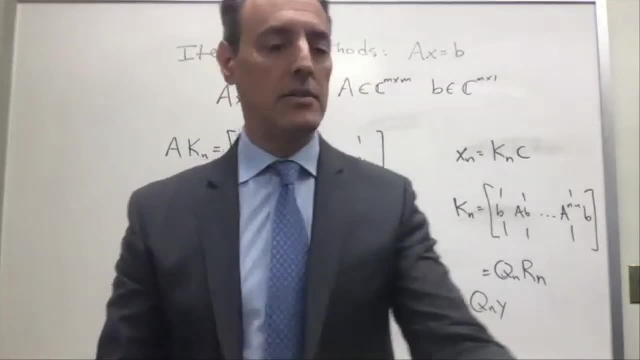 but i'm going to sort of sketch out for, but i'm going to sort of sketch out for you some of the important things here you, some of the important things here you, some of the important things here, and then, if you want, and you get very, and then if you want and you get very. 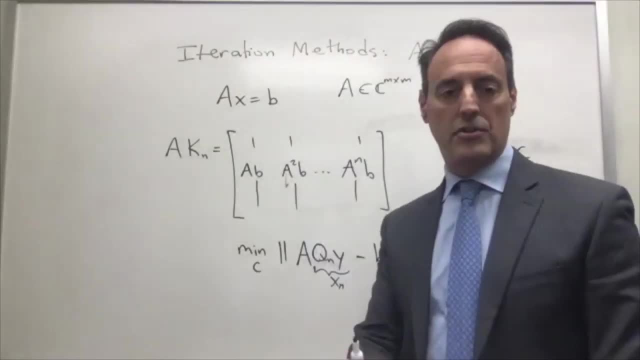 and then, if you want and you get very interested in this stuff, interested in this stuff, interested in this stuff, there's a lot more out there to, there's a lot more out there to. there's a lot more out there to follow up on, follow up on. i have a quick question. yes, does the? 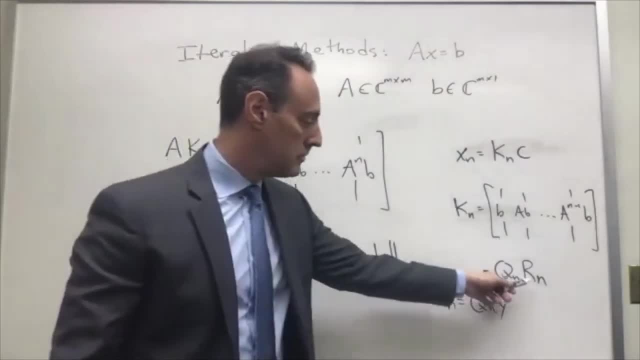 i have a quick question. yes, does the? i have a quick question: yes, does the? fact r is missing here. uh, fact r is missing here. uh, fact r is missing here. uh affect which set of uh columns you're affect. which set of uh columns you're affect. which set of uh columns you're selecting. 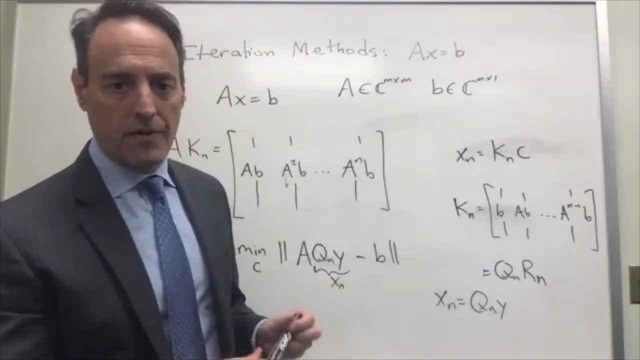 selecting, selecting the fact that r is missing. so i'm not the fact that r is missing. so i'm not the fact that r is missing. so i'm not sure if i understand the question. sure, if i understand the question. sure if i understand the question. so, instead of saying uh, x being uh, 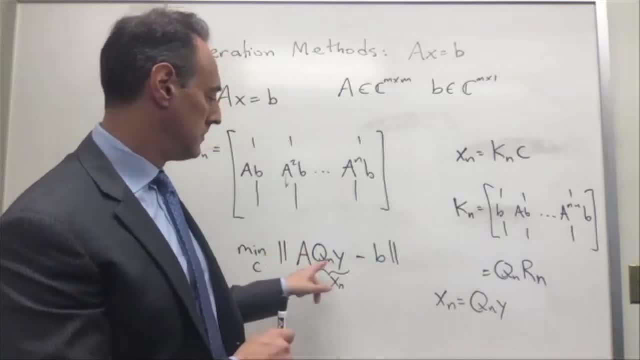 so, instead of saying uh x being uh, so instead of saying uh x being uh kc, now you're using uh qy right kc. now you're using uh qy right kc. now you're using uh qy right, yeah, um, yeah, um, yeah, um. so basically you're saying x is qy. 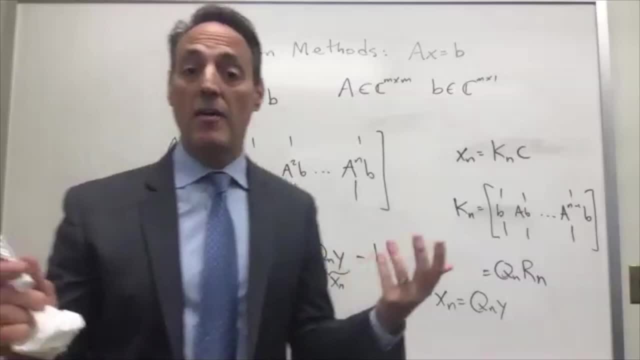 so basically, you're saying x is qy. so basically you're saying x is qy without uh considering r at all. yeah, i without uh considering r at all. yeah, i without uh considering r at all. yeah, i don't care about r, don't care about r. 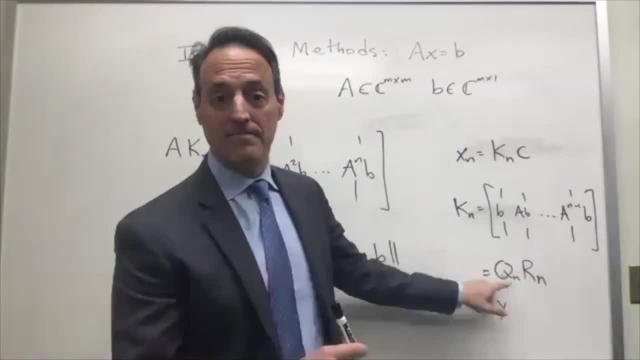 don't care about r. all i care about are these orthonormal. all i care about are these orthonormal. all i care about are these orthonormal vectors, vectors, vectors. that's it i just want to take go from. that's it i just want to take go from. 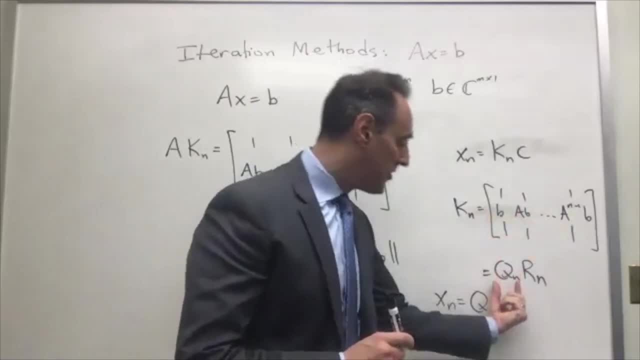 that's it. i just want to take go from working in that coordinate system, this, working in that coordinate system, this, working in that coordinate system, this. so, in other words, this here spans that. so, in other words, this here spans that. so, in other words, this here spans that subspace, and that's all i care about. 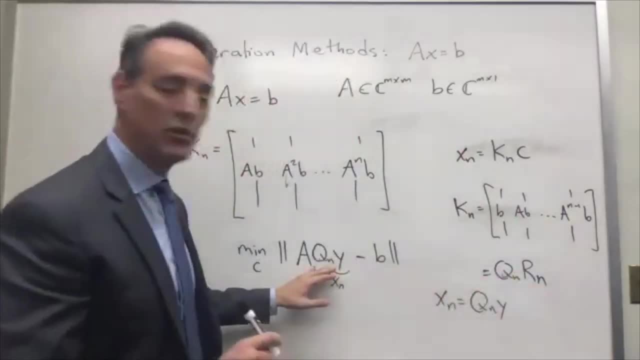 subspace, and that's all i care about. i don't really care how i got there once. i don't really care how i got there once. i don't really care how i got there once. i get them, i get them. i get them, i use them. 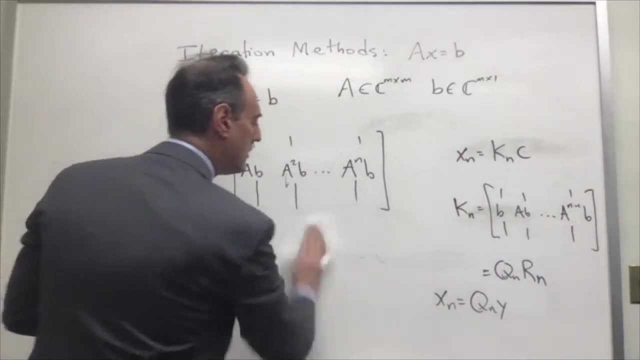 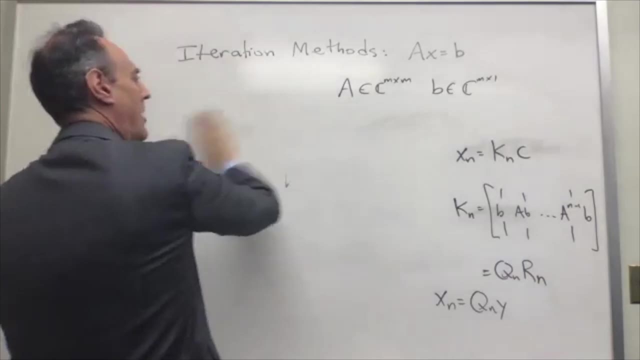 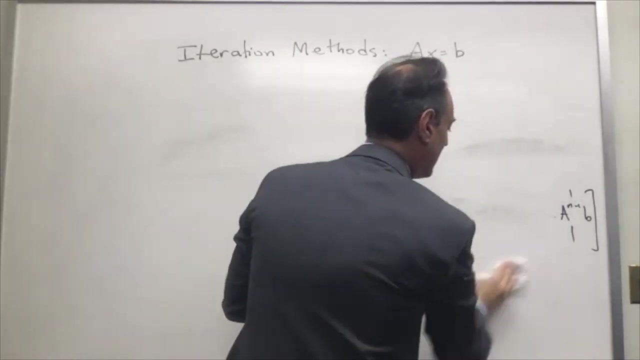 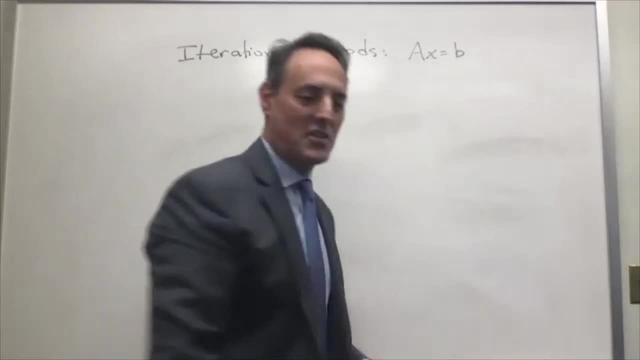 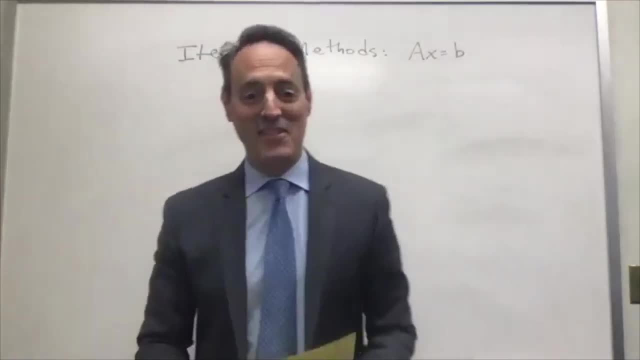 arnold, or actually arnoldi. i'll know the iterations, iterations, iterations. i was talking about arnold schwarzenegger. i was talking about arnold schwarzenegger. i was talking about arnold schwarzenegger. these are like arnold schwarzenegger. 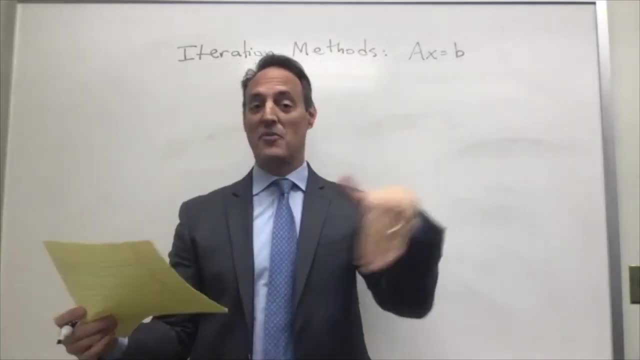 these are like arnold schwarzenegger. these are like arnold schwarzenegger anyway. this is like the powerful method anyway. this is like the powerful method anyway. this is like the powerful method for doing iterations, and it turns out for doing iterations, and it turns out. 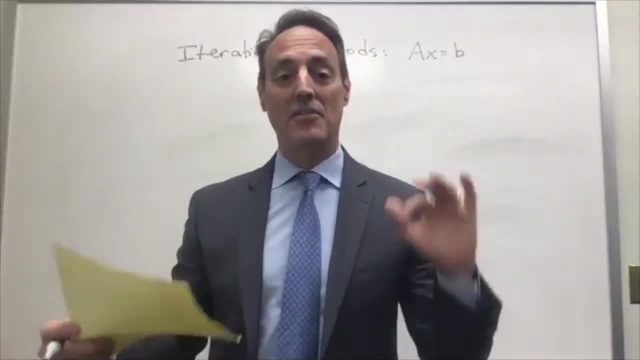 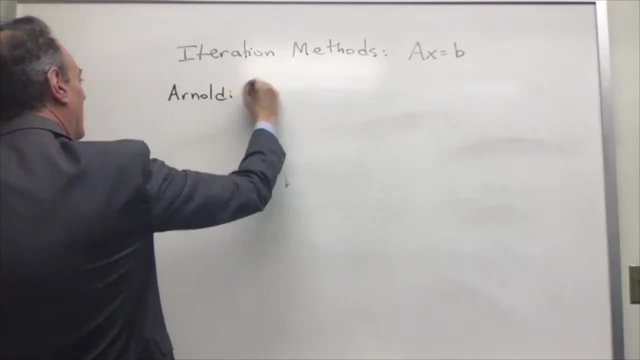 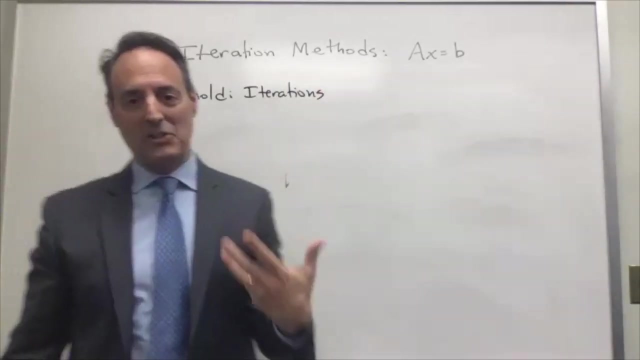 for doing iterations and it turns out it underlies a lot of the fundamental. it underlies a lot of the fundamental. it underlies a lot of the fundamental ideas of these iteration techniques are null the iterations. okay. so now we're going to come back to. okay, so now we're going to come back to. 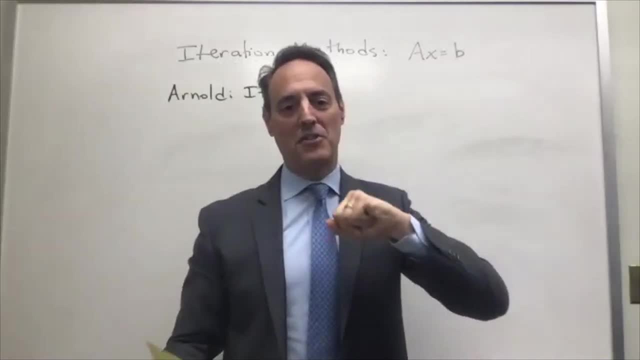 okay, so now we're going to come back to some ideas that we already learned, some ideas that we already learned, some ideas that we already learned before before, before about matrices, and we were doing this about matrices and we were doing this about matrices and we were doing this with eigenvalue, eigenvector. 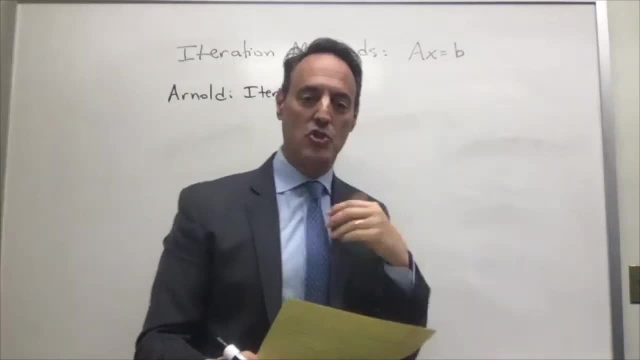 with eigenvalue eigenvector, with eigenvalue eigenvector: uh uh uh. algorithms, algorithms, algorithms which is transforming the matrix and which is transforming the matrix and which is transforming the matrix, and then using iterative procedure, then using iterative procedure, to find the eigenvalues and eigenvectors. 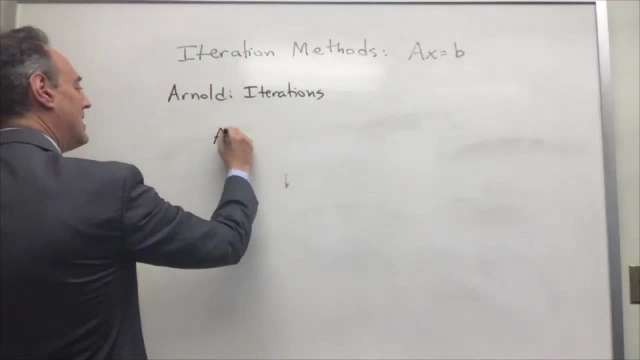 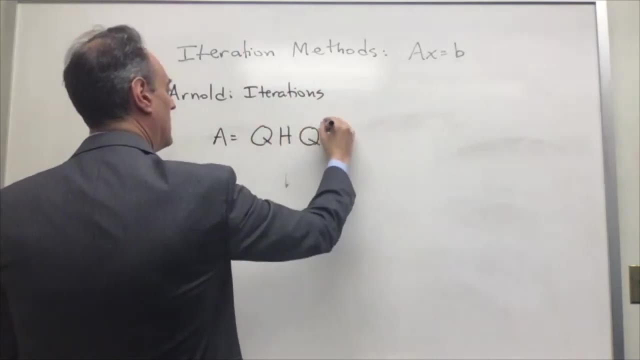 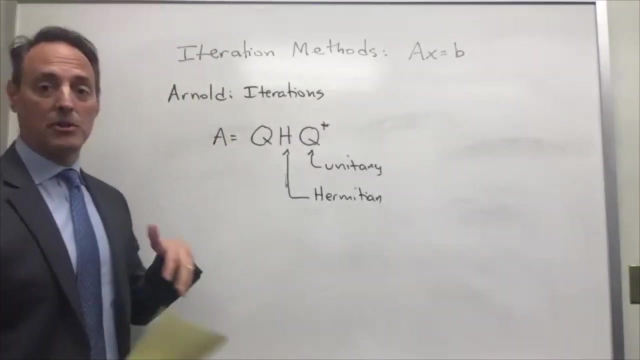 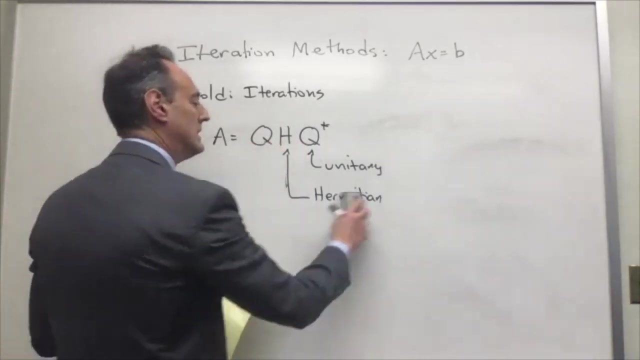 So, in particular, we can write a matrix A in self-similar form with the following transformation: Q is unitary and H is Hermitian. So this is a full self-similar transformation into a complete orthonormal set of vectors. And this is in sorry, not Hermitian, sorry, Hessenberg. 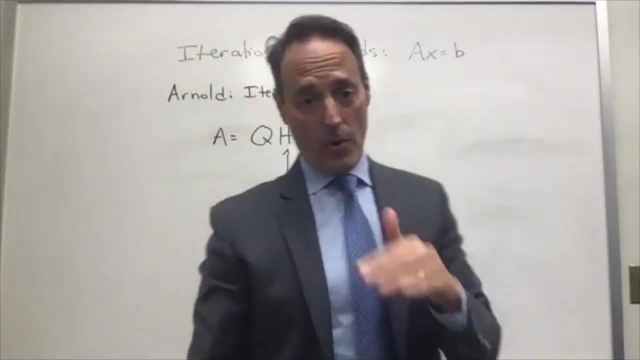 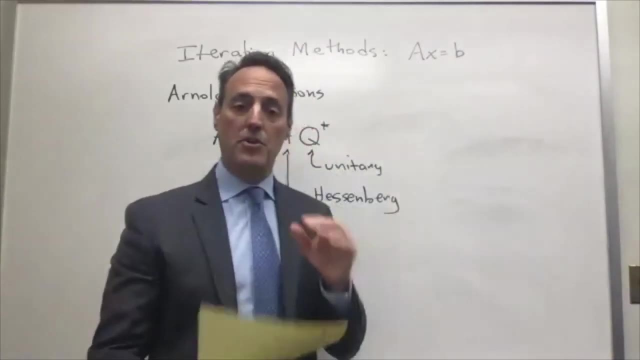 So you can put this in Hessenberg form. In fact, that is the one of the ways, the first tricks you do for doing eigenvalue, eigenvector decompositions. If you remember what we talked about, some of the algorithms there. 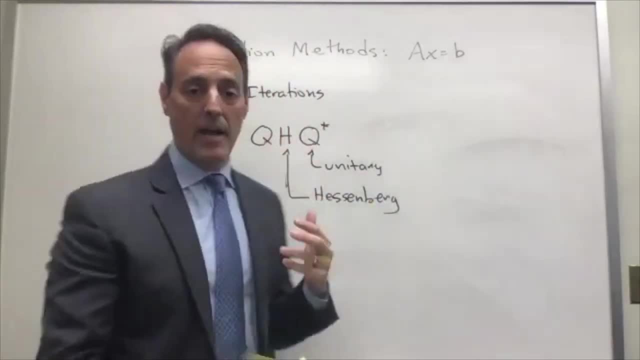 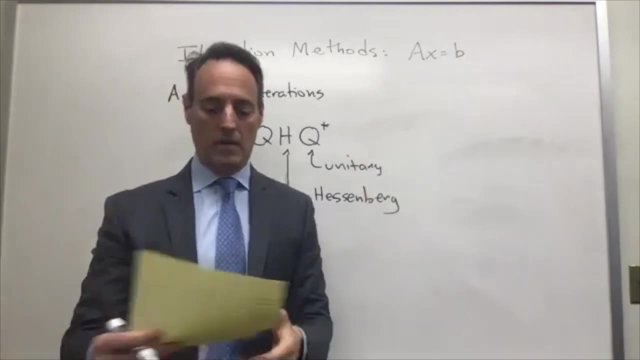 the idea was to recursively first put it in Hessenberg form and once you have it in there, then finish off your eigenvalues by doing iterations. okay, Here we just have this form, which tells us: okay, I know, I can do this decomposition. 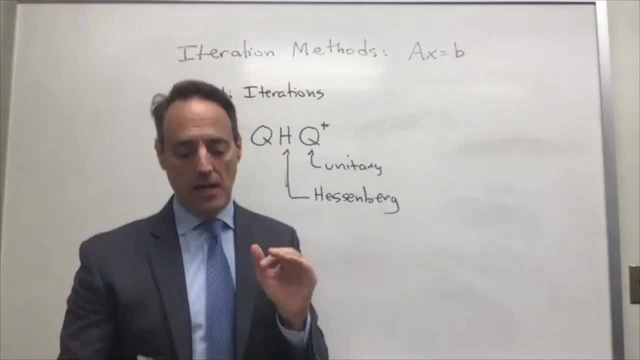 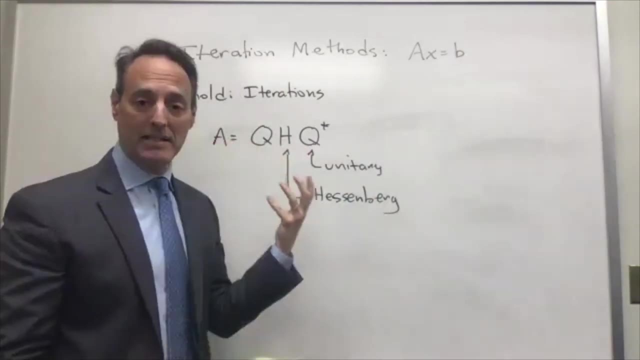 and this is where we're gonna make a connection to this idea of when I do a part as I start to do this decomposition. this is a full decomposition And if this matrix A is massive, I don't wanna do a full decomposition. 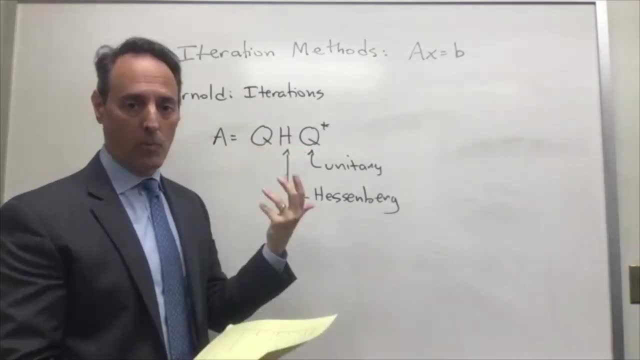 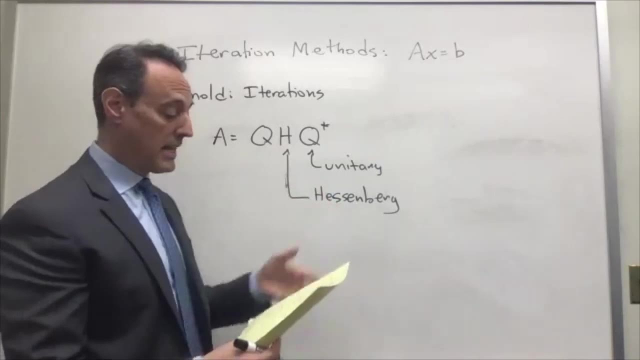 What I really like to do is start doing this decomposition stop wherever I want, Okay, And so I wanted to go N iterations in. And what does that look like? Well, so first of all, I can rewrite this by multiplying on the right-hand side. 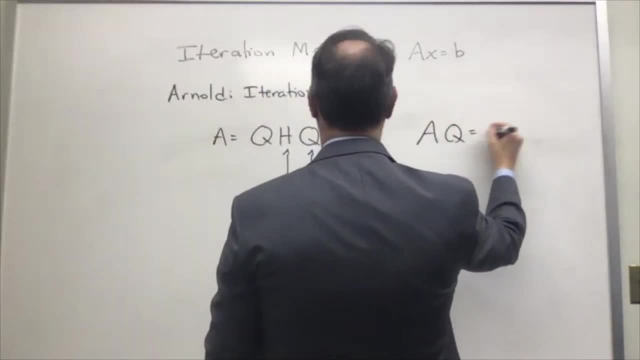 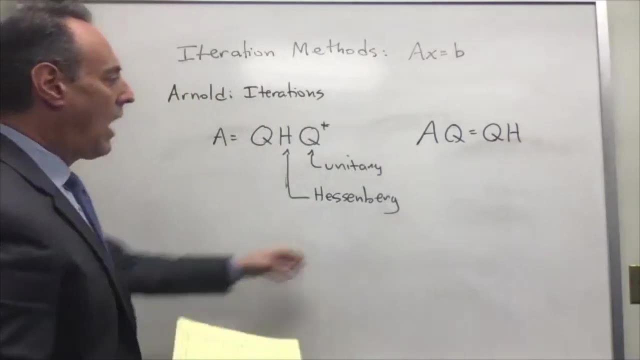 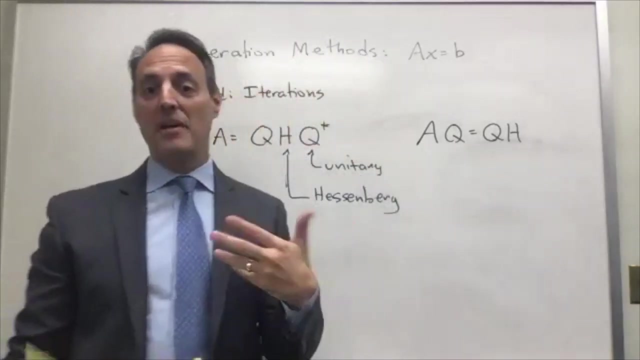 by Q, as AQ equals QH. okay, And what I really wanna look at is how would I get the first N columns of that Q Okay? Now it turns out, if you do it a little bit, if you do a little bit of linear algebra. 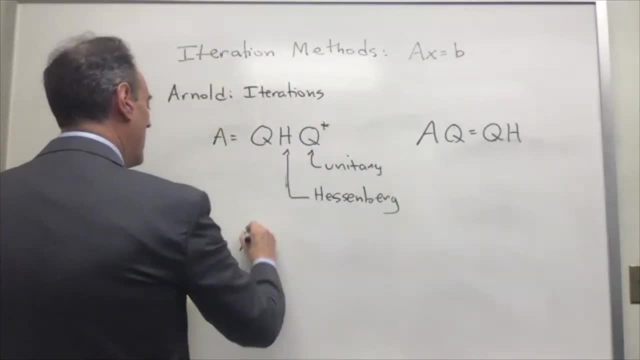 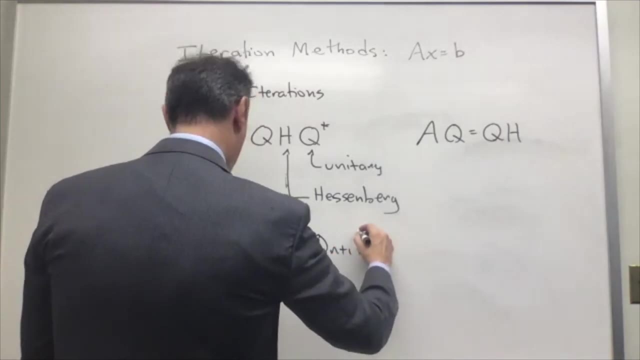 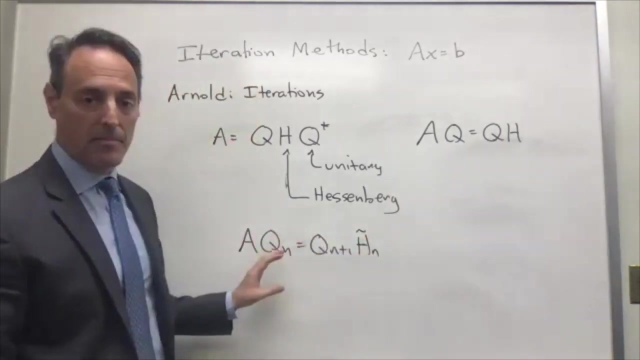 I won't do it here. you find this interesting relationship: A acting on Q of N is equal to Q of N plus one HN. So all of these are partial decomposition. So this I'm not doing a full decomposition. What I'm looking at is just the first N columns. 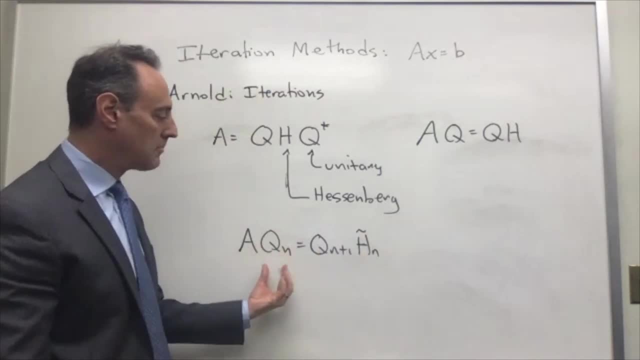 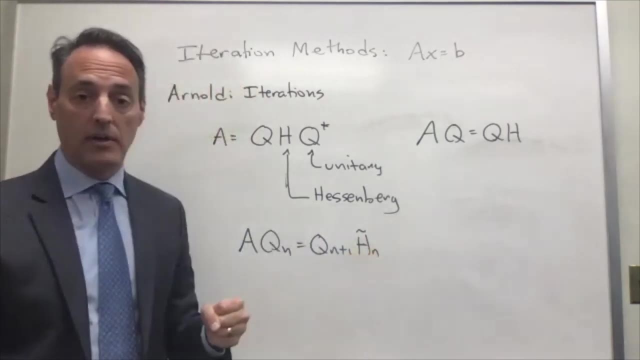 And here's the important thing You find when you do the first N columns: there is a recursion relationship between Q of N to Q of N plus one, because this thing is Hessenberg. So we can work this all out, by the way. 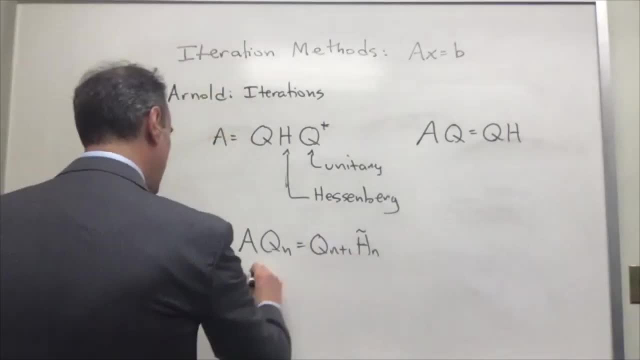 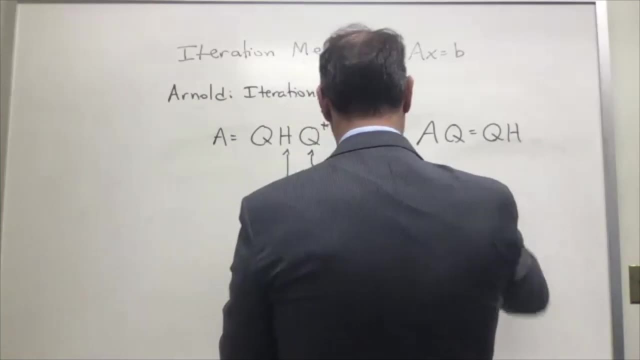 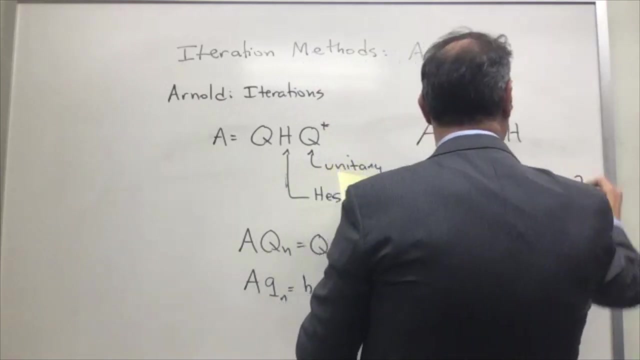 And in fact, what this tells you is that A acting on Q of N is equal to H1N. In fact, let me write down the Hessenberg matrix: H is equal to 811H12H1N, And remember it's diagonal merchandise right. 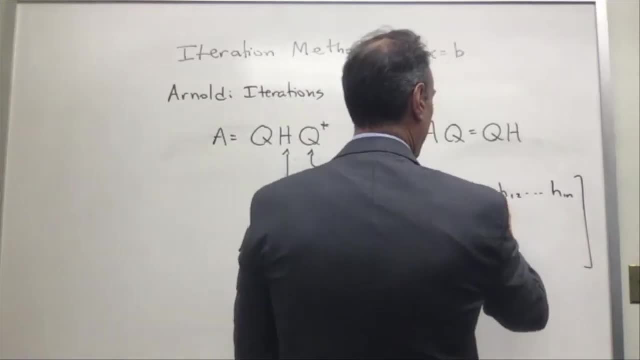 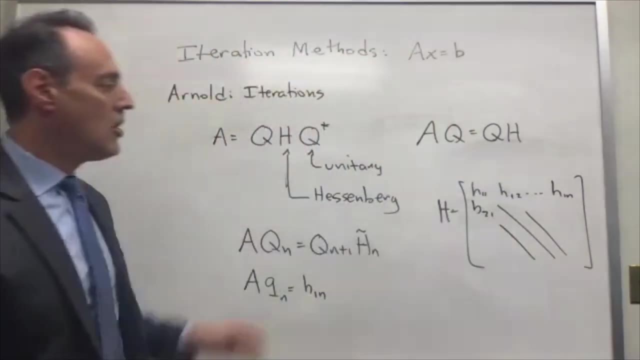 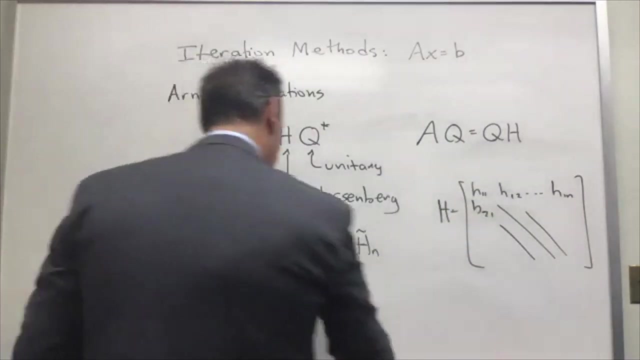 So we're gonna do this. it's diagonal, with one of the off the below diagonal not being zero, h two one and everything else here is zero. but because it has this form, it creates a recursion relationship between the q of n to q of n plus one, which is h one, n, q of one plus all the way to h. 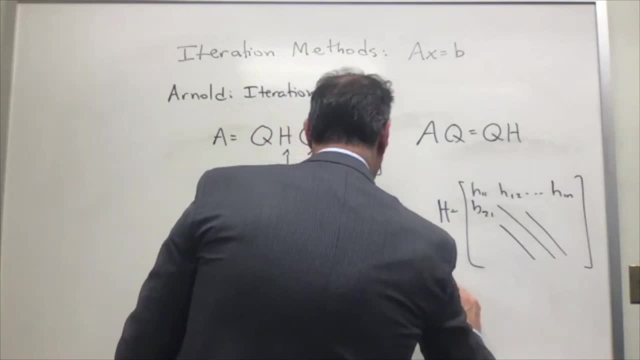 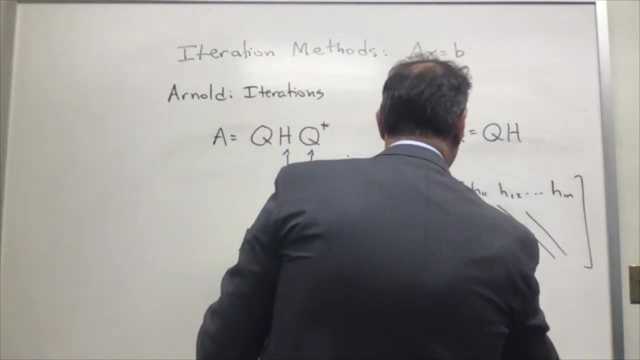 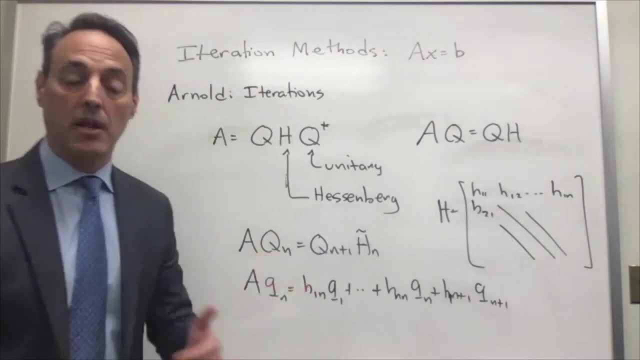 n and q of n plus h, n plus one, uh sorry, one n plus one, q of n plus one. and this is a really important recursion formula. it's the basis of these arduino iterations. in other words, once i have the q of n, i can get q of n plus one. once i have the q of n plus one, i can go get the q of n. 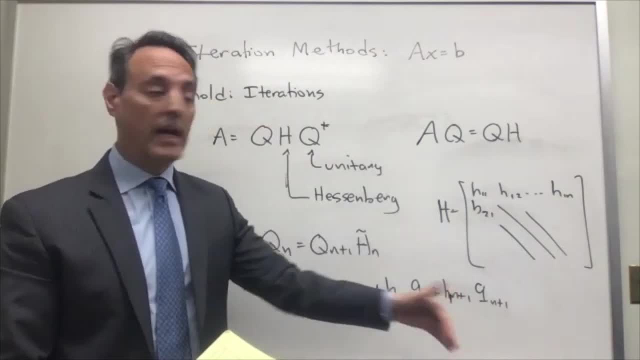 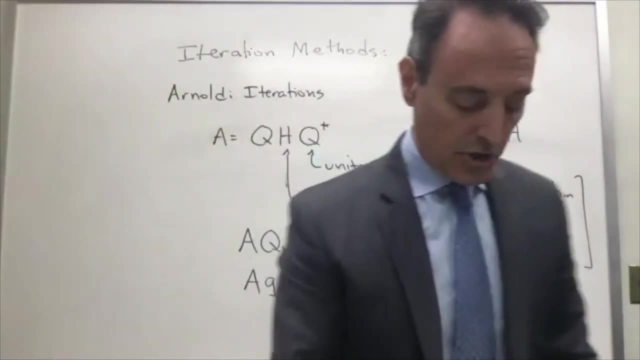 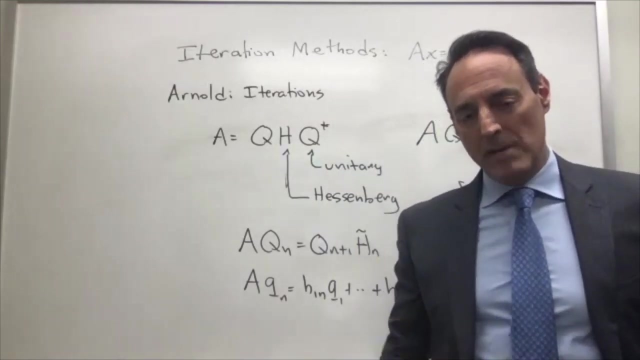 plus two. once i get q of n plus three i can go get the q of n plus three. i have a connection. formula you, O. so this is in some sense a different version of graham schmidt. right, because i start off with a certain number of directions. remember graham schmidt started. 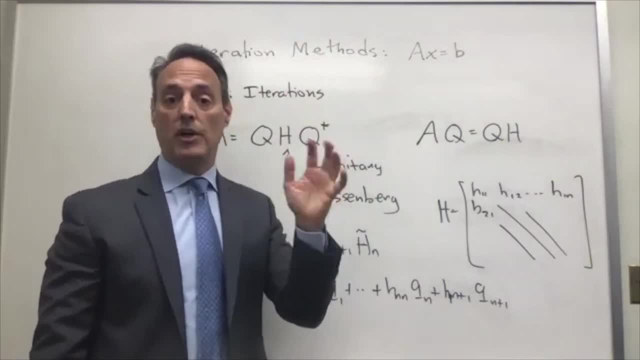 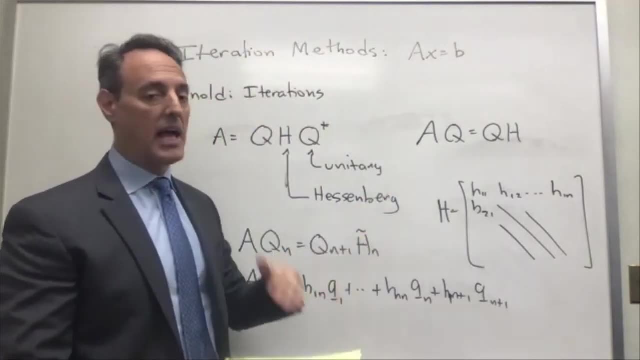 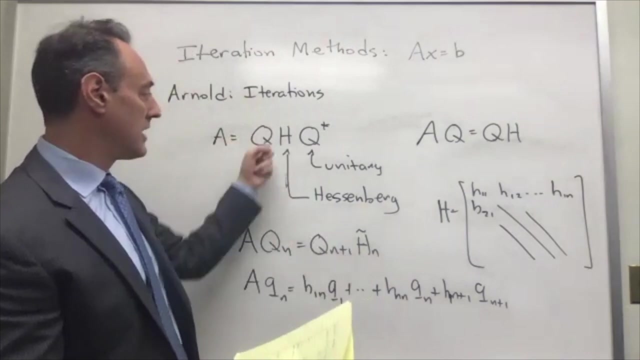 with q1, which then allowed you to get q2. once you have q1, q2 allows you to get q3. once you q1, q3, you get q4. same kind of idea here, once i. i'm just building it recursively and this is the recursion formula that you have from this diagonalization here, which is a. 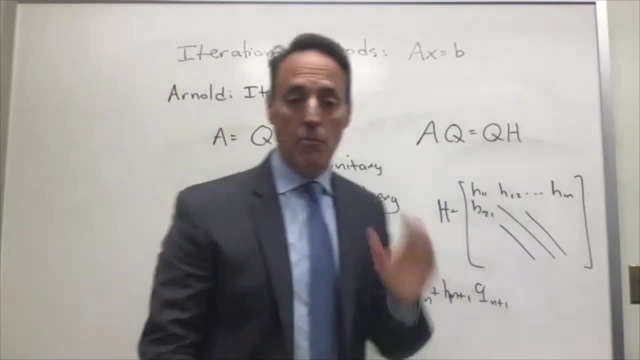 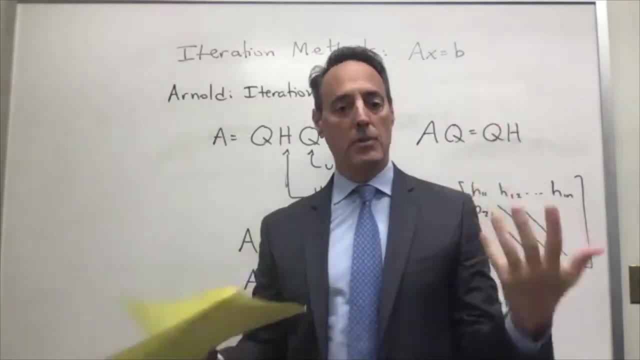 self-similarity, transformation to the hessenberg. and remember, if you look back at those lectures on eigenvalues and eigenvectors we talked about, how could you do decompositions in a principled way, to put any matrix in the hessenberg form and then from the hessenberg form, then you can finish. 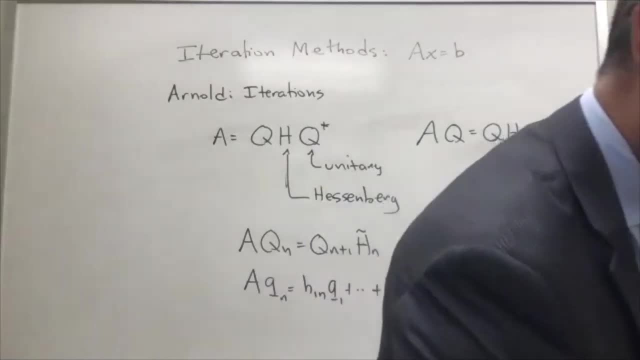 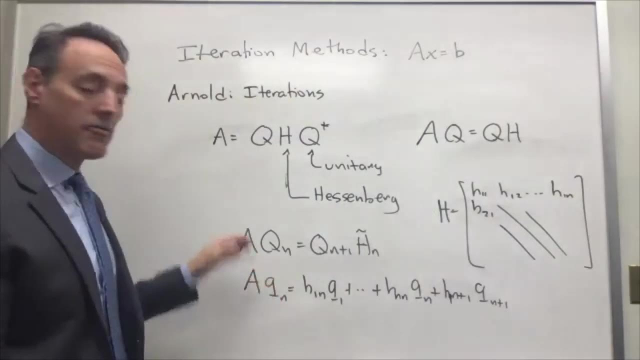 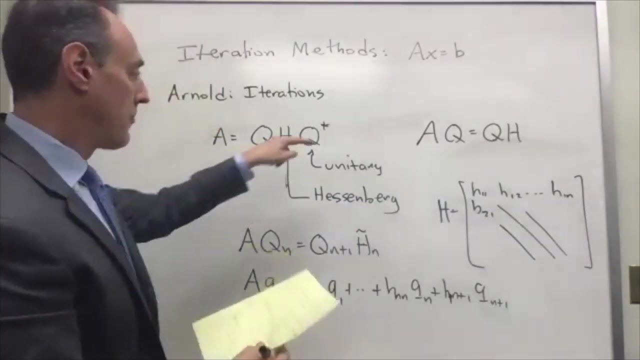 it off with iterations. so this is the main idea behind arnoldi- is: i have now a recursion relationship that allows me to just iterate from q of q of n to get q of n plus one. okay, so we have this formula here. this is an important one. 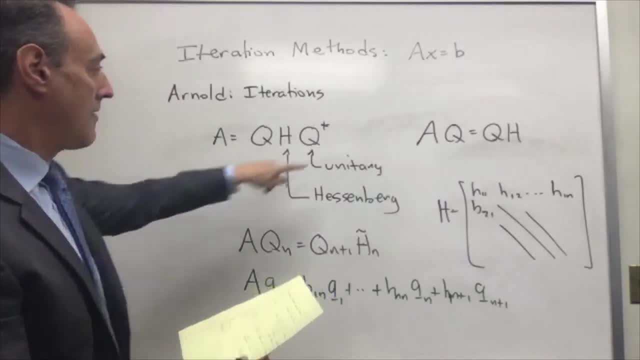 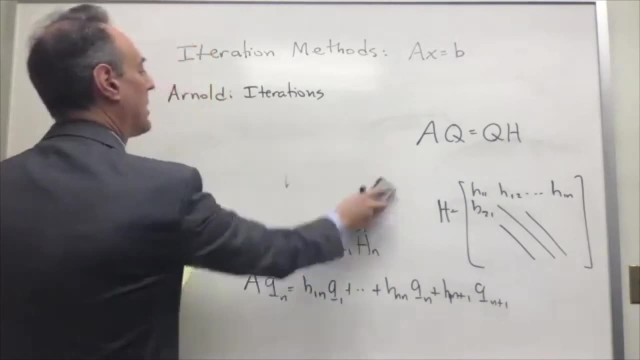 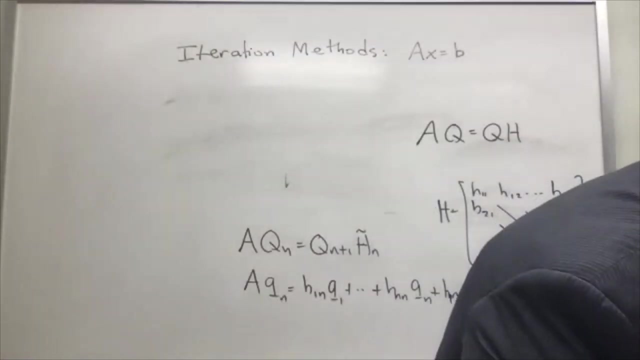 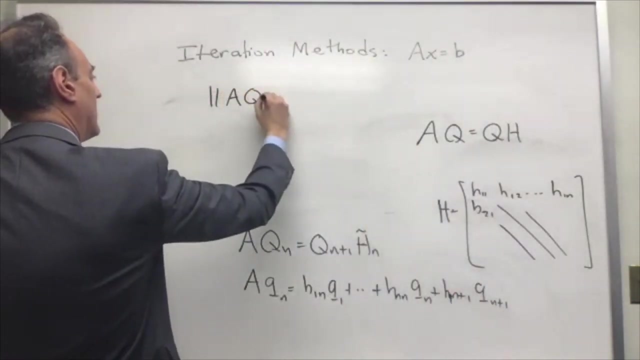 okay, and we have a of q of n now. remember, let me erase here what we had previously. how do we bring martin olding in then to this gm res? well, if you remember what we wrote down, with gm res, we're trying to minimize the residuals, and that was minimize this q of n y minus b. 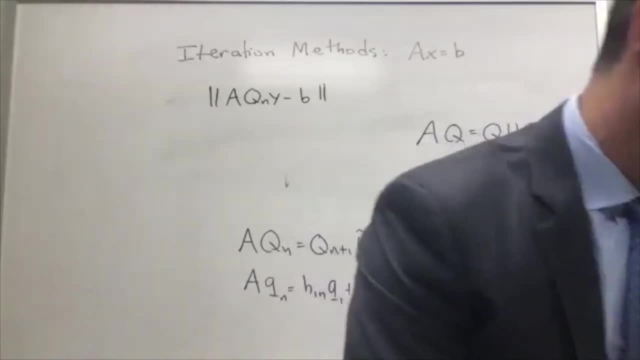 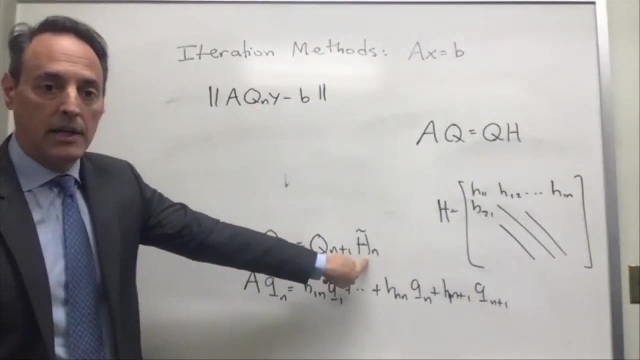 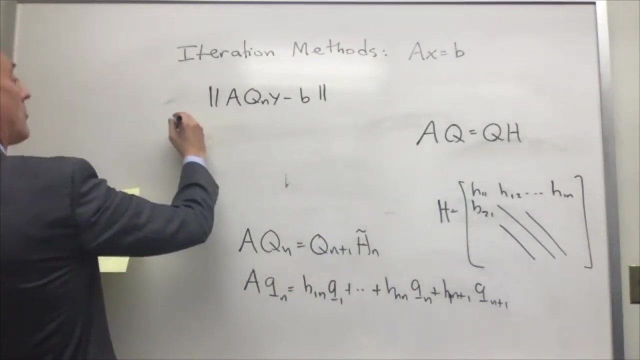 well, a of q of n is here is actually q of n plus one h of n. so when i come back to here then i'm saying: well, i'm going to minimize this over y, which is equal to minimize over y. this a of n? q is now q of n plus one. 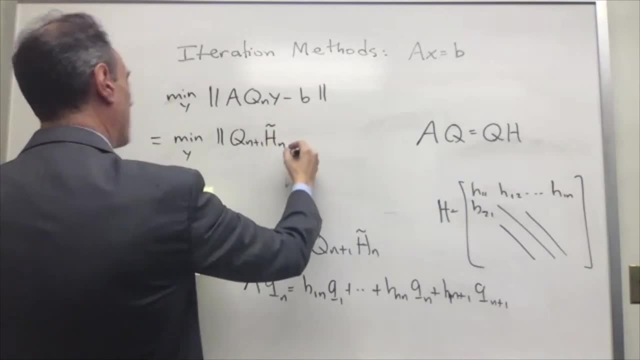 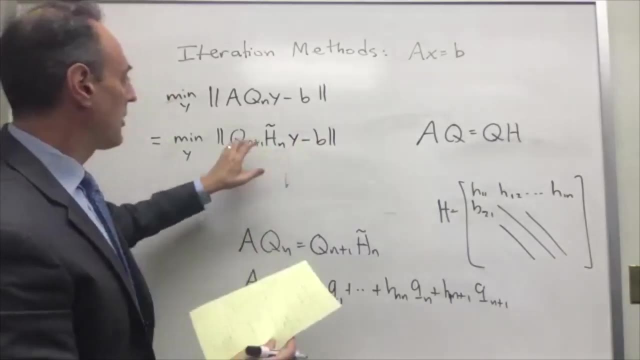 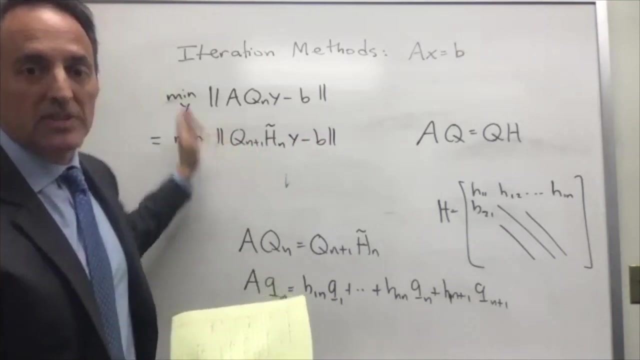 now this hessenberg, nth hessenberg form: y minus b. now turns out y and b are both in the column space of q n plus one, and so what i could do for both sides is multiply by q n plus one star. in other words, because this is a unitary transformation. 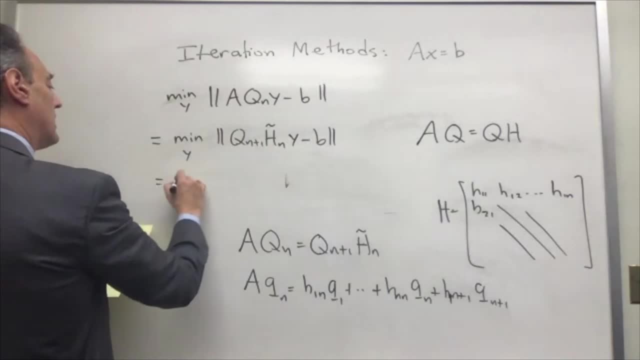 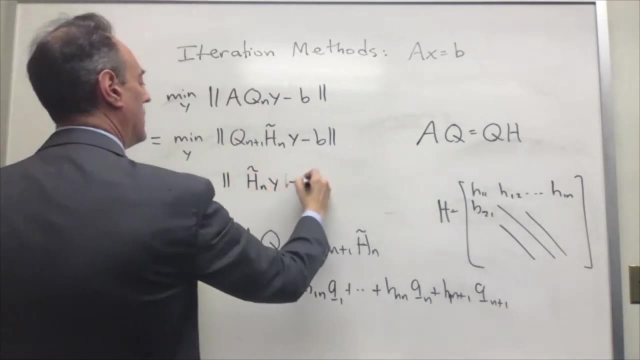 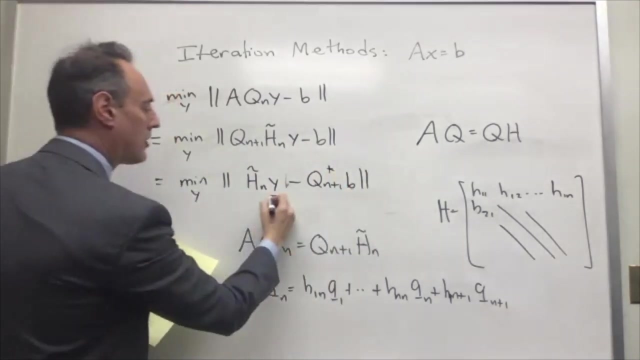 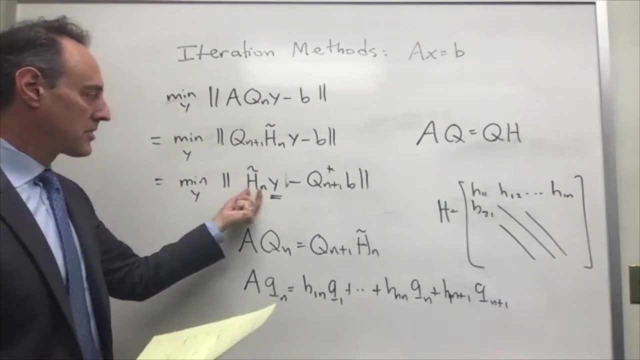 i can simply take the inverse of it to basically get the following. okay, and remember what i'm trying to solve for is this here, this y, so i want to minimize the y's. i have this matrix now i can compute everything, and this is an upper hessenberg form, so it already is in the spot. 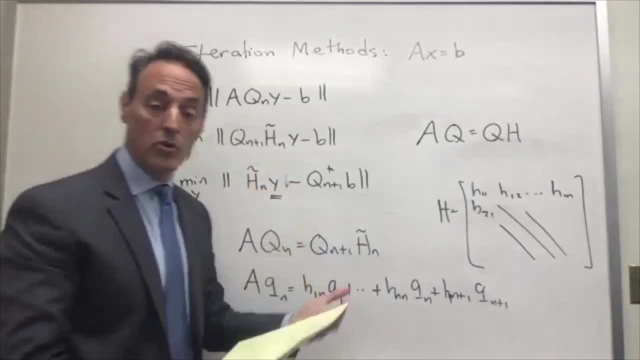 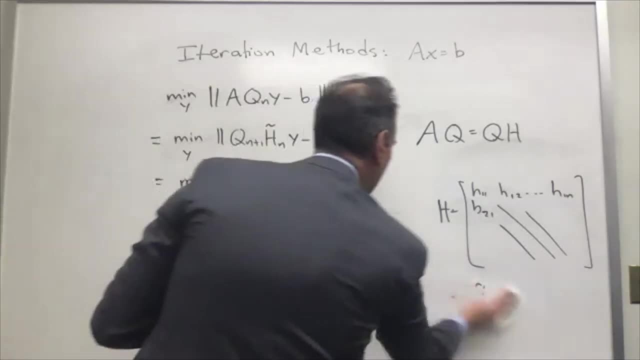 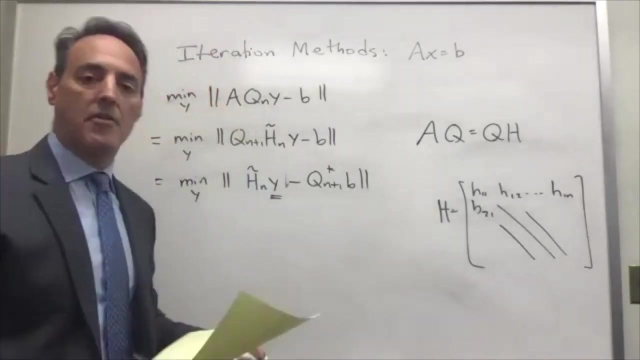 and it's in a situation where it sets me up very nicely for doing, in fact, a least square fit. so there's a lot of steps i'm skipping here because i just want to get to the punch line and uh, and so that you at least have the main idea. but this is, this is the idea, remember that. 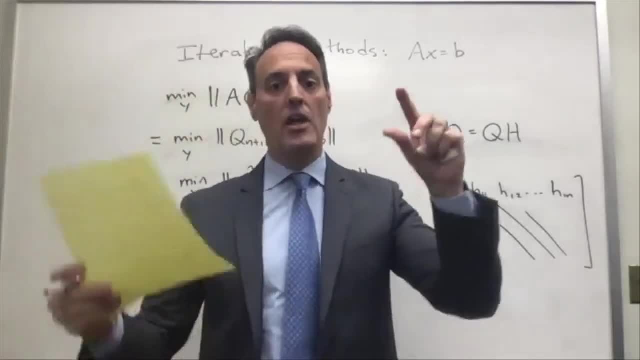 iteration techniques- and i said this previously, but i'm not going to do that, because i'm not going to do that, because i'm not going to do that, but i'm going to do that, because i'm not going to do that- with eigenvalues. iteration first: make a transformation into some favorable 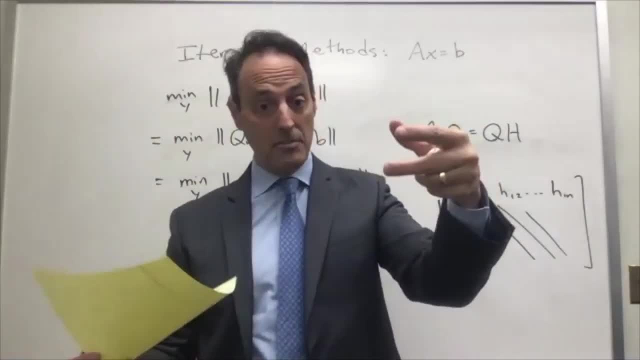 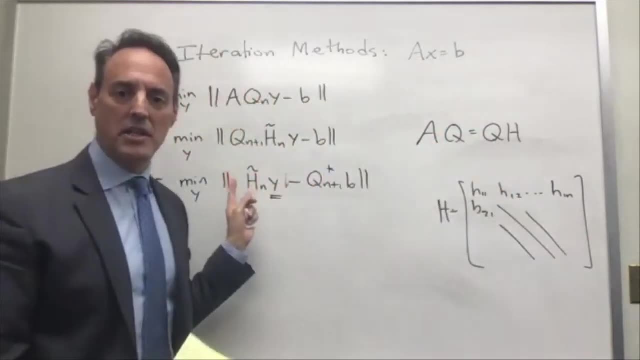 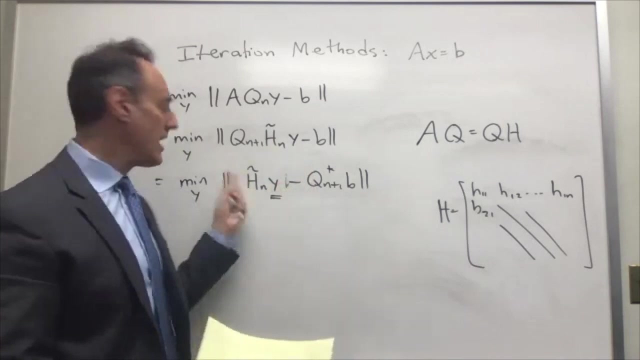 variable, setup like hessenberg form and then do iteration. we were talking about that in the context of eigenvalues and eigenvectors, but notice, i just did it here in the context of solving x equal to b. use that hessenberg form and now i've set myself up to do the iteration. 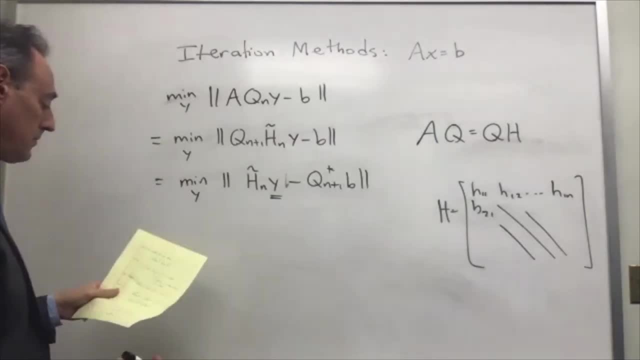 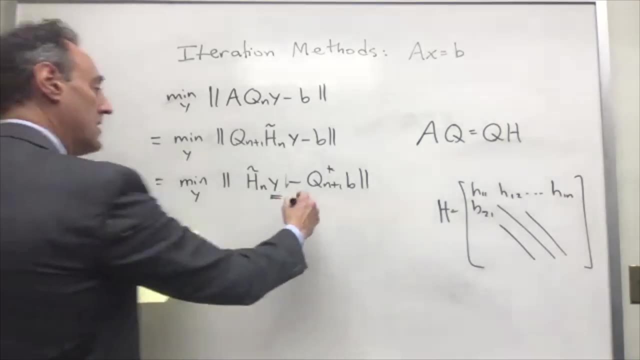 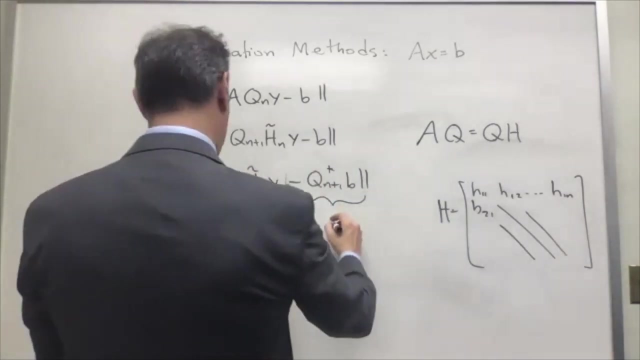 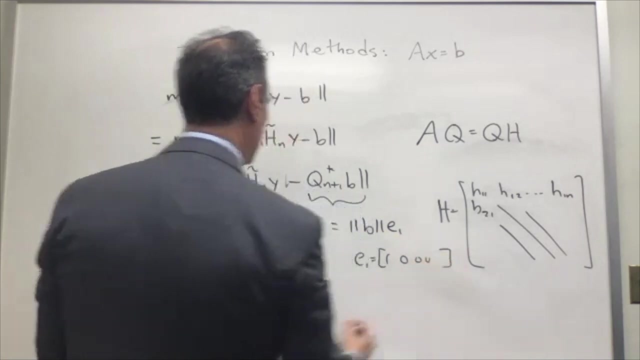 from here. okay, all right. um, the only other thing i want to point out here is that this guy here- because now it's in the nth plus first direction- this is equal to the magnitude of b times e1 vector, which is one zero, zero, zero. so this thing here just results in- and i know i'm skipping a lot. 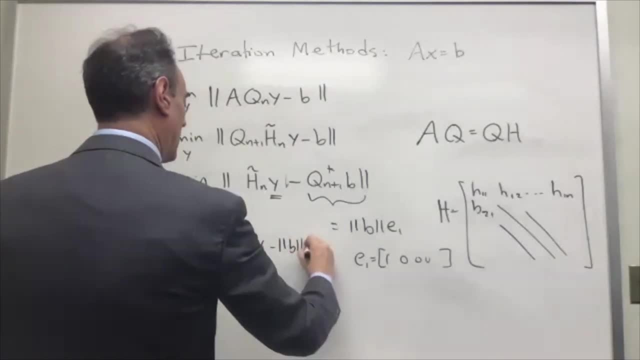 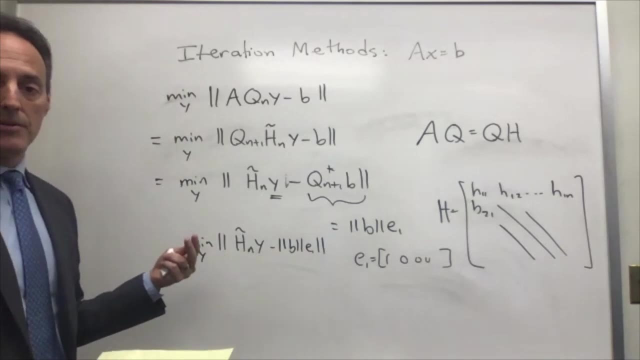 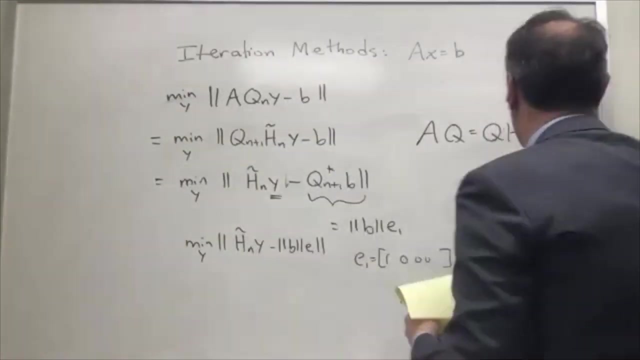 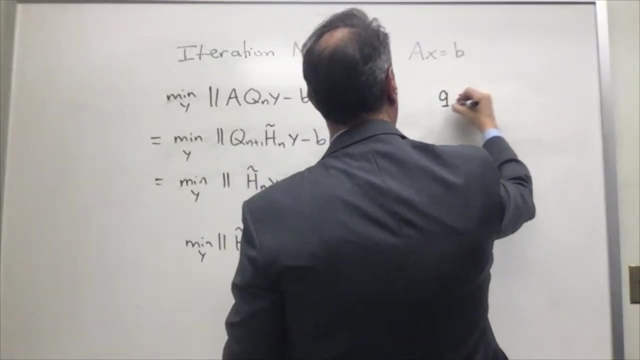 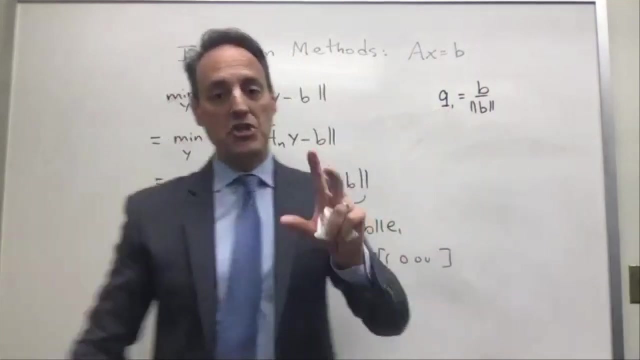 of algebra, but that's just the way it's going to go for today. but minimize that respect to y. so this is your generalized method of residual algorithm. so let's talk about how we do it in practice. as an algorithm, your first direction is the b. this is just like graham-schmidt. remember that my 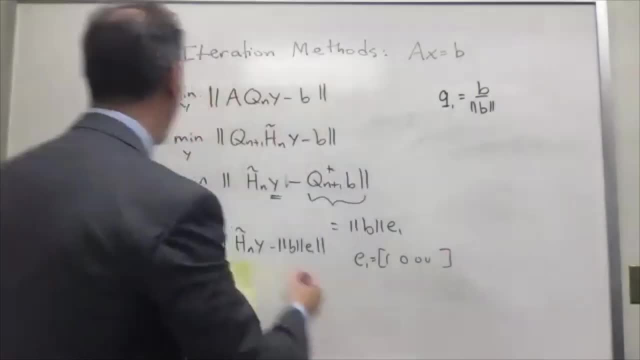 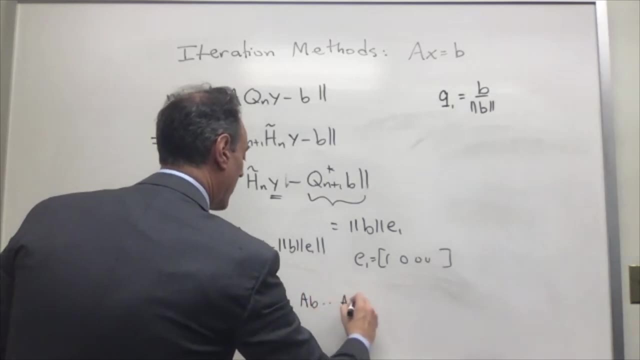 i'm working with the nth plus first direction and i'm going to do the iteration with this krylov subspace. remember what the krylov subspace was. krylov subspace, krylov vector for b, a, b, so forth, all the way to a of m minus 1 b. 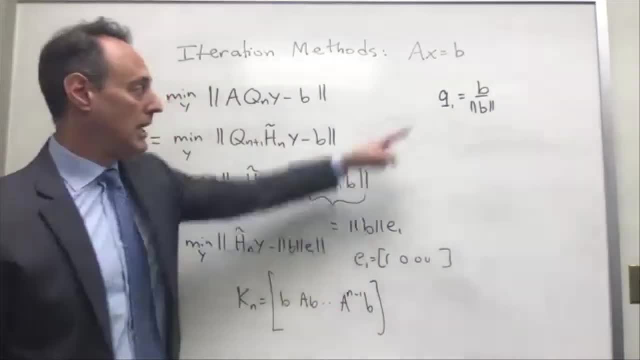 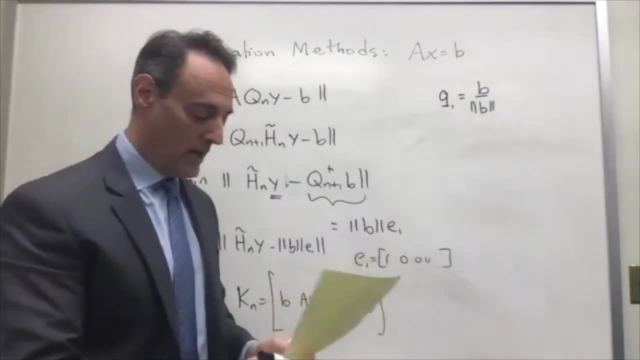 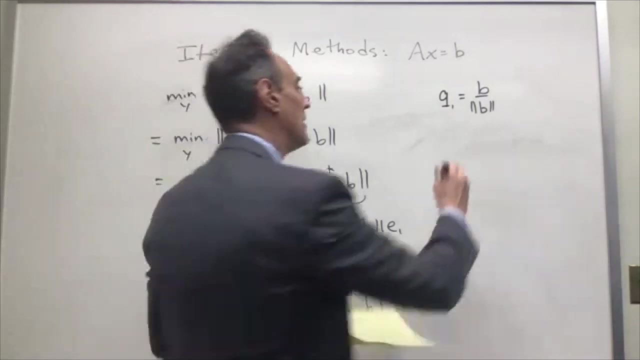 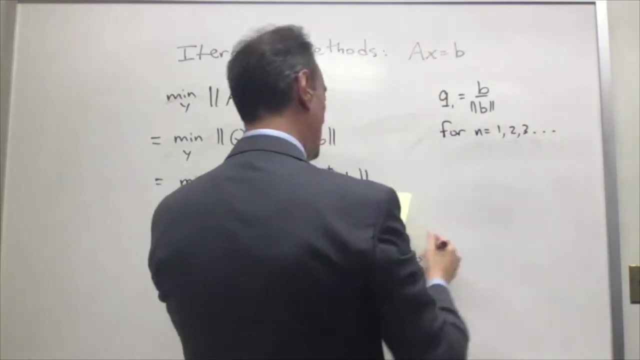 how did we do qr on this? we picked the first direction and normalized it, that's q1. okay, now what do i do? well, what i got to do is now go get all the other vectors and start this process and time. so four n equals one, two, three, so forth. first i do arnoldi. 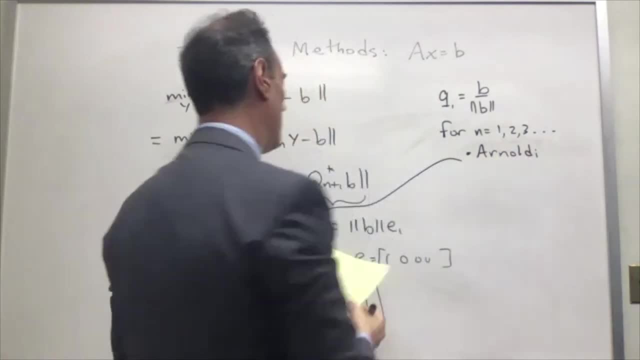 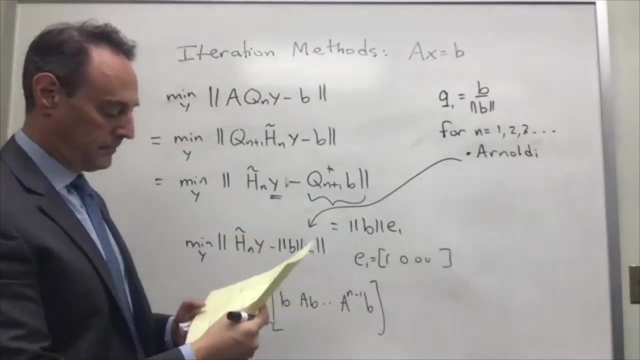 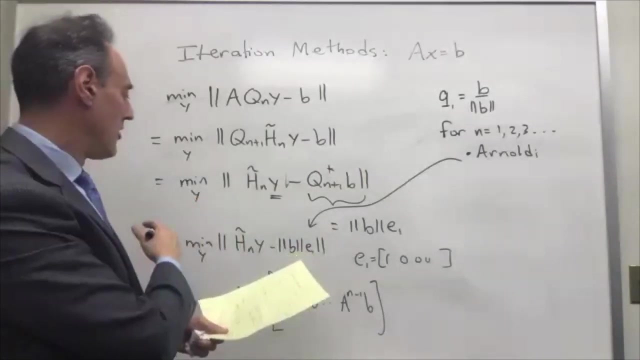 which is this guy right here. okay, and the step of the arnoldi. solve this, okay. sorry, the arnoldi is what i erased. it was the uh, the arnoldi is what's going to give you. uh, sorry, i erased it. it was that recursion formula. 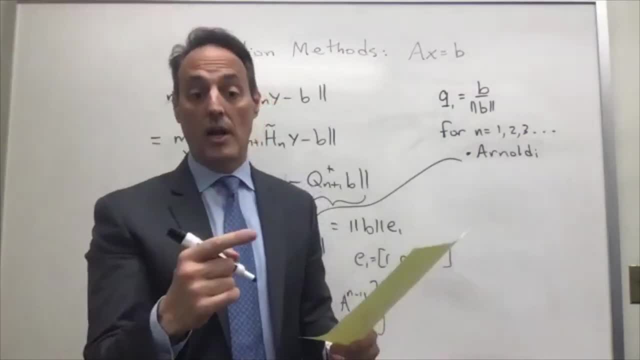 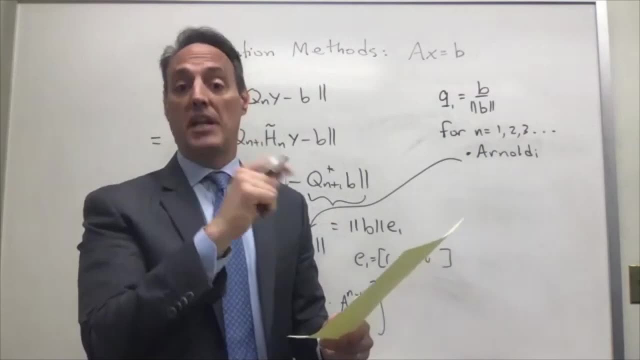 and once you have that recursion formula for getting the q of n plus one right- so that's the thing you want to get- is you get your next q from that recursion relationship that i showed you, which was the arnoldi formula right of a acting on q event, which was related. 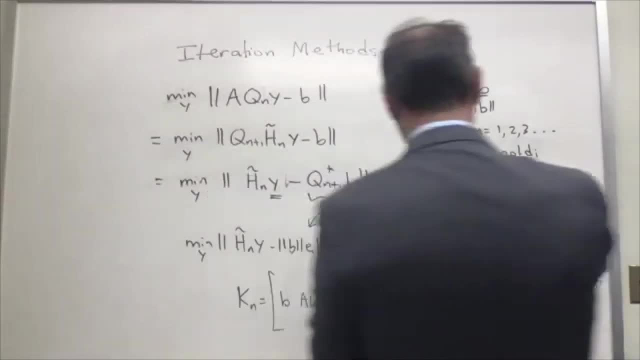 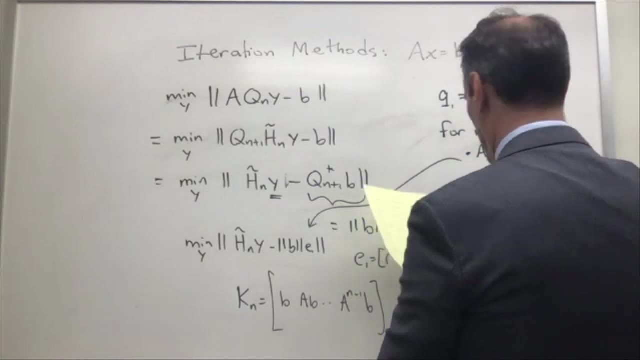 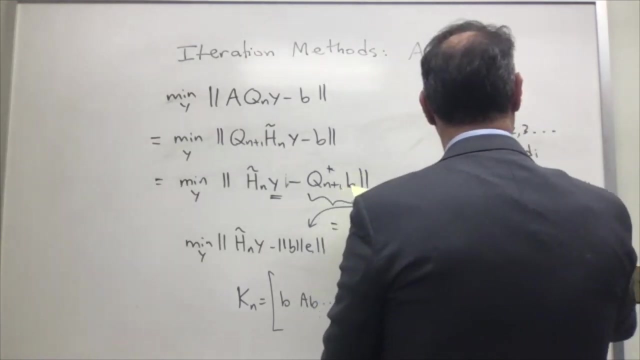 to the q of m plus one. then, once you have that, then you do this method, and then you do this, This minimization over Y, H, Y minus B, B1.. And then your X of N is equal to Q of N Y. 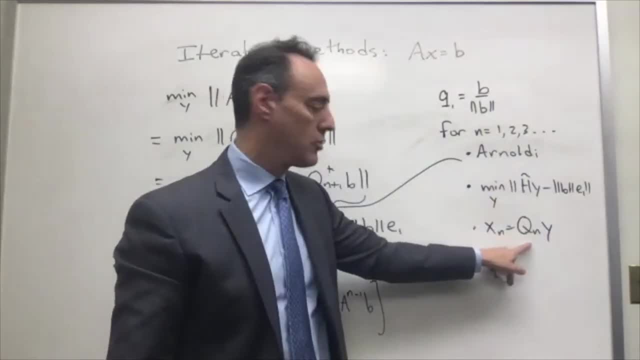 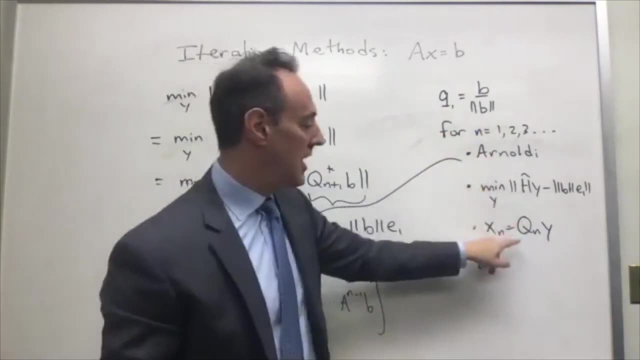 So you solve that Y. your next X of N is just project onto those orthogonal directions. Repeat, that's it. So when you come back up here you connect it to the next direction, Q of N plus one. Now you can solve this. 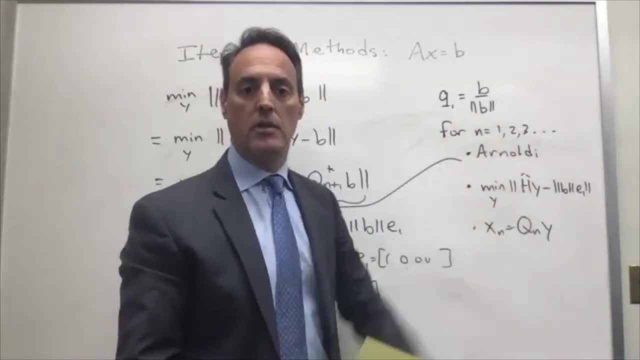 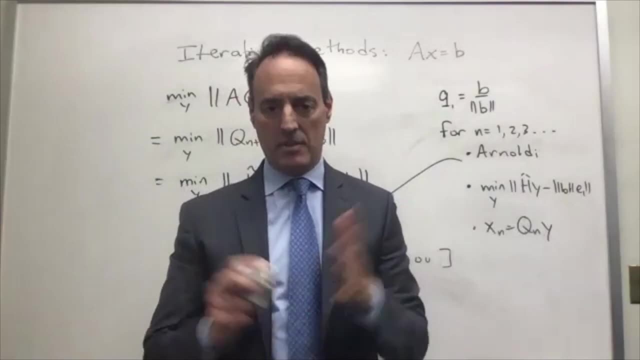 Now I'll go here Q of N plus two and you just recurse. So that's generalized method of residuals. So you see it's kind of fancy, but it's. I mean, if you kind of spend a lot some time with this. 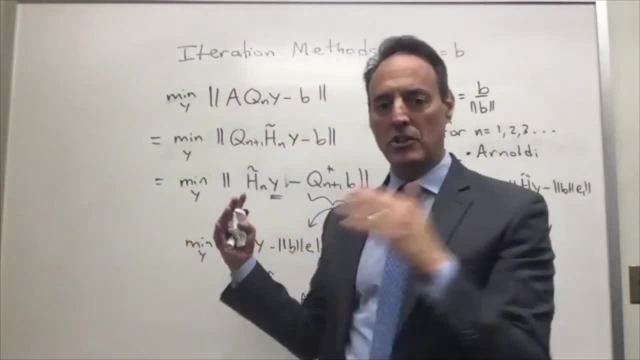 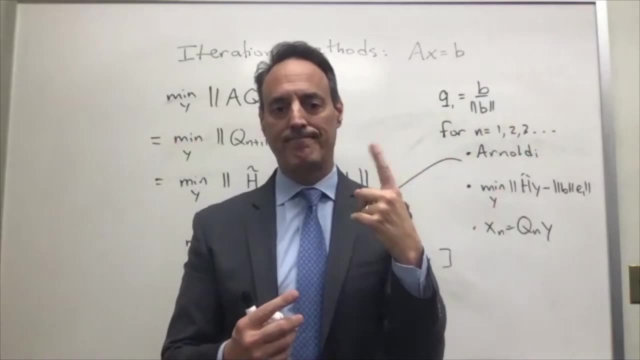 this. I you know this building up to this GM lecture, GM res lecture. there's like three or four lectures in trofethin and I compressed it down to one. Sorry about that, But all the details are there.